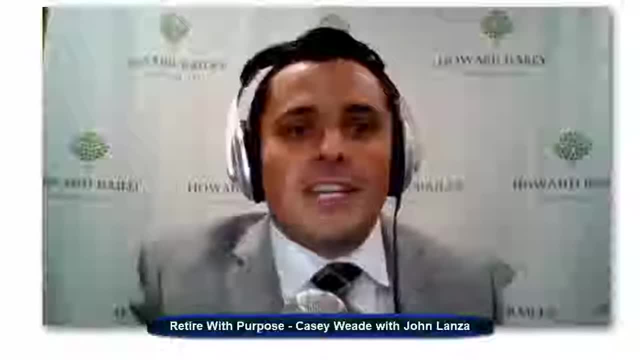 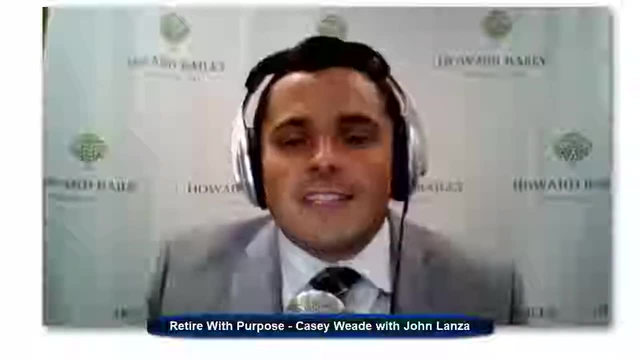 guide to raising money-smart, money-empowered kids. John and his program have been featured everywhere. John has been featured in The New York Times, The Wall Street Journal, He's been featured in the LA Times and he's here now finally with us on Retire With Purpose. 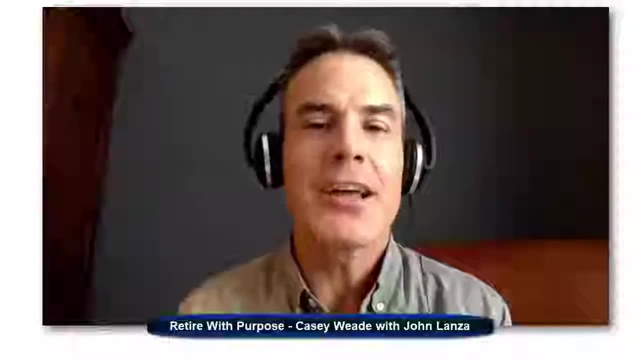 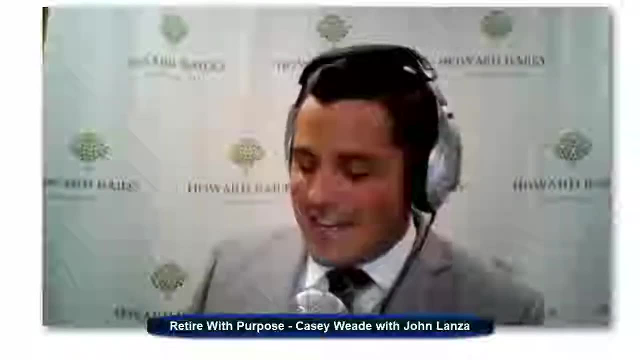 John, welcome to the show. Hey, thanks, Casey. I'm glad to be here. I like to see that your Art of Allowance is fully tabbed out. Yeah, well, absolutely. I got through the Art of Allowance and there was so much, Really. 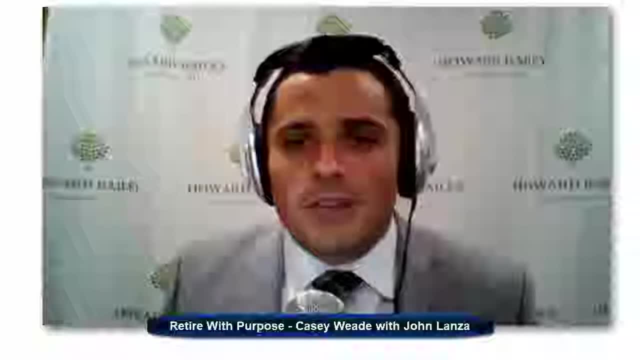 it's largely common sense. We're one of Dave Ramsey's smart investor pros and the reason we were put on his program was because of our common sense approach. Yeah, I just feel like we've lost touch with over the last couple of decades. Maybe the 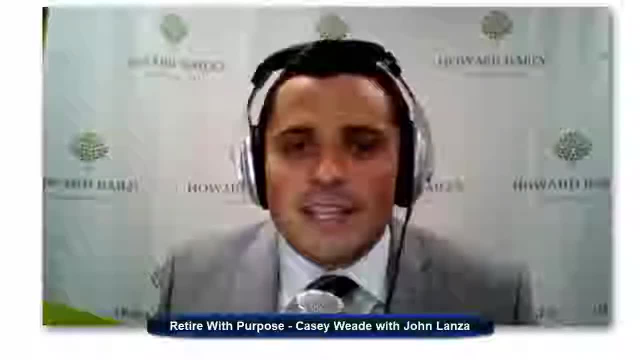 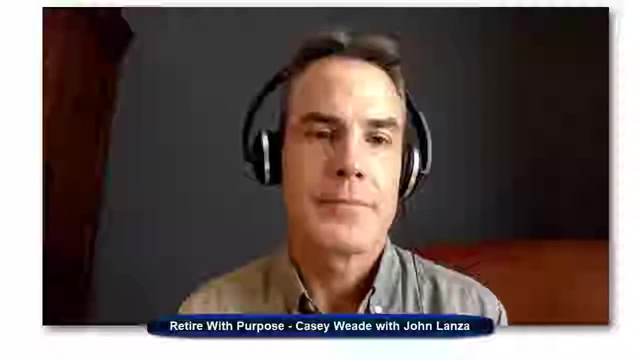 last 30 years, even, I think, in the investment world, it's completely changed, where we've lost a lot of common sense. People want the silver bowl, They want the perfect investment, and we just need to get back to the roots that our grandparents had through the Great 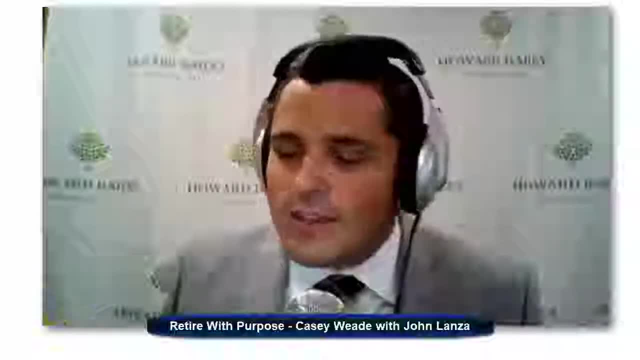 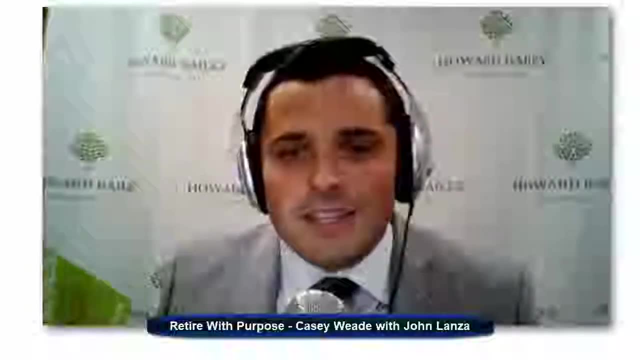 Depression that I learned a lot of lessons from. Yeah, I think what you had here was largely common sense to the Art of Allowance. It's just something that I've learned from many of my friends, So I do appreciate that. I appreciate it. 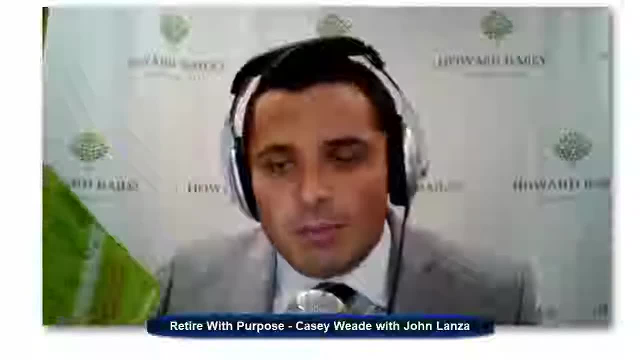 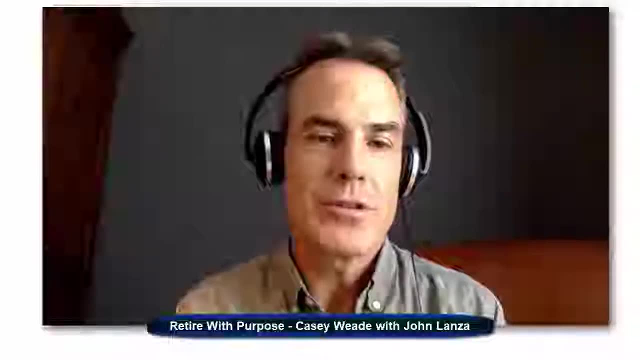 that I think so many people just don't think about. We just need to be brought back to that every once in a while. Yeah, and you know that as a CFP, I talk to someone like you who really, really knows finance. 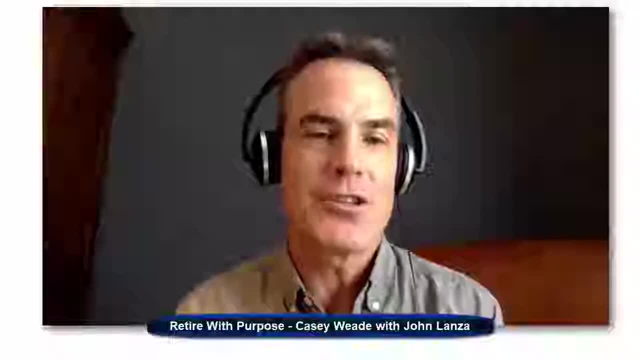 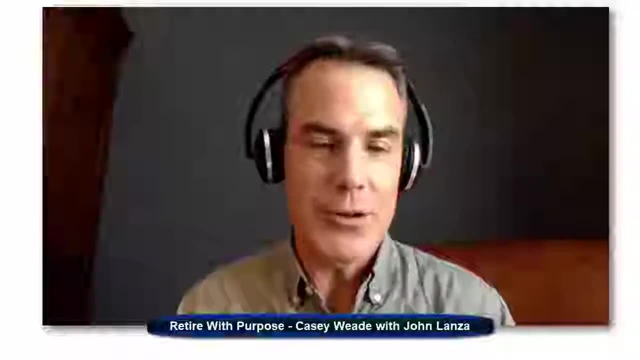 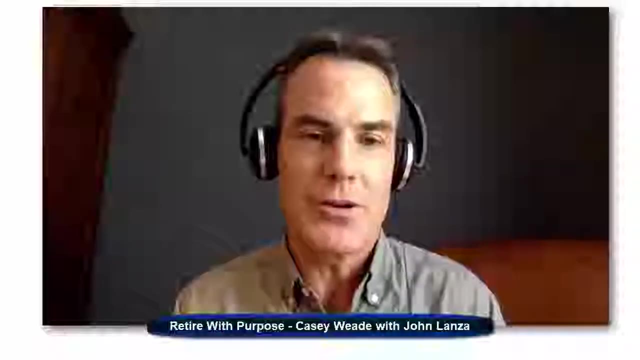 and so you know the details And I think it's the details that really get to people. because if you just kind of pare things back to the basics, like in the book, we talk about just like the basic: money, smart principles, saving for goals, making money, smart choices. 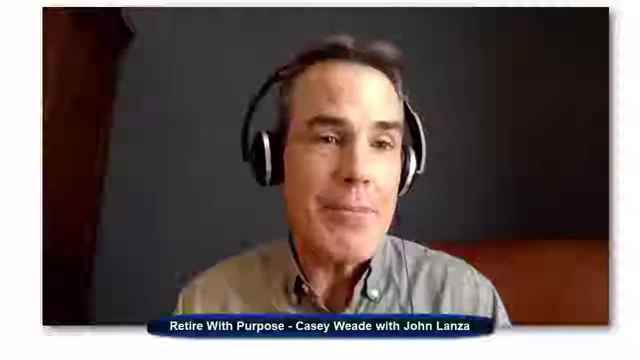 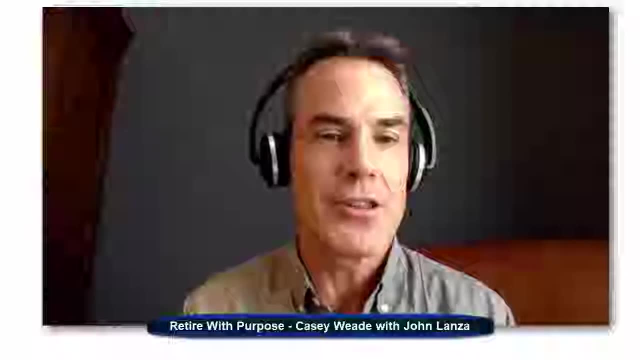 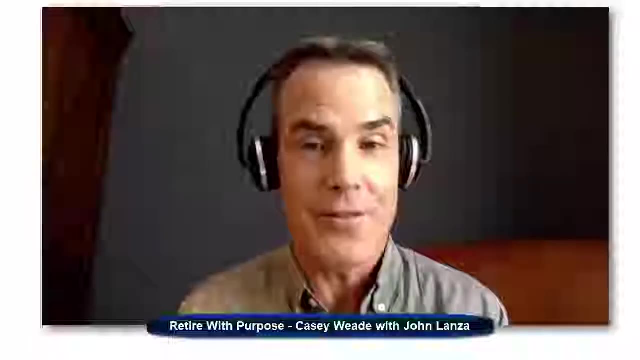 and distinguishing needs and wants. that makes it a lot easier for a parent to kind of take this on, because it's not as intimidating When you start thinking about the rule of 72, compound interest and complex financial instruments- and I'm not a finance expert- 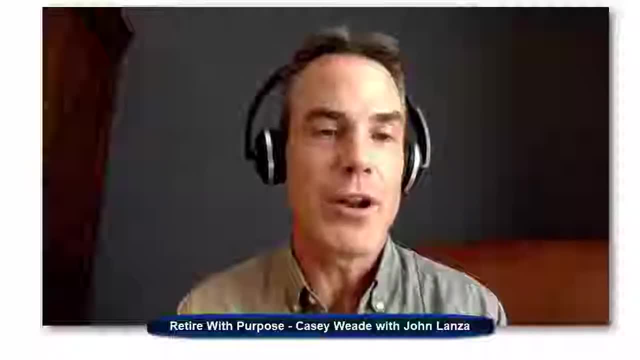 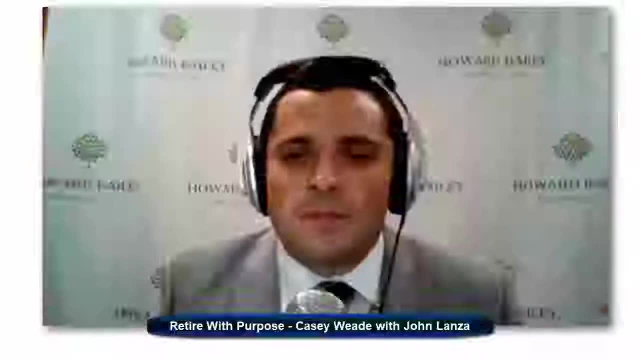 so that stuff scares me sometimes. So that's what I want to do and I think you hit it dead on which is it? It is very much common sense and that's what I want to kind of impart to parents out there. 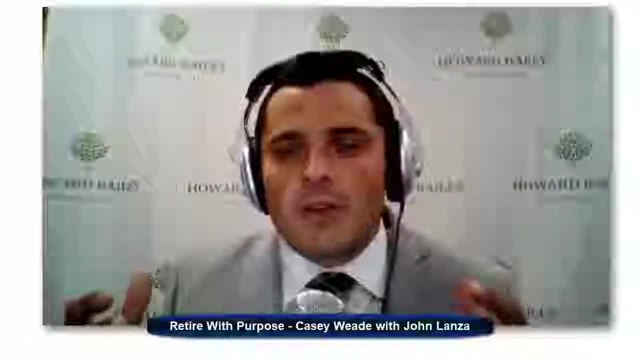 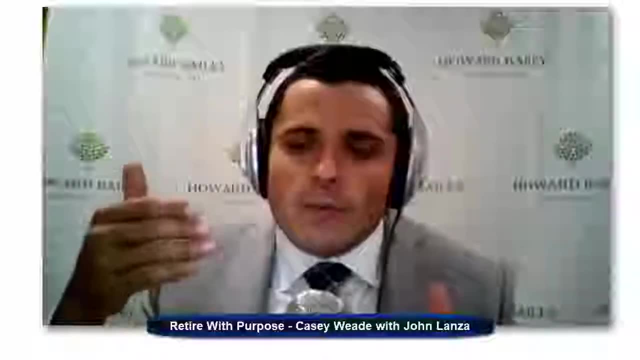 Well, you've provided a framework, I think, for people to work from, and that's what the purpose-based retirement was all about was we don't need to – we need to kind of work ourselves backwards and work ourselves into the finer details, and that is okay. 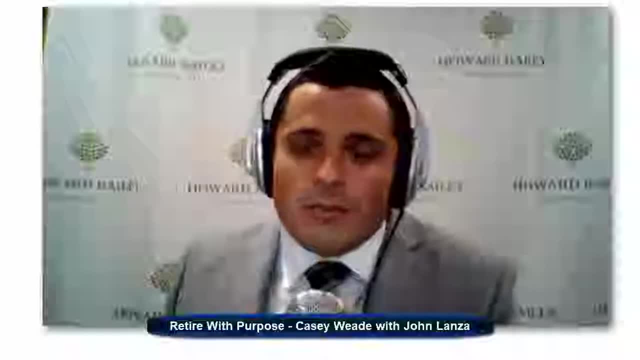 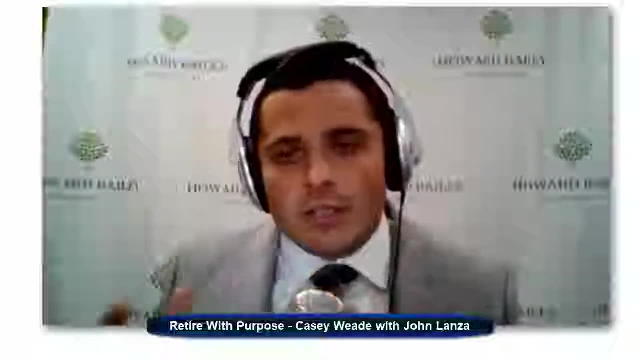 you've got emergency money. You've got income money. You've got growth money for inflation. You've got your estate plan to take care of health care and taxes and estate documents. We just need to determine how much goes in each bucket and then we finally work into those finer details of the vehicles. 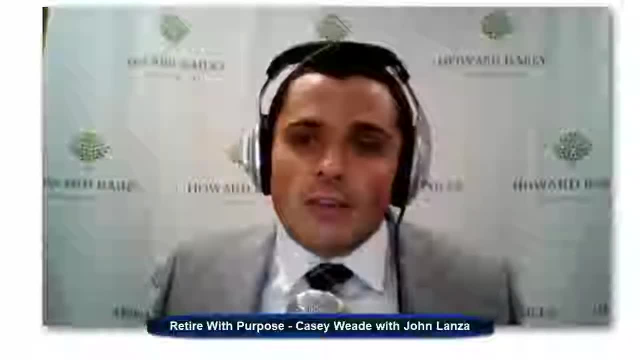 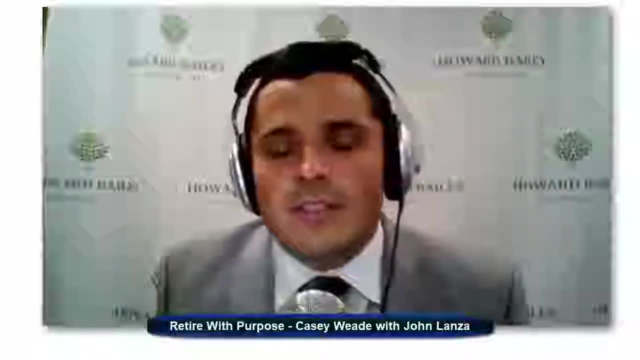 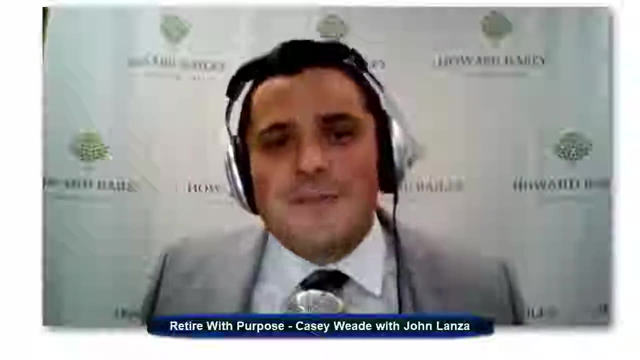 that are most efficiently going to get us to the end goal, and I think that's really what spend smart and save and share has really done for even kids. So before I just start telling everybody about what you have going on here, I'd like to hear it from you, and I'd like to start with some questions. 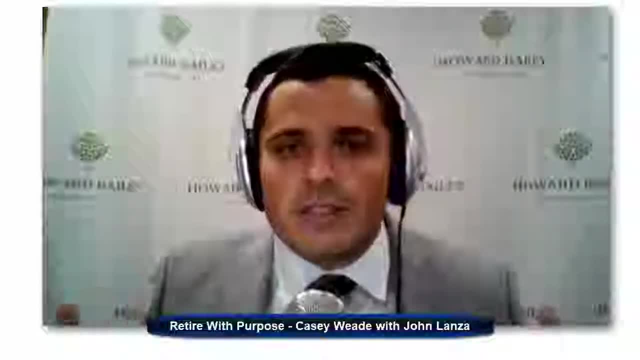 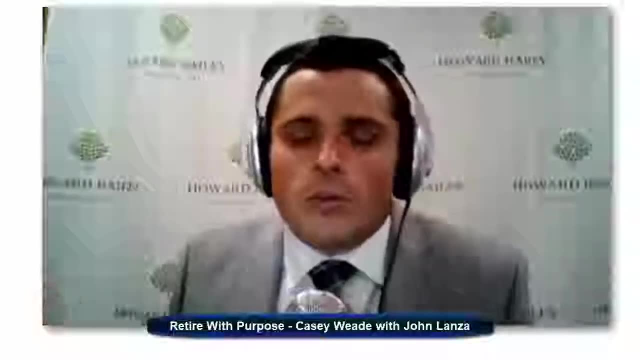 from our fans. We get some questions prior to our interviews that we'd like to get out and make sure get answered, and I think some of them are very common sense. that will get us to, ultimately, I think, your goal, which is spreading the word of allowance and Money, Smart Kids. 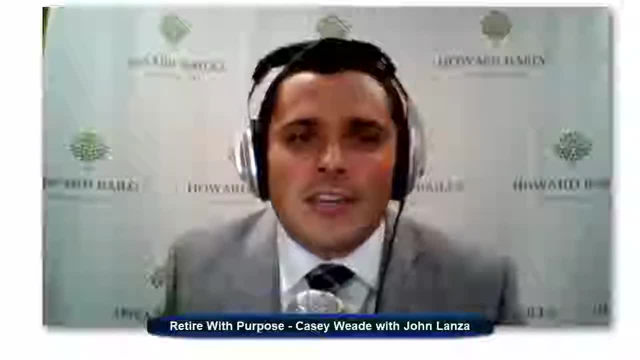 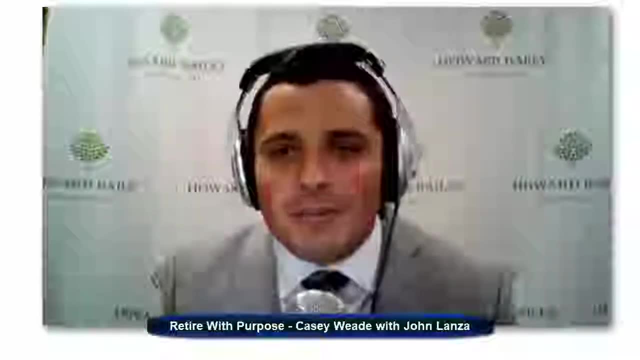 and our first question comes from Deb Johnson and Jeff and Deb Magsom. I kind of combined these two questions into one because they're really one and the same. I wanted to give them both credit for the question and they said: is it a good idea? 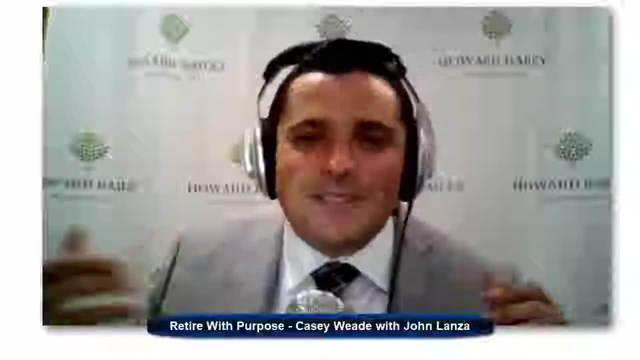 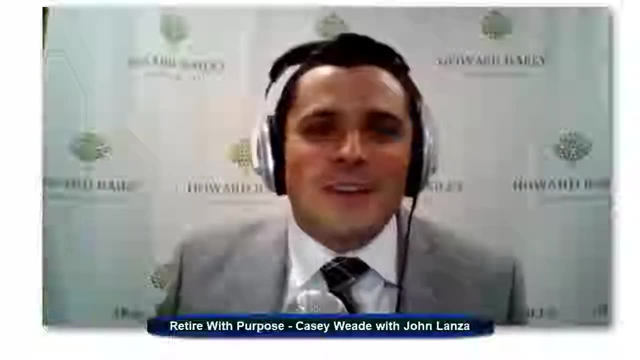 Is it a good idea to give your children an allowance? And that was such a great opening question. so why don't we? obviously you believe in allowances, so why don't you just share with us why you believe an allowance is such a good idea? 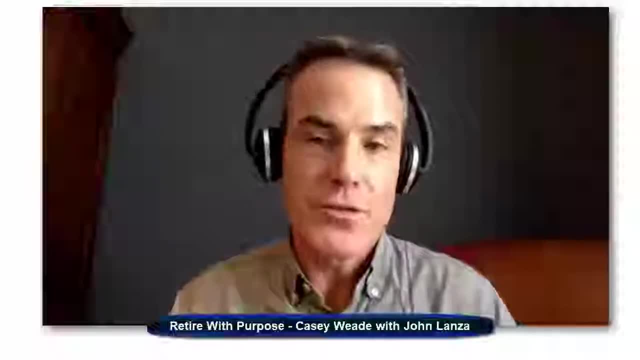 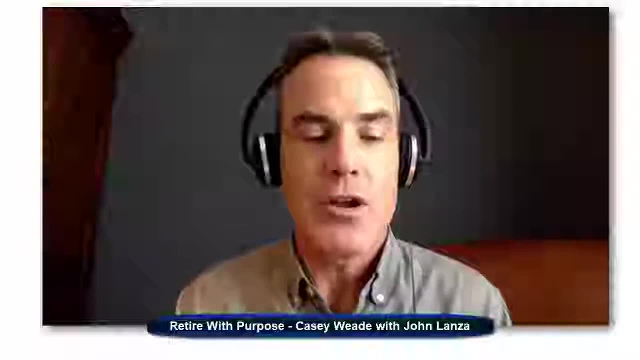 Yeah, The reason is that an allowance, first of all talking about purpose-based- you have to have an allowance that has a purpose behind it, and I think the reason that people sometimes ask that question is that they don't really know what it is that they're going to get out of it. 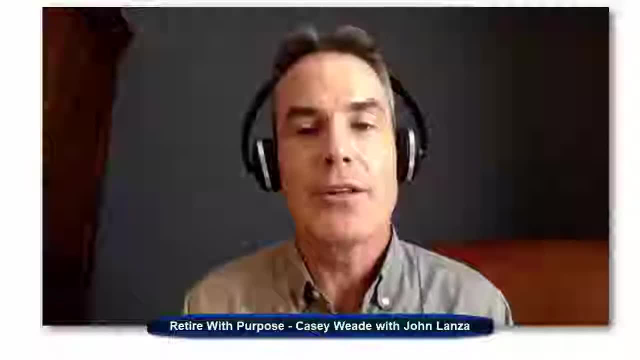 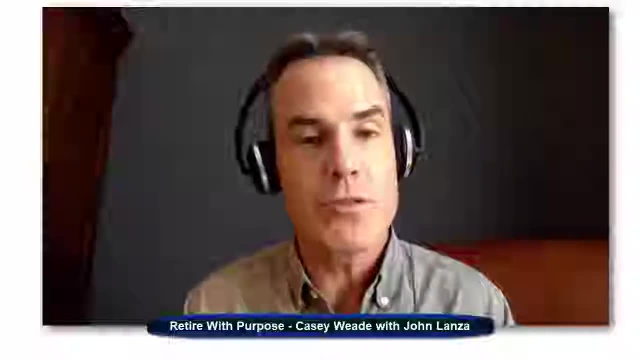 They don't really know what it is that they're going to get out of it. They don't really know what purpose to put behind an allowance. So an allowance is designed to teach your kids money smarts, and that is to get them comfortable with using money and to eventually become 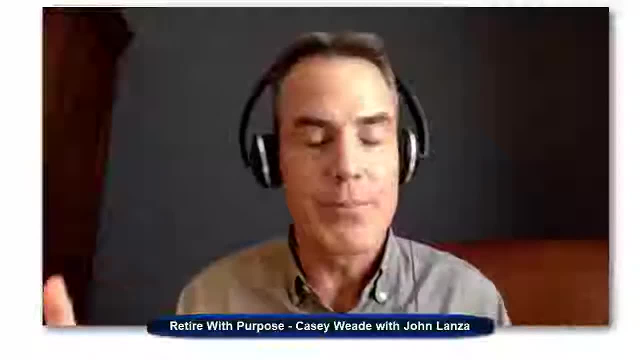 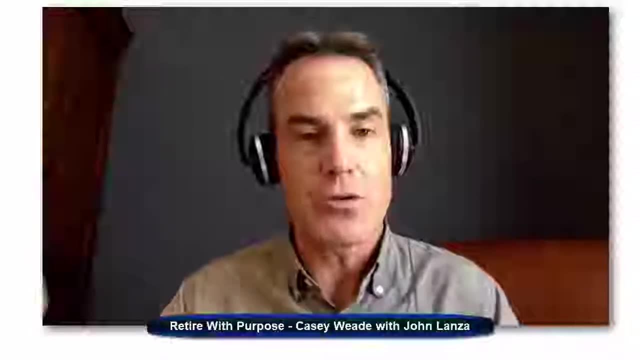 kind of money empowered, and what I mean by money empowered very simply is just that they learn to have control over money, versus the other way around, where money is kind of having control over them. That's the long-term goal, That's not your short-term goal. So the allowance is doing just that. You set up an allowance that kids get money to practice with, because there's no way they can learn to become financially smart or money smart without actual money, and you dole it out on a weekly basis in the beginning. 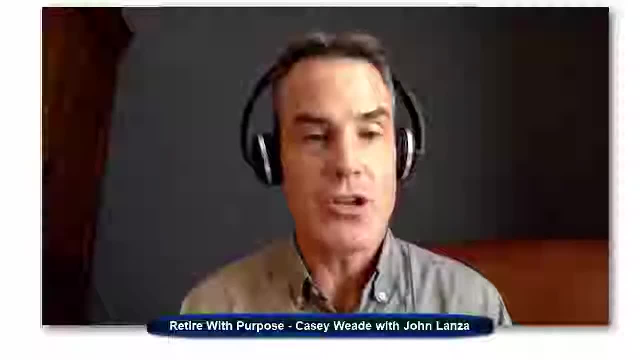 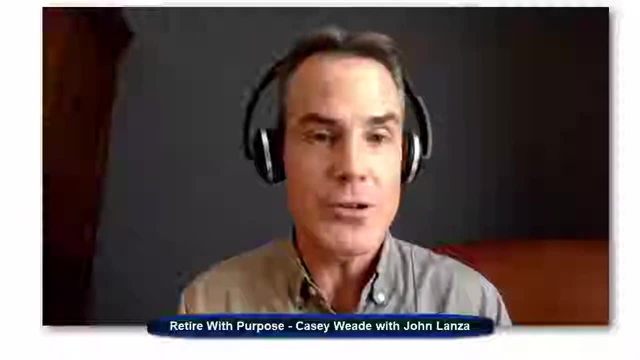 and you get them used to making money, smart choices, and used to understanding those differences between needs and wants and starting to save for goals. So that's the purpose of setting up an allowance for your kids. Well, I think a lot of –, I think there's –. 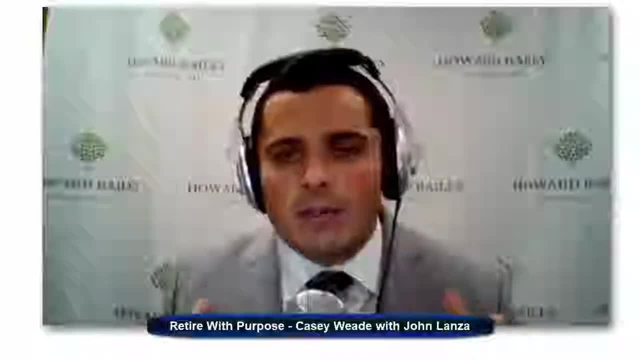 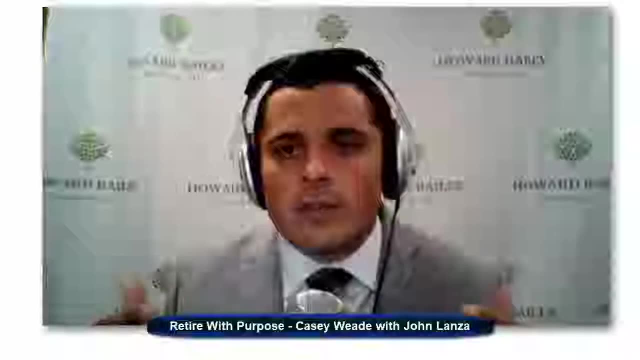 in some ways there might be a bit of a taboo for some regarding allowance because they – I think especially our audience largely being in this generation of baby boomers, they're afraid to deliver any more feelings of entitlement to the millennial generation that they already feel is there. 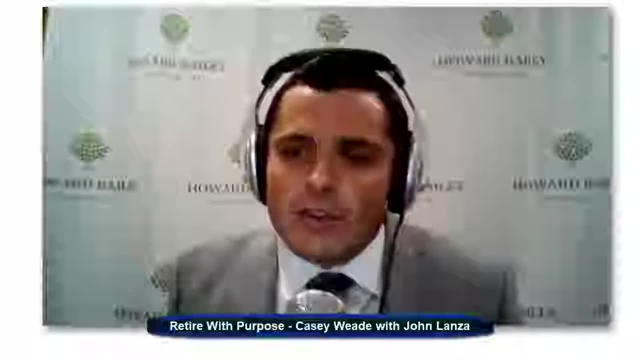 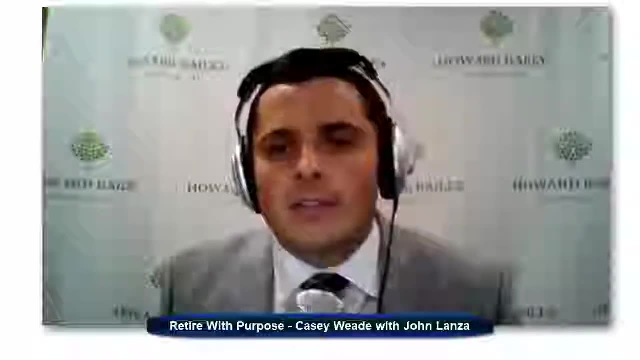 So if we just start giving them money and they're not doing anything, they're not doing chores, then aren't we just entitling them to? well, I deserve to get that $20.. Yeah, it's a very good question. 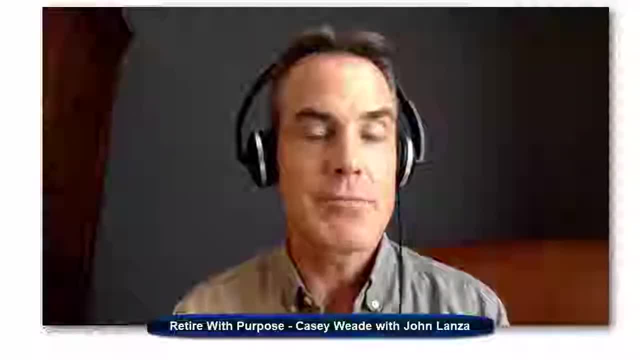 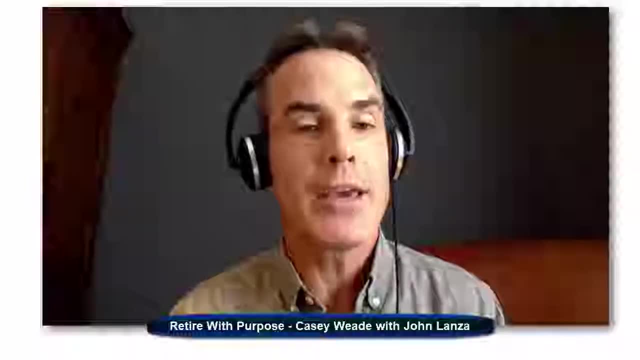 And the term allowance is a loaded term because people do sometimes think it's an allowance. It is just a giveaway, And it is a giveaway if there is no why behind it. So the why behind it is that you are teaching your kids about money. 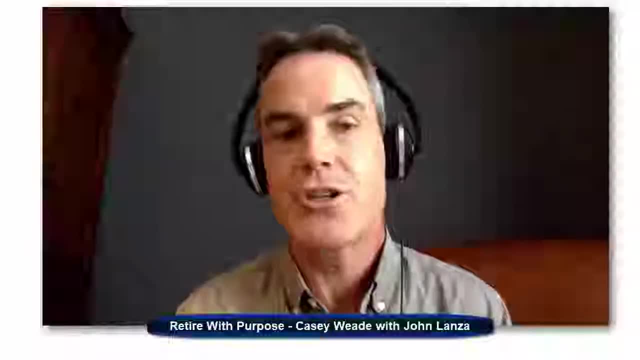 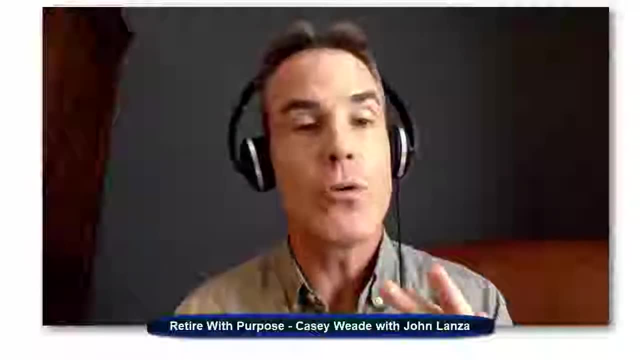 You don't have to tie it to chores, because chores teach a different lesson. The lesson behind chores is that you need to work to earn money. Great lesson. You don't have to – that's not the purpose of an allowance And so –. 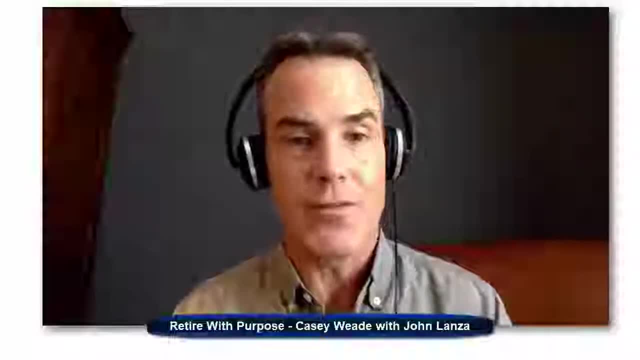 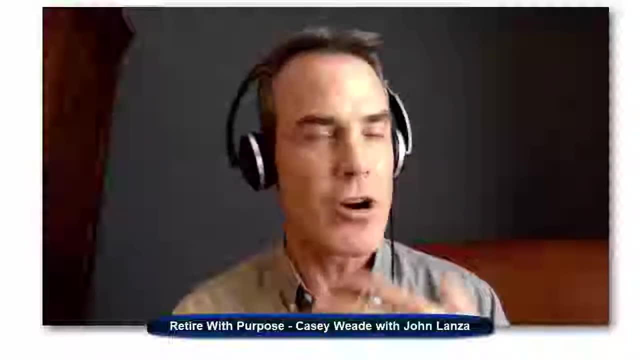 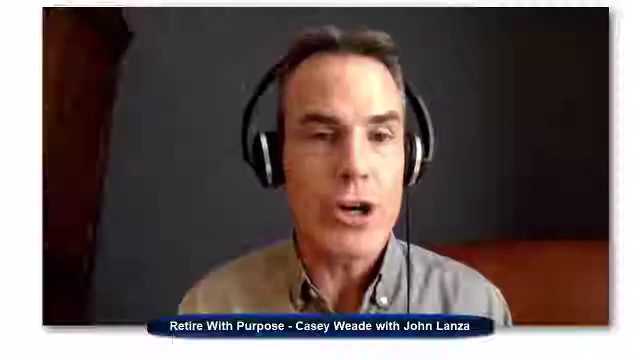 So an allowance without a purpose behind it is a giveaway right? So, for example, my parents were wonderful, but we didn't really have a consistent allowance. We started with an allowance at one point for a short period of time And they didn't really have a sense of how that should work. 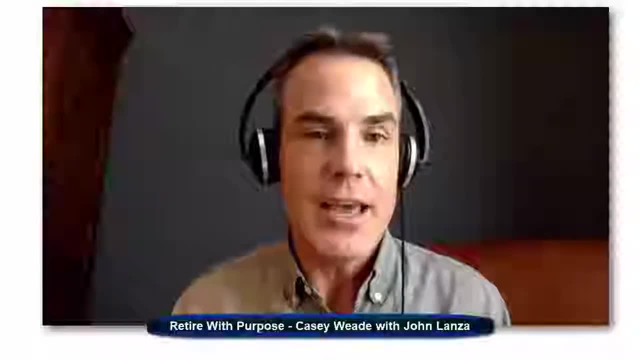 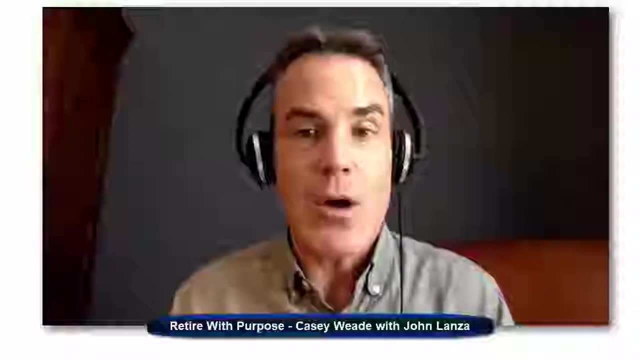 And so it kind of started and stopped and was done, And they did it out of the good of their heart. They wanted to teach me about money, but they didn't really understand how to set it up to provide. They didn't really understand how to set it up to what the framework is. 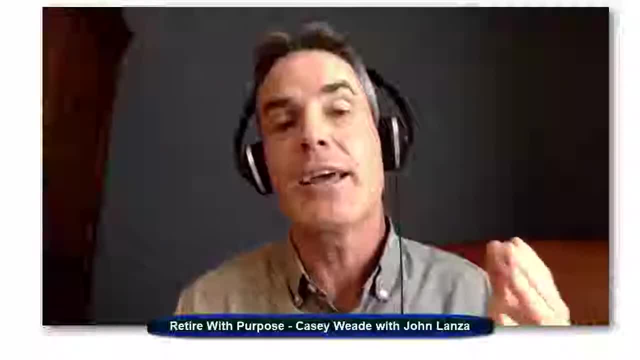 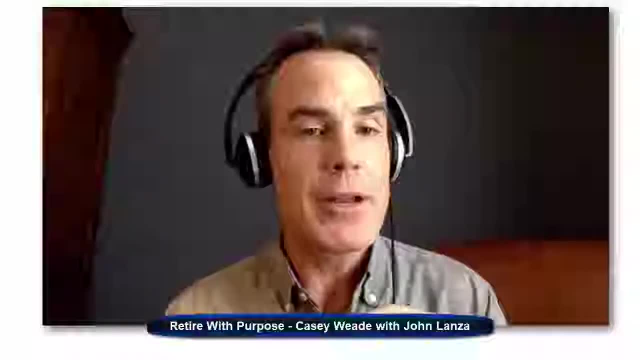 And that's kind of my purpose here is to explain to people that there is a framework, And I like that you use that word because, as you find, when you deal with families or anybody, when it comes to money, everybody is going to be different. 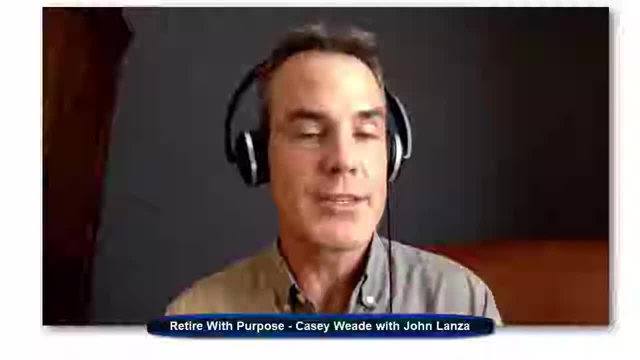 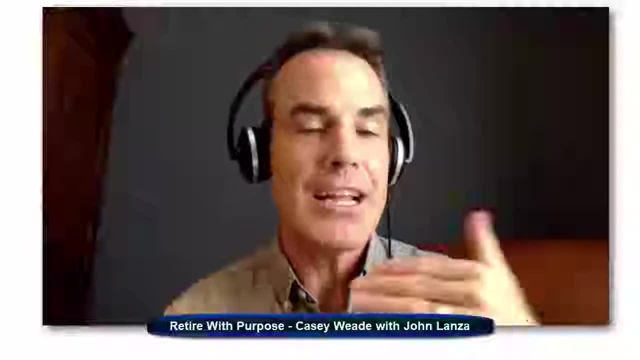 Every kid is going to be different. Every parent is going to be different. There's no one-size-fits-all plan, But there is a framework and there are basics that you can work around, And that's what we're trying to do with this allowance setup. 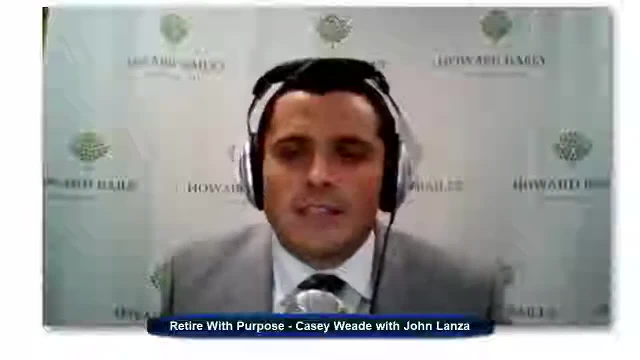 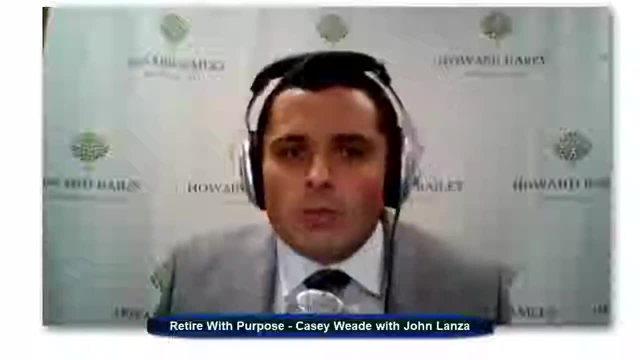 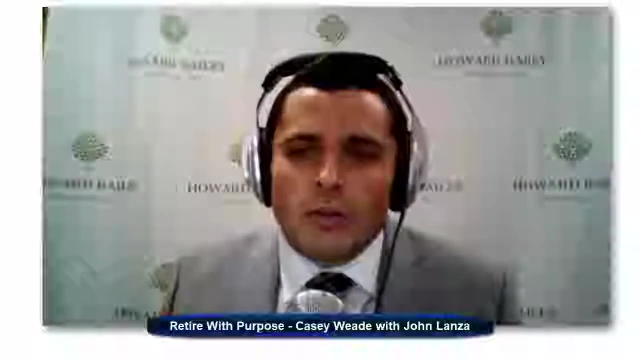 Which I think is really – The art of allowance. right, It's imperfect, Everybody is different, Everybody is unique, And it's just another word for really just providing a framework, and then you work within that. overall, What I really found interesting within your book was the discussion regarding chores and allowance. 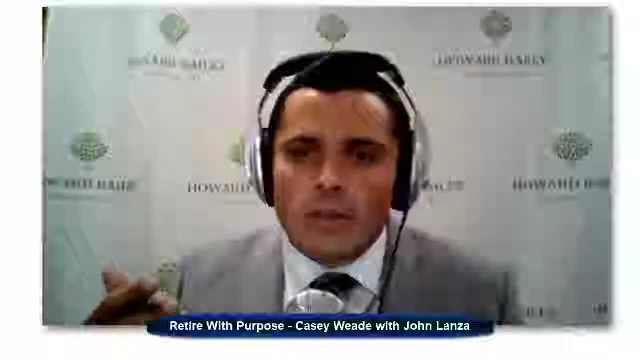 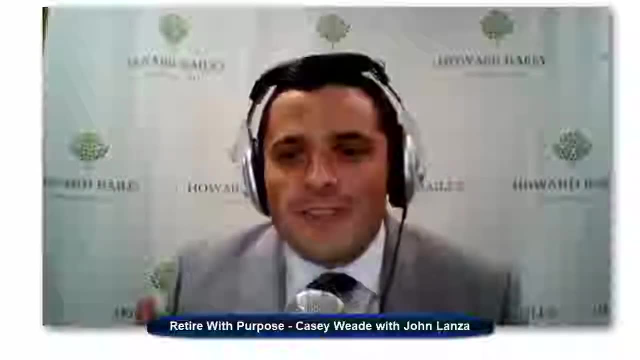 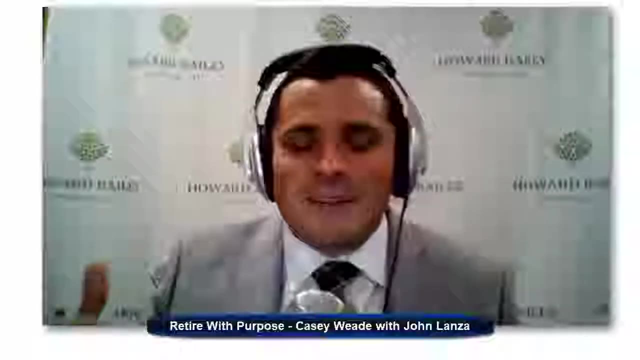 I think in a lot of families in order for the children to be compensated there have to be chores. I think we were kind of running into this issue even in my own family. I had already implemented part of the art of the allowance before I got to the chapter on money negativity and decoupling chores and allowance. 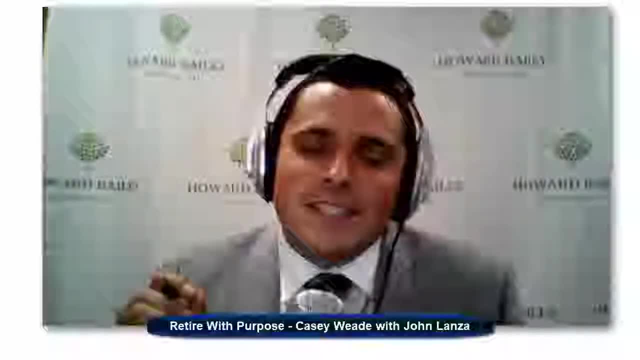 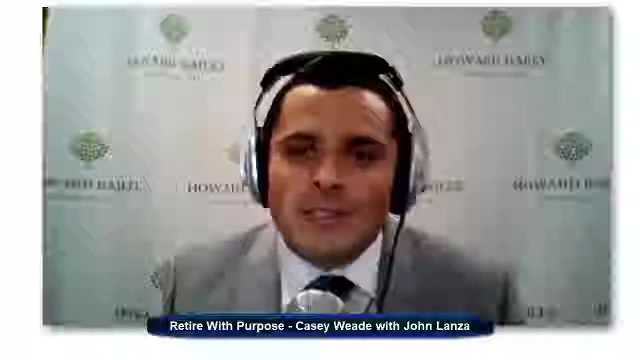 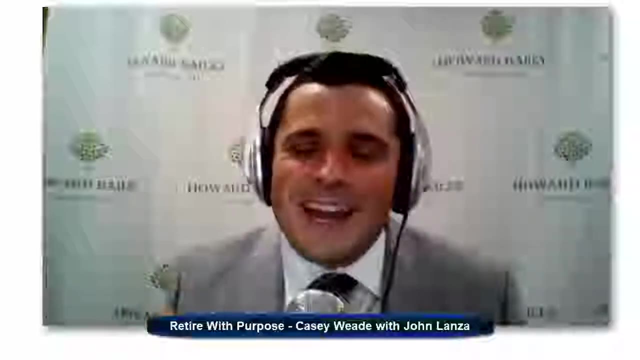 And I know my son, he wouldn't put his clothes on in the morning And I said: well, if you want to get your allowance next week, you'll put on your clothes. And then I read your piece on money negativity and I thought, wow. 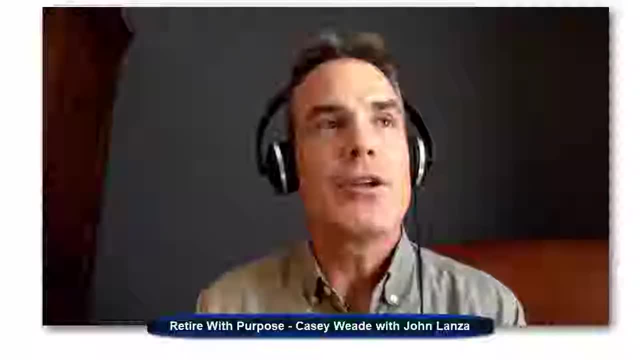 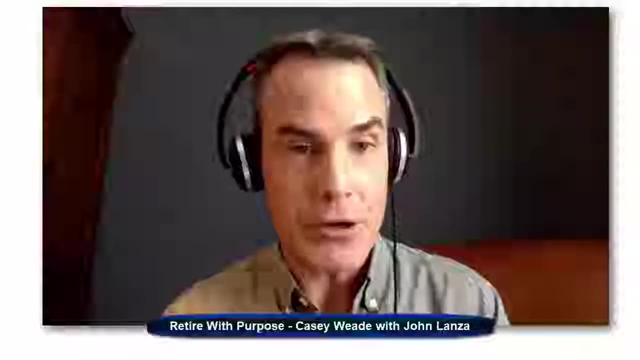 Can you speak to that a little bit? Yeah, So the primary reason that you don't tie chores to allowance – and we're talking about basic chores, So we're talking about, for example, putting your clothes on. If you call that – we'll call that a chore, because for a three-year-old that can be a chore. For our kids. it's emptying the dishwasher. My kids are now 15 and 12. So it's emptying the dishwasher, It is setting the table, It's cleaning the rooms. those kind of things. We are never going to pay them for those tasks. That's what they do as a part of the family, And so if you set it up where you're paying them in the beginning and then they get to the point where they're 15 and they don't necessarily need to get paid for it, then you're setting up a false choice, because they can't opt out of doing those chores. 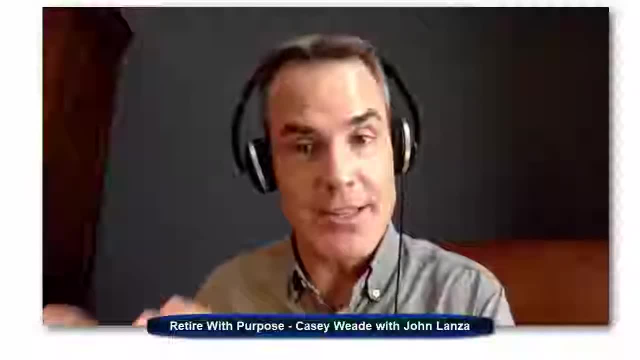 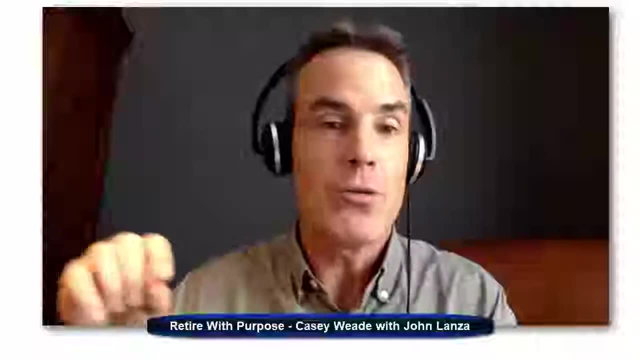 So for parents who want to teach that separate lesson, the chores they can do it for above and beyond chores, So things that they might be paying someone else for, whether it's washing the car or it might be some kind of yard work, then you can pay your kids for that. 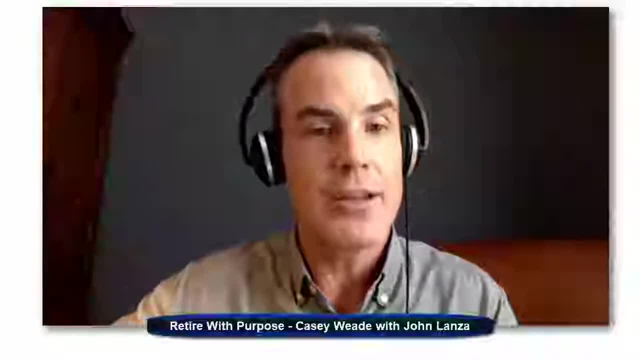 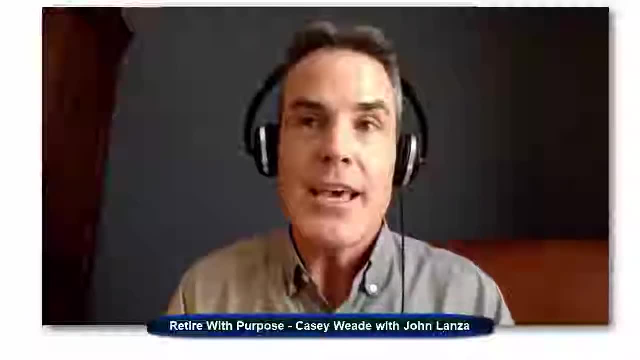 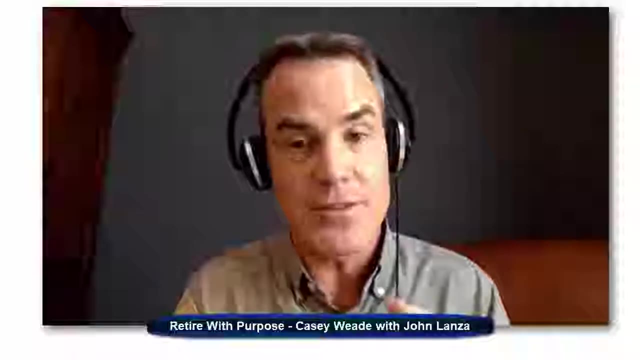 And then they learn that lesson. They learn that lesson that work can yield money. But getting back to the allowance setup and the tie between chores and allowance, so that's kind of the framework. But, like you said, one of the real side benefits of doing this, of decoupling the two, is that there's so much money negativity in society as it is. 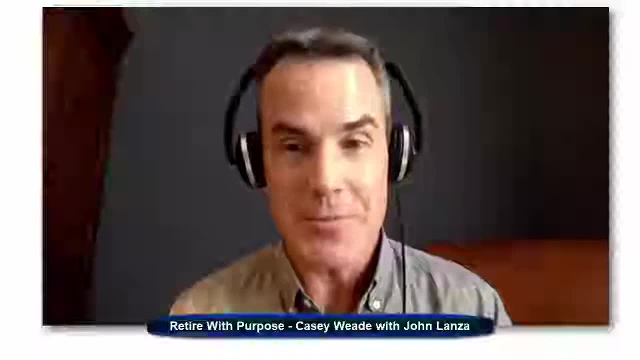 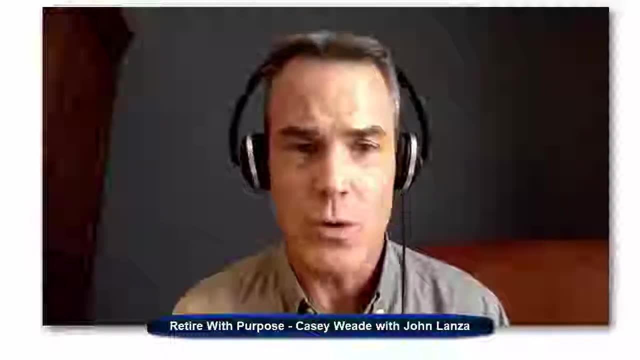 And I know as a parent- and this may just be my failing as a parent- but we have constant back and forth battles about doing the chores. It takes five minutes to empty the dishwasher, But any time you ask for the dishwasher to be emptied it's just a nightmare. 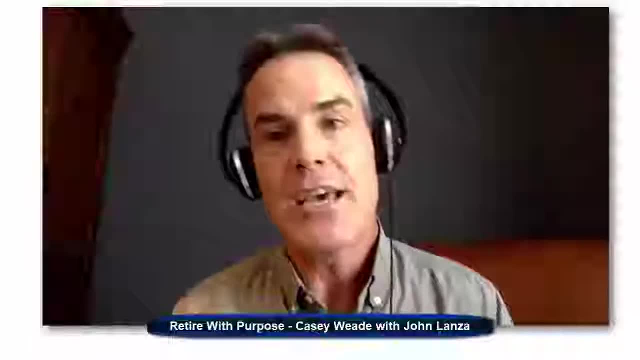 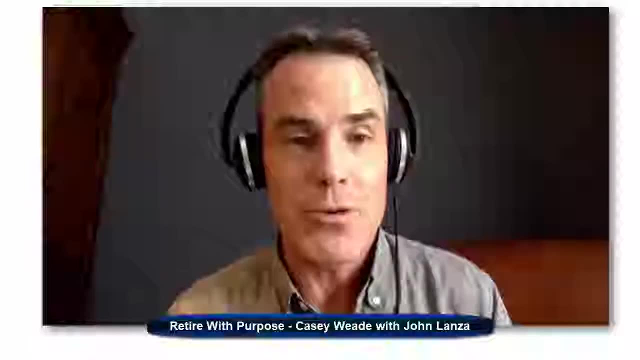 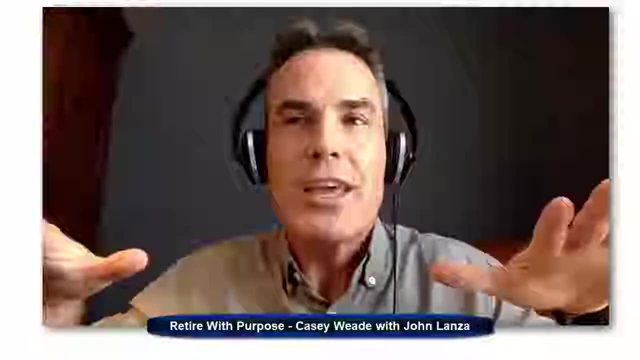 And if it turns into this kind of tit-for-tat, which is, if you want to get whatever money you've assigned to that task done, it's going to be almost a nightly ritual where you are threatening to take away their money. And so, like you talked about, the more we can kind of surround positivity with money and just make it that way. 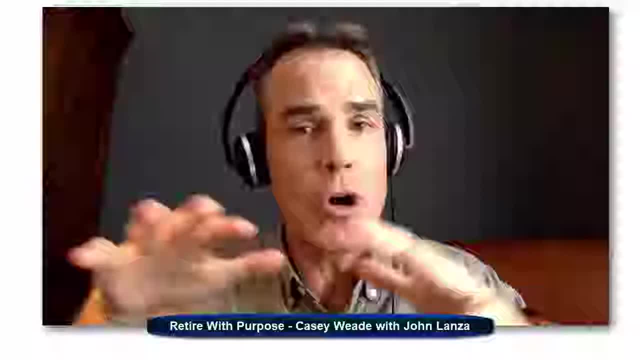 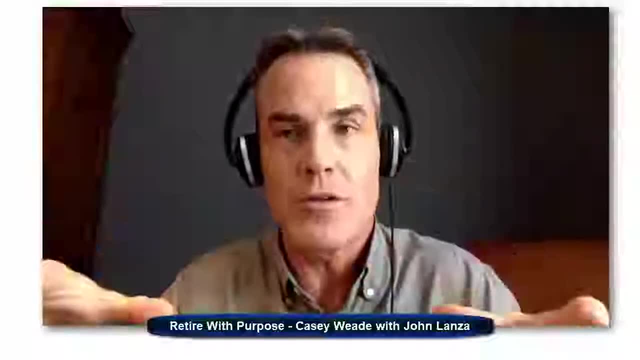 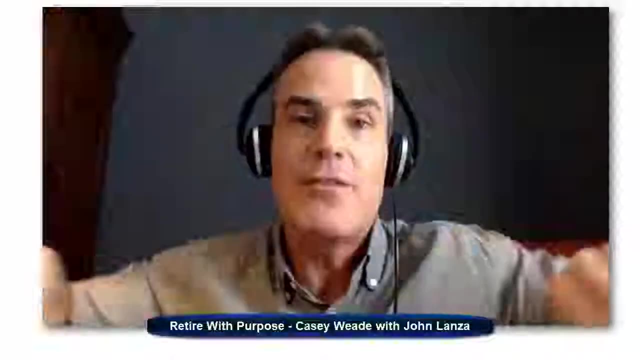 Yeah, It's something that is just a tool, That's all it is, Because we want to get to this point of money empowerment and that really is this point where you feel comfortable and in control of your money. The more we can kind of decouple those chores and allowance and the more we can decouple negativity and money, the better off we're going to be. 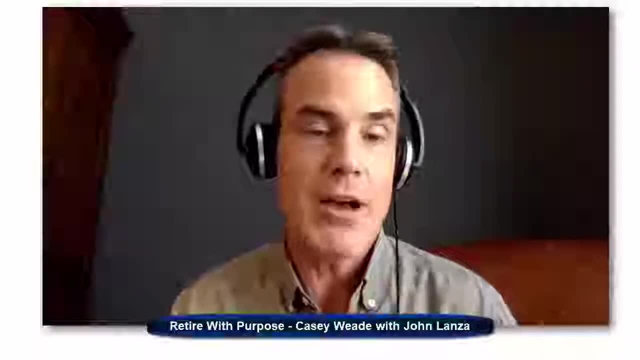 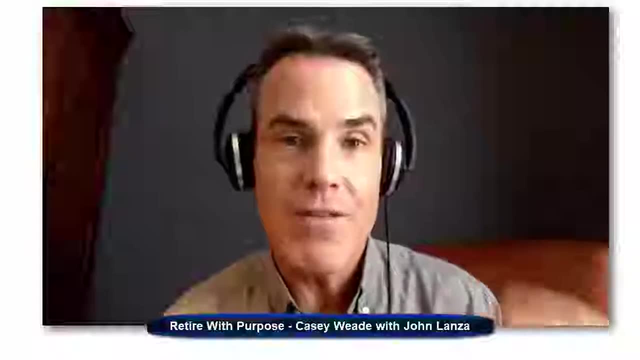 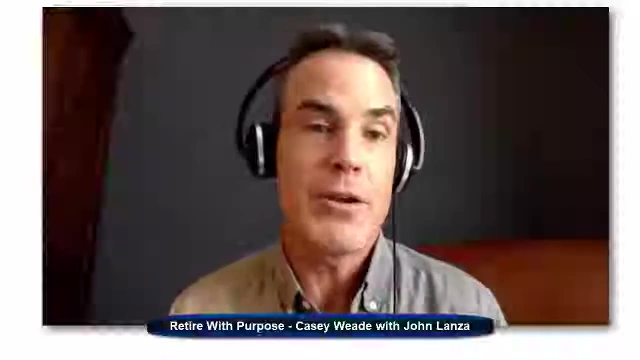 Because we want an open conversation with our kids about money. That's a lot of what the purpose of doing this is is that by setting up an allowance with your kids from a very young age, you're setting up an ongoing conversation with them that you're going to have throughout their kind of period that they're going to grow up with you. 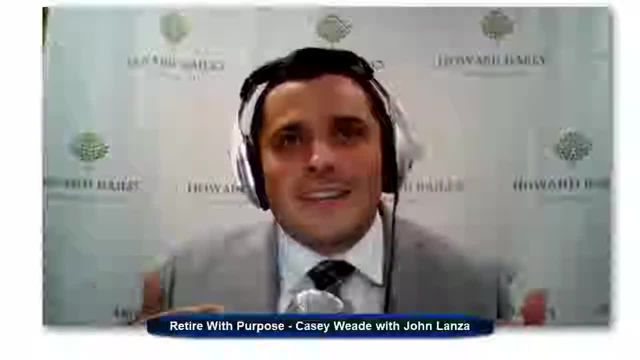 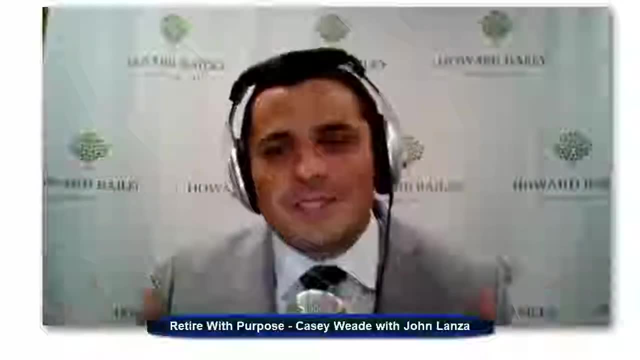 Maybe this is a likeness or a comparison I shouldn't make, but when I was growing up, I always had animals. I was always training animals, and one of them being dogs, And I've always had a dog ever since I was a kid. 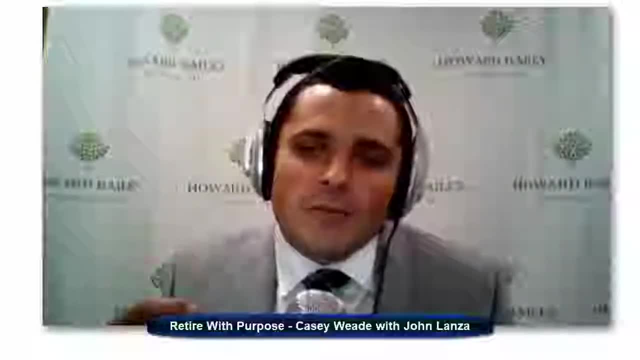 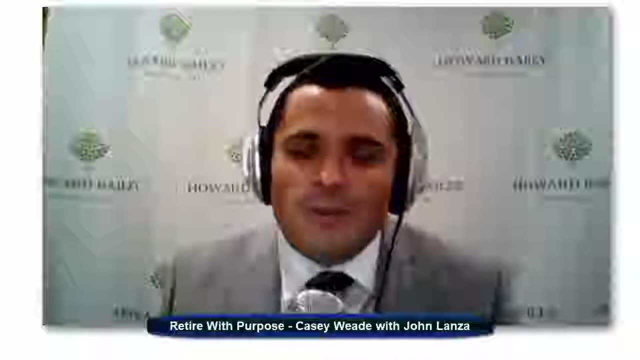 And one of the ways that we train that dog is: you be careful You don't give them a treat. You give them a treat every time they do something right, Because then they won't do that anymore without the treat You teach them. 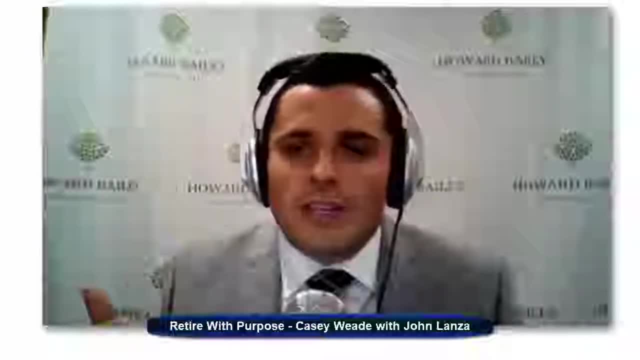 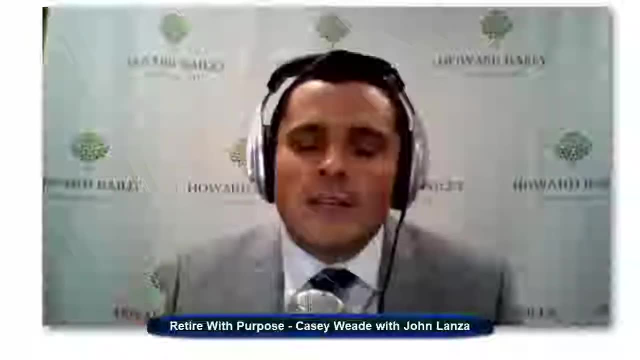 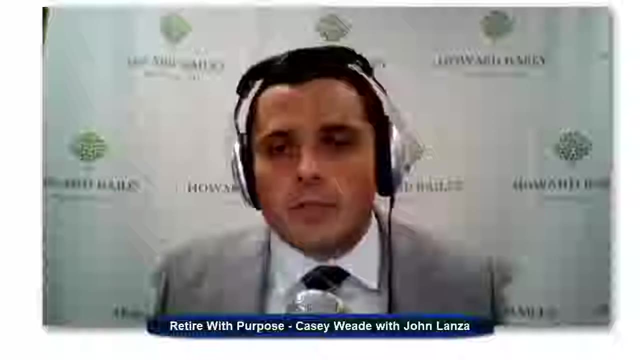 And dogs. they love being rewarded just with a pat on the back, a scratch behind the ears, because they're helping, They're contributing, They're helping their owner, They're helping their master And I think, as children are growing up, you get to a point if they're doing the things they're supposed to be doing- making their bed. 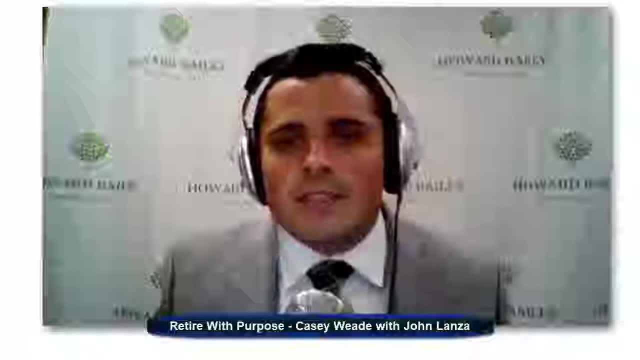 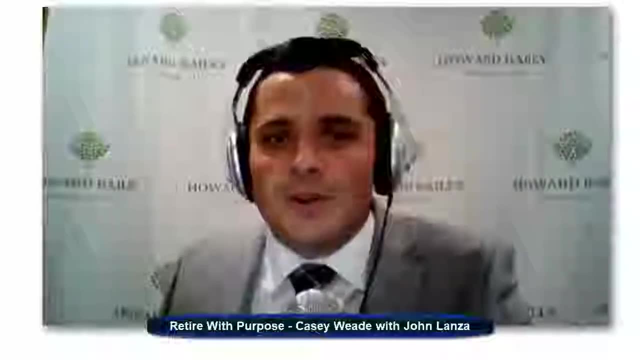 they're just contributing to the family, And that becomes in and of itself a bit of a reward. If you pay them every single time, well then I can see. then it can easily snowball to a point where you run into a little bit of trouble. when they start getting a big enough allowance or they start getting a job, They go well, I really don't need to do that anymore. I guess I'll go ahead and forego that $4 for next week's allowance. I'm just not going to make my bed. 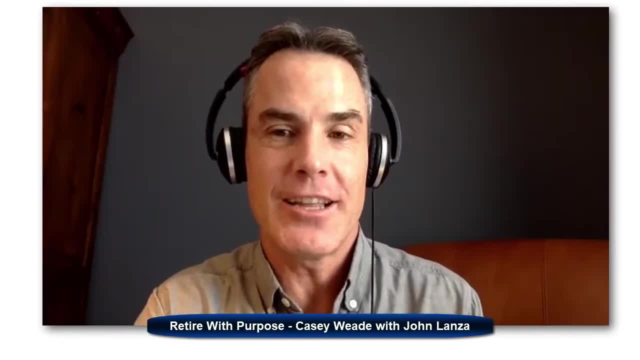 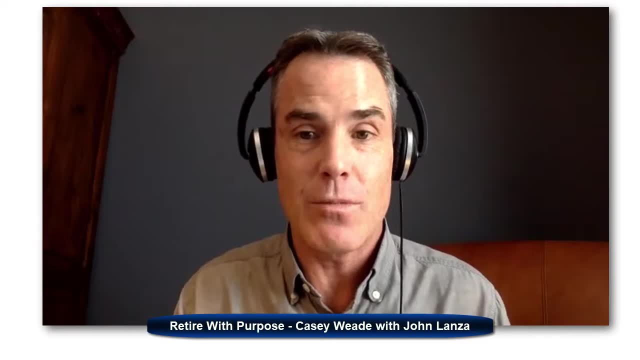 Yeah, I think you're bringing up this incentive thing And this is a little bit off from that particular point, But the idea that you're talking about the dogs the same with humans. I don't know if you've read Daniel Pink's Drive. 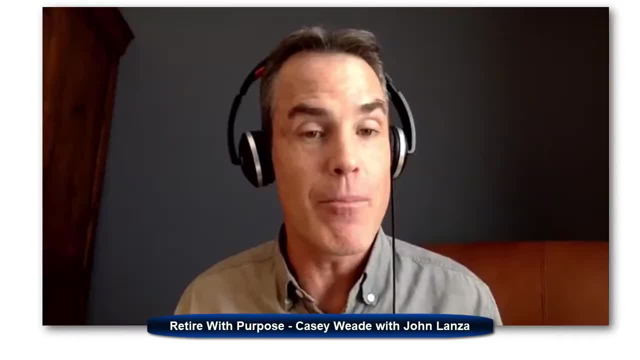 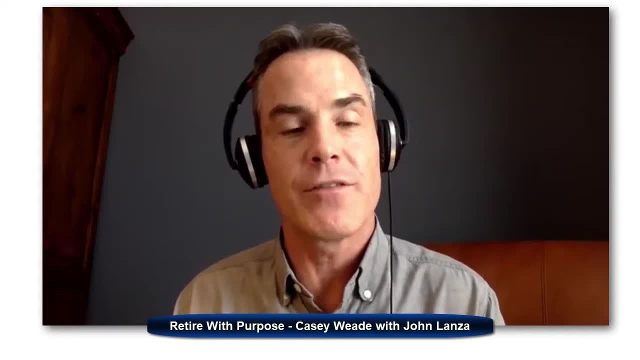 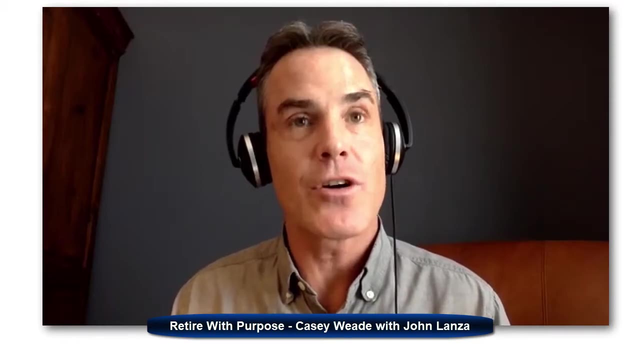 I have. Yeah, Okay, So you know about. when he talks about motivation, he says that incentives work very effectively. Rewards work effectively if they're not consistent. Yeah, And this is a good thing to realize. So for our kids, they have their own allowance. 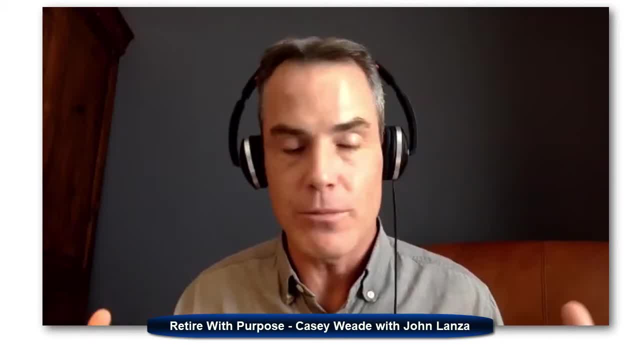 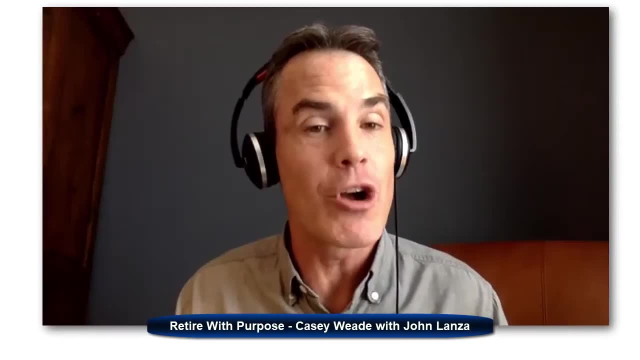 We don't buy a lot of things for them, aside from food, to go to school and your basics. You keep clothes on them, We keep them clothes, But they're actually responsible for their own clothes. now, right, So they have to buy their own clothes. 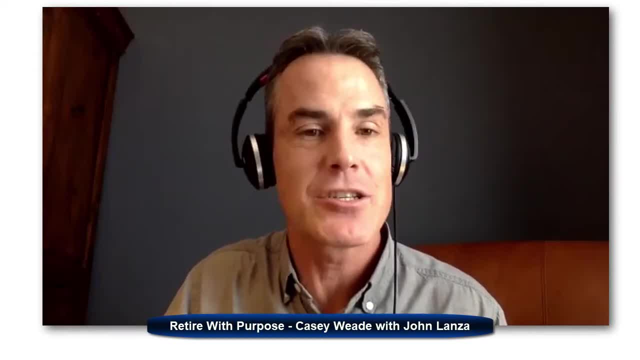 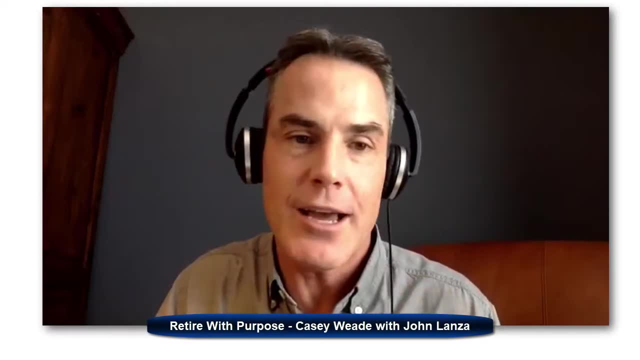 But that doesn't mean, as a parent, that you can't splurge once in a while. And the once in a while because parents will ask me this all the time. They'll say, oh, there's this one time that I would…. 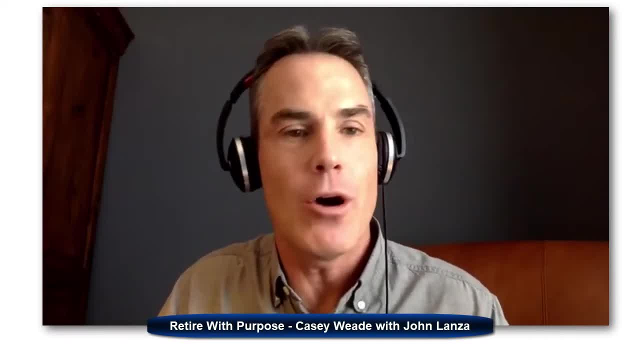 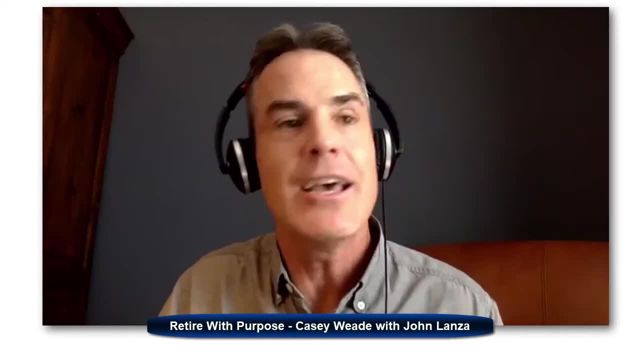 Is it wrong of me to have said, oh, I'm going to buy you that pair of shoes or I'm going to buy you something, when that's supposed to be their responsibility? If you do it every once in a while, it's perfectly fine. 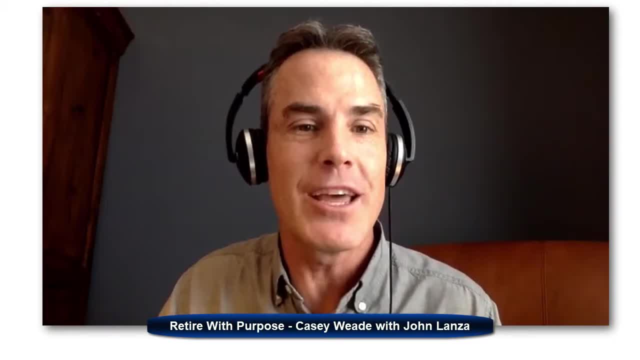 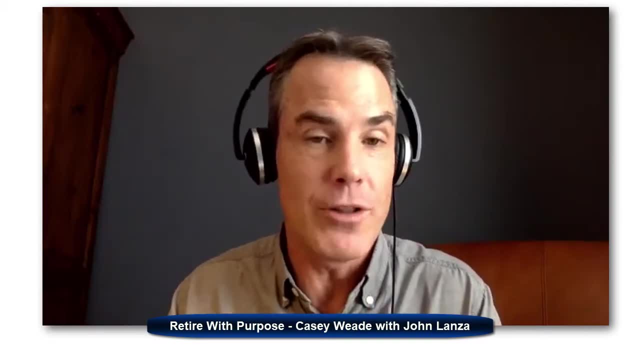 Like that's your parent prerogative. What I'm getting at like when we talk about our framework here. what you don't want to do is set up an allowance where they're responsible for, for example, clothing, and then they're just begging you for clothes and you're caving in on a consistent basis. 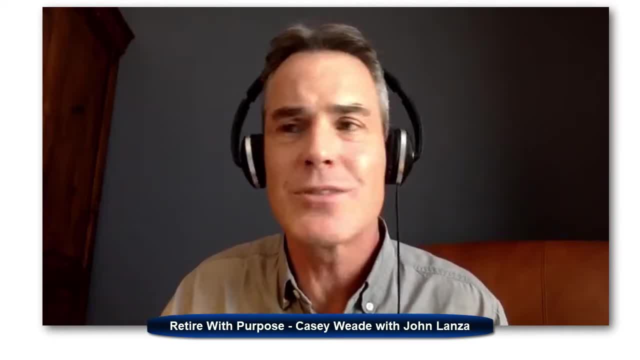 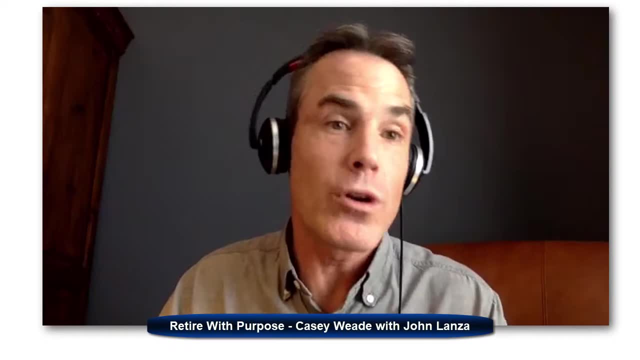 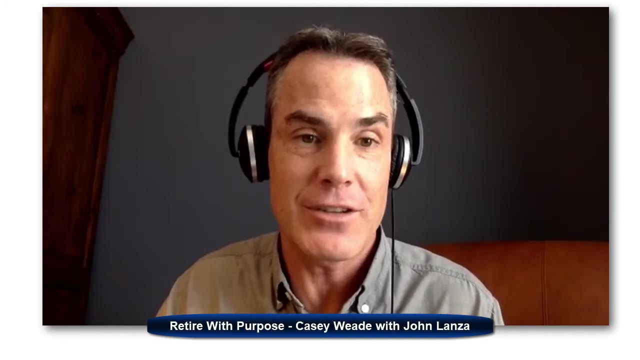 That doesn't work, But once in a while it's wonderful. It's a wonderful thing to do as a parent, It's a wonderful thing to receive it as a kid And it works very effectively as an incentive for kids And if it's not a consistent thing, they're going to get a lot more benefit out of it. 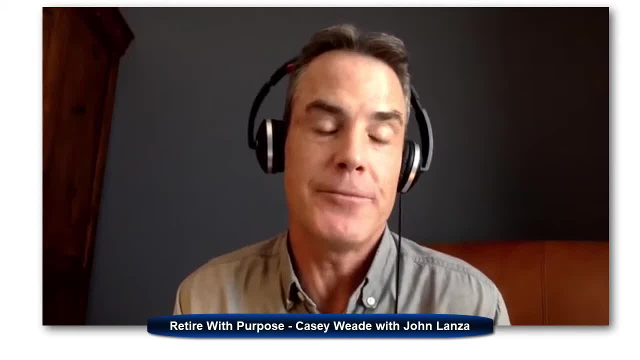 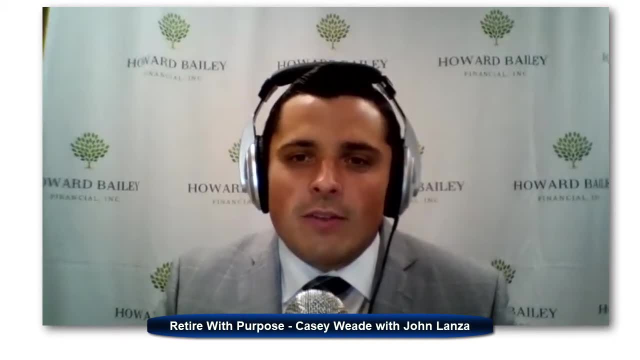 from like an emotional and happiness standpoint as well. I've got to believe that most of the audience right now is wondering how you got your children to pay for their underwear And their socks. You said 12 and 15 years old, So they're literally paying for all of their clothing. 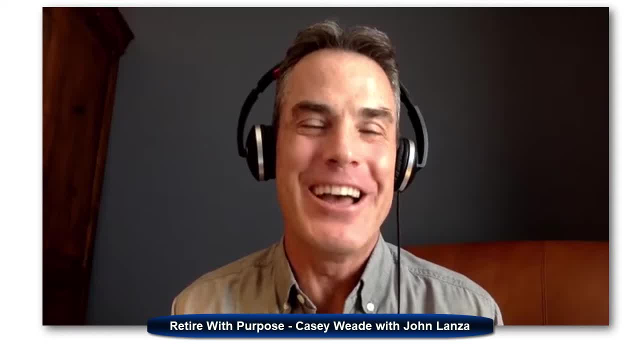 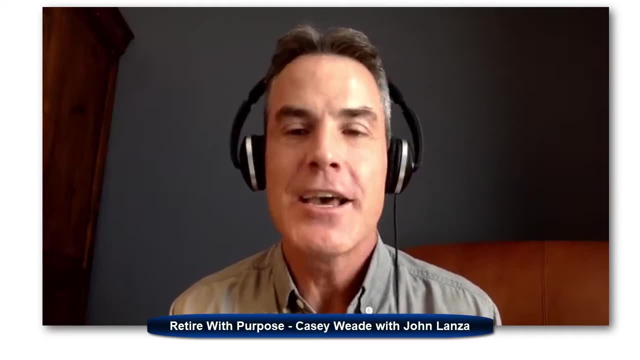 Okay, You caught me on the underwear. We will buy their underwear from most of the time and some of the socks, But the clothes, yeah. So the way that it worked for you know, maybe we should talk about like the basic. 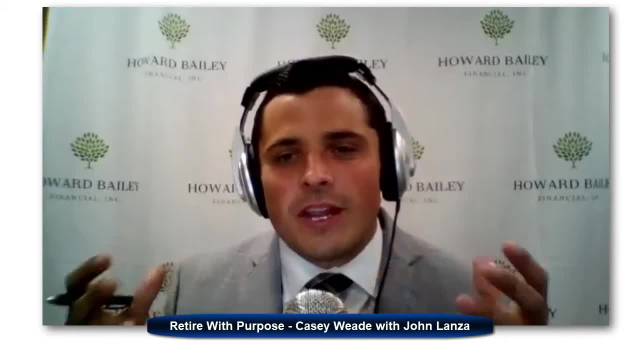 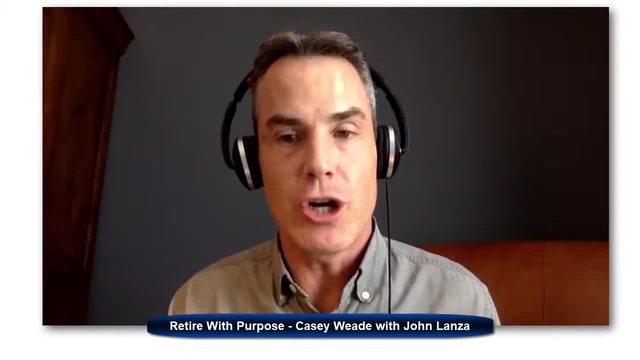 allowance first. Yeah, Why don't you just share with everyone kind of the framework before we get too deep? Yeah, Let's do that. So the way to set up a basic allowance is you set up your three jars. So the three jars are going to be save and share and spend smart. So the save is for longer term items And for a younger kid. those longer term items are not going to be that long. They're going to be something that's going to take, say, two to four weeks to save. Share is for charitable giving. And then spending- or spend smart- is for stuff that they want to buy anytime they go to the store. So the easiest way to start is $1 per week. Spending is $1 per week per age of the child. So your five-year-old gets $5 per week. 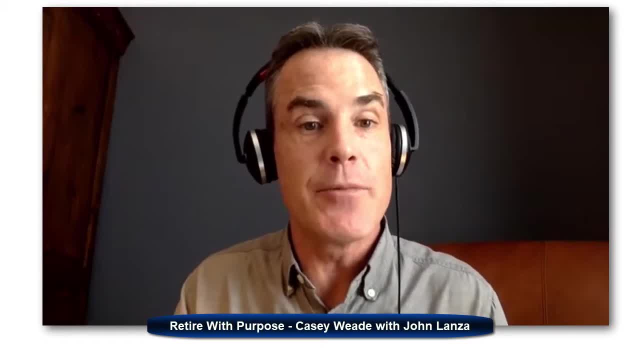 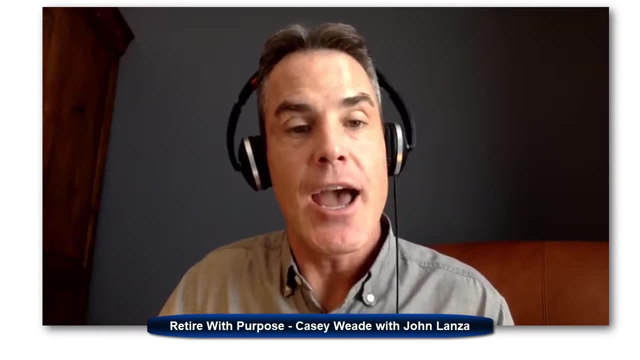 And the way we broke it down was because we're a little bit lazy- is we would just give them $5 and one would go in the save, one would go in the share and then one goes in the spend smart jar And the thinking behind, or three go in the spend smart jar, or they can go into any of 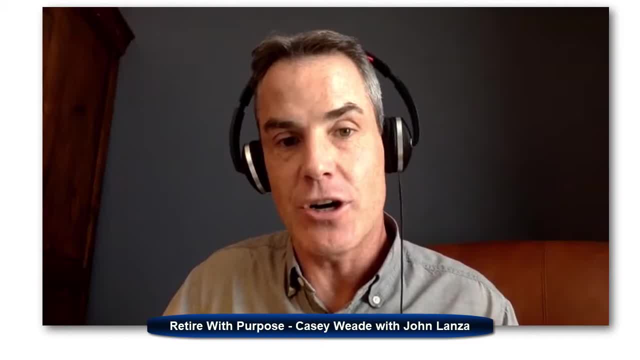 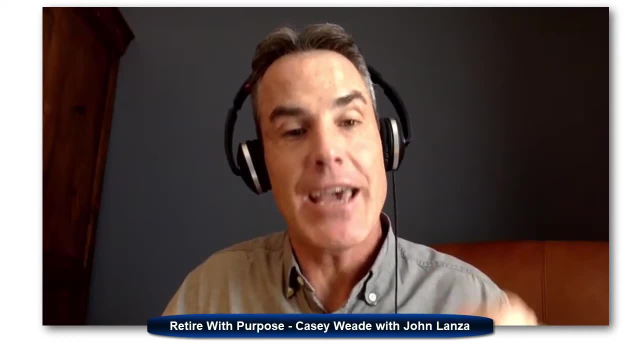 the jars, But the thinking behind it is the one that goes into. the save jar is kind of opting them in or kind of nudging, if you know that concept. So they're going into this idea that they should pay themselves first. So that's what the save jar is. 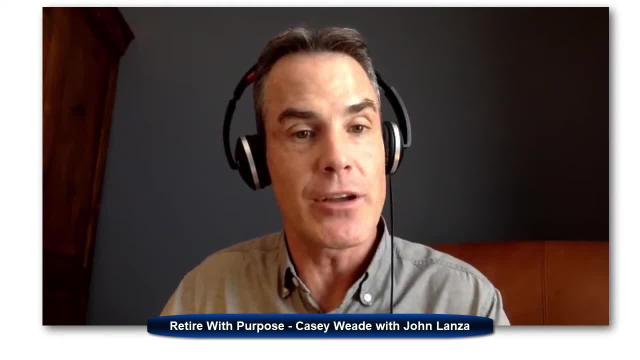 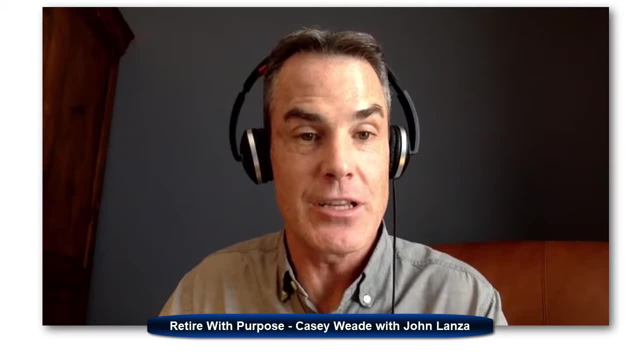 Then share is money that's going to charitable giving. We all kind of agree that it's a good thing for us. If you've read the book Happy Money, we realize that investing in others is a great way to use money to generate our own happiness. 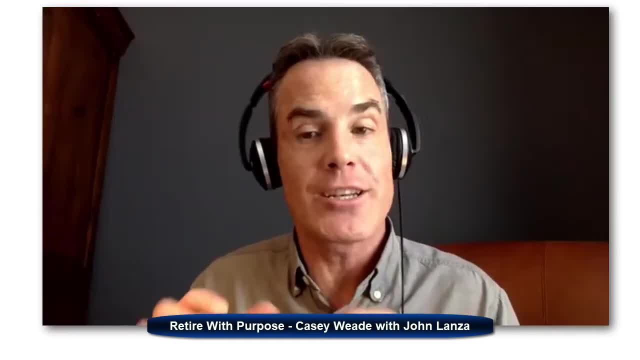 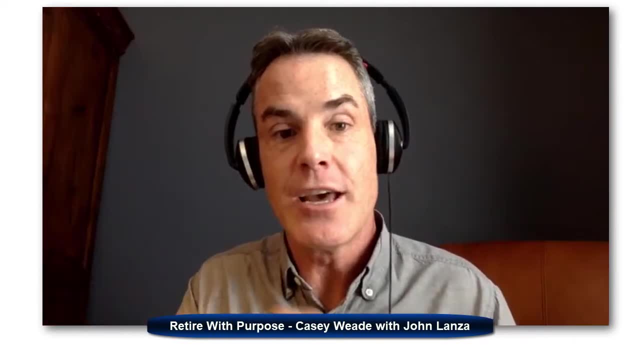 Yeah, And then the $3 is the kind of autonomy, the autonomous dollars. So those are the discretionary dollars that they get. So the one and the one have to go in the other jars, But the $3 can go anywhere. 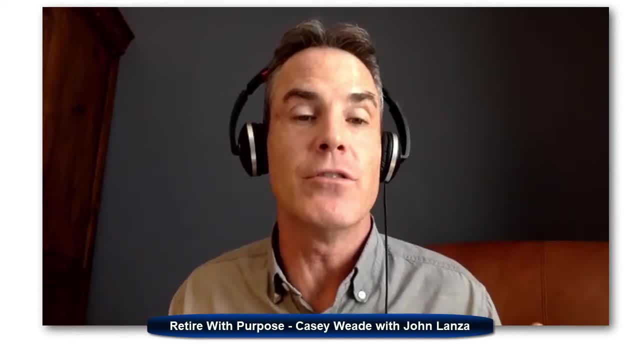 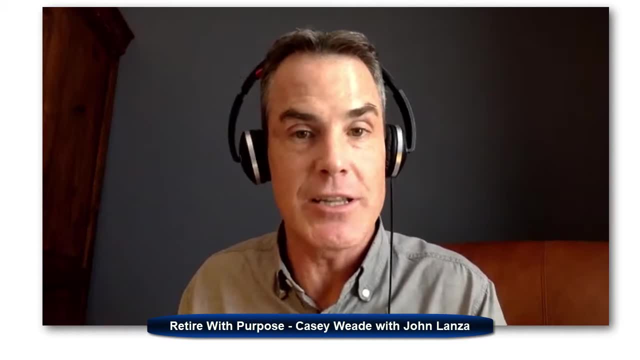 They have control of it And this is really powerful for a young kid because they can put it all in the spend money and then when they go to the store they can go buy whatever that is and they can accumulate that spend smart money, or they might be saving for a goal. 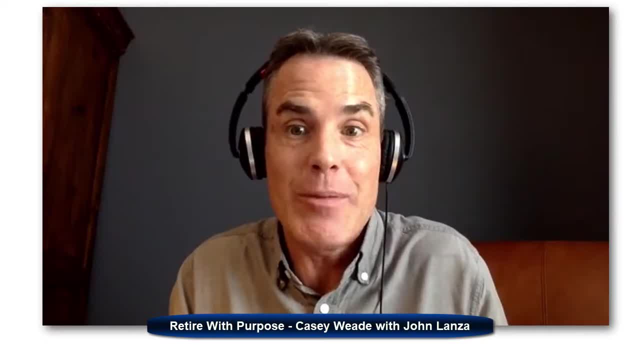 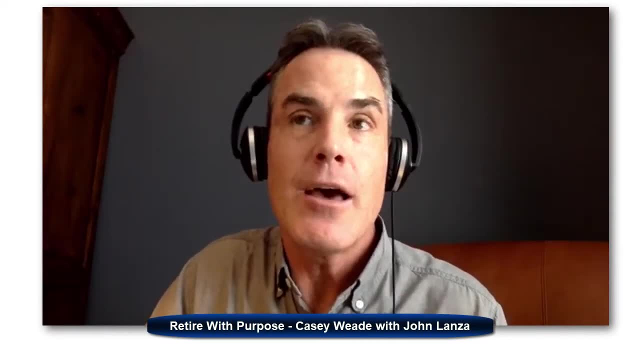 They can put it in the save jar. They might be just charitably oriented and they might put it in the share jar, but it's their money And that's really a key part here, And parents have to get comfortable with it and it's not easy. 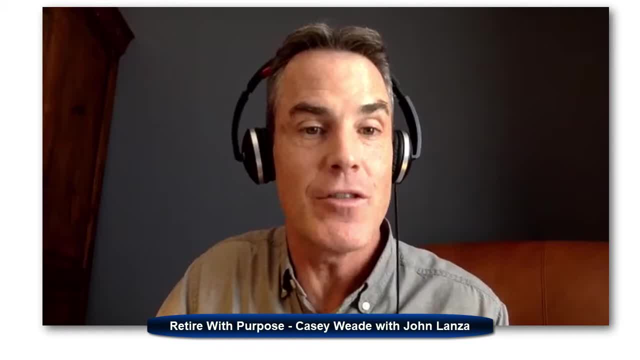 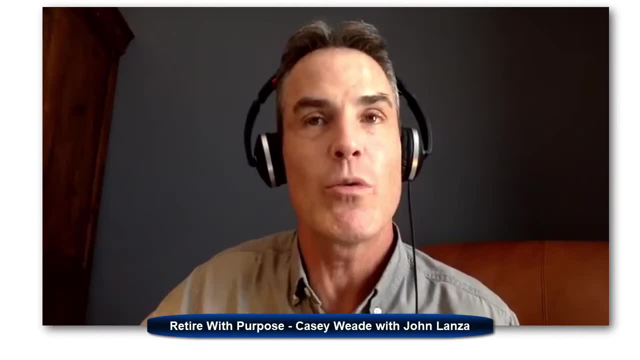 Because they're going to make mistakes with that money. but that's kind of the point. In a low-stakes environment, having them buy some things that might not be things that you agree with is kind of okay, because we're trying to get them comfortable with making. 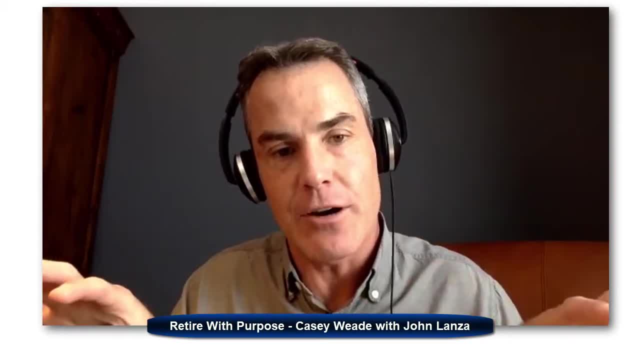 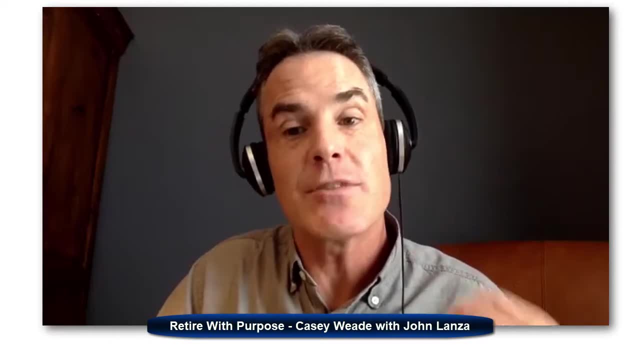 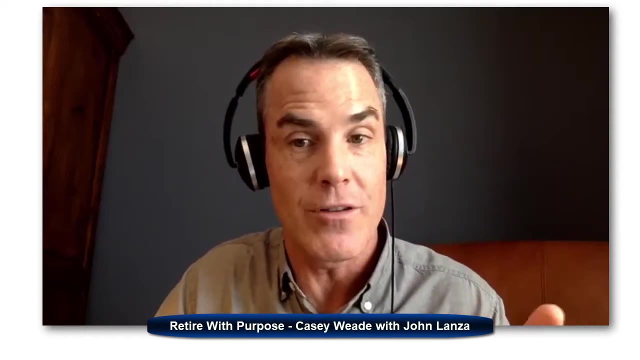 smart money choices. So that's your kind of basic setup there, with your allowance, And then one of the kind of immediate things you want to do is get them saving for a goal and pasting a picture of that goal on the jar. The reason you want to do that and you want it to be a short-term goal for a five-year-old. 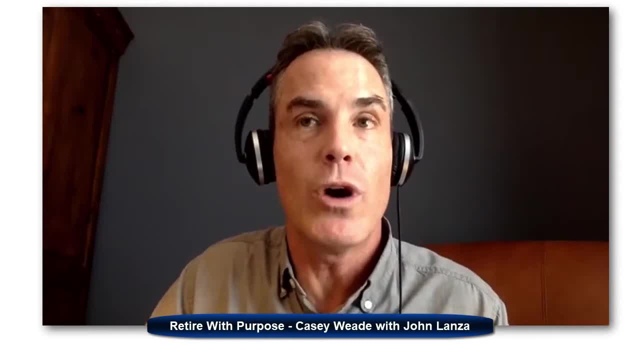 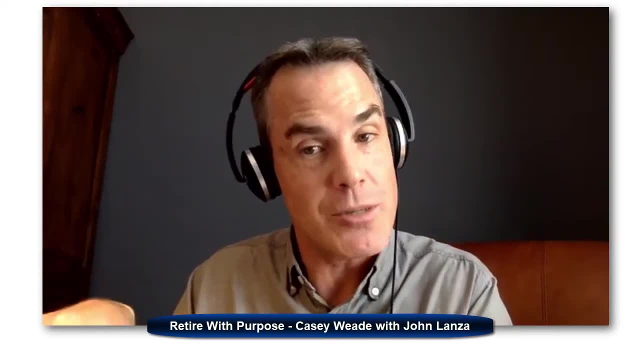 because they'll lose track pretty quickly. You want to do that because you want to get them thinking, when you're giving them the money, those three dollars that you know what, maybe I won't just put it in the spend smart, I might put it into save because I can get to this goal faster. 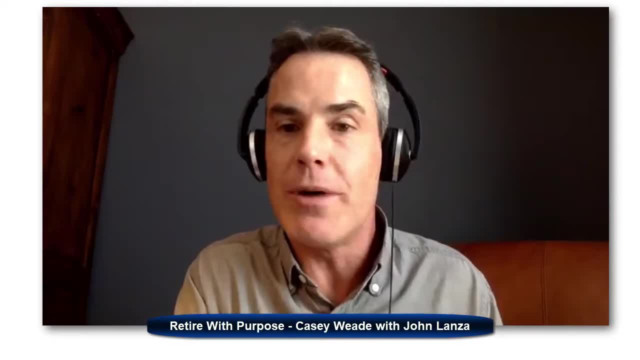 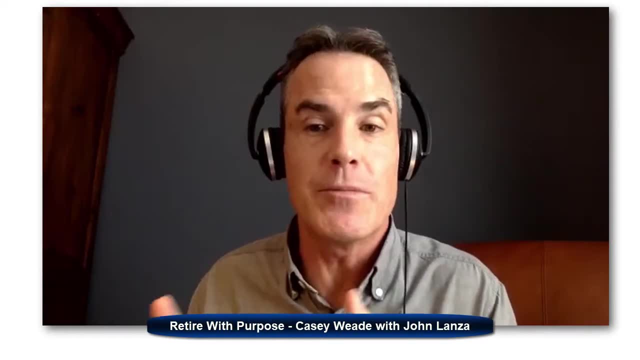 Now, it doesn't mean if a kid is putting all their money into save, that's not necessarily a positive or a negative. It just is what it is. We don't want to keep them from spending their money, But if there's an opportunity to teach them about delayed gratification, why not take? 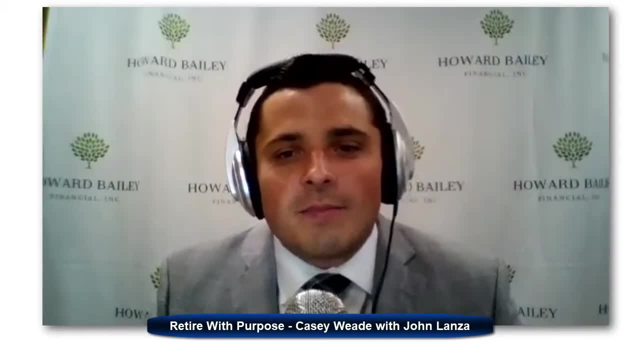 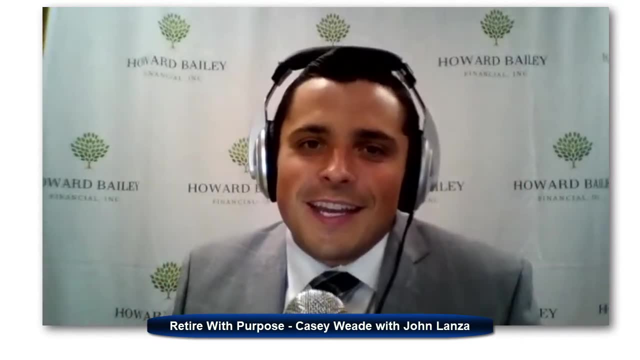 that opportunity? Yeah, We're. currently we set up the first save spend smart jars for our and also share for a three-and-a-half-year-old And I asked him what he wanted to save for and he said he wanted to save for a lizard. 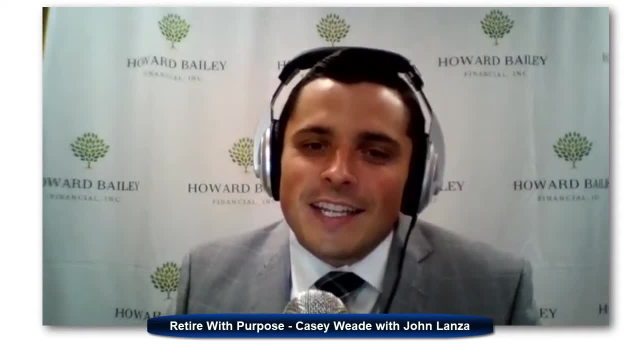 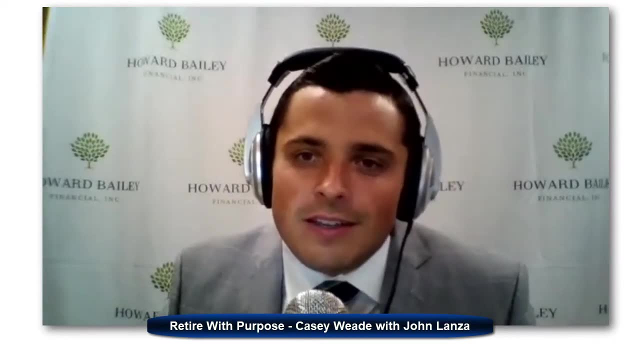 And so right now we're saving- for a lizard, I think. So I tried. he wanted me to draw a lizard to put on the side of the save jar. So I drew my best likeness of a lizard And he went up there the other day. he looked at his jar and he said: he said we're saving. 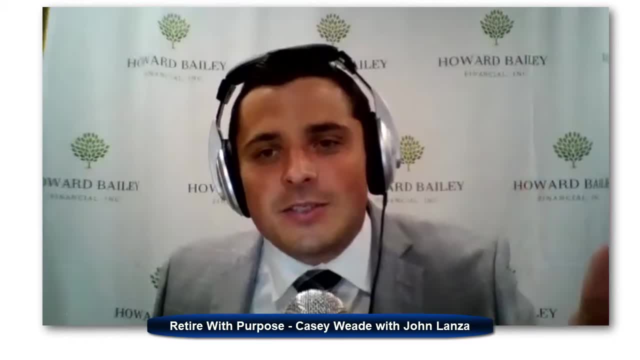 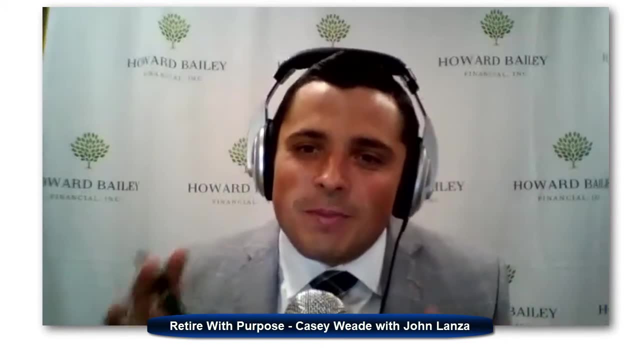 for your lizard. He said that's a squirrel, No, it's a lizard. So I think it's important- unless you're an artist- to actually go find a picture of whatever you're saving for and paste it right there, so they get that good visualization. 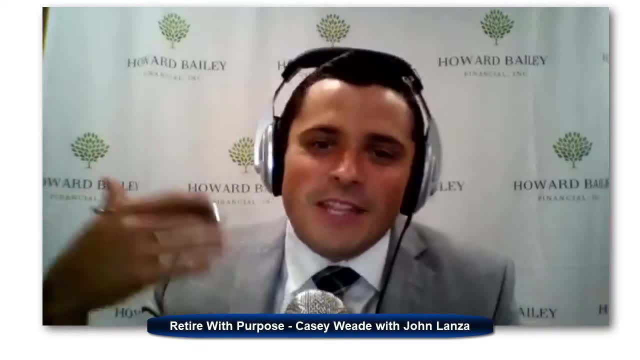 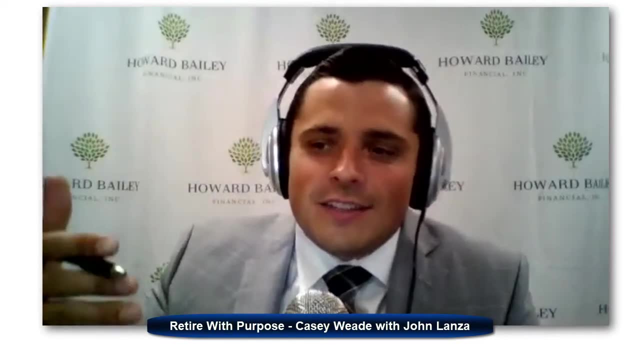 I mean in all seriousness. it's so important for them to be able to visualize that goal and not think that they're saving for a squirrel. They know exactly what they're saving for. They know exactly what they're saving for. They know exactly what they're saving for and they're thinking about it. 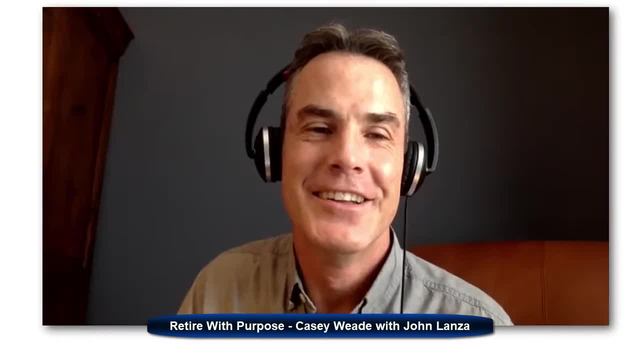 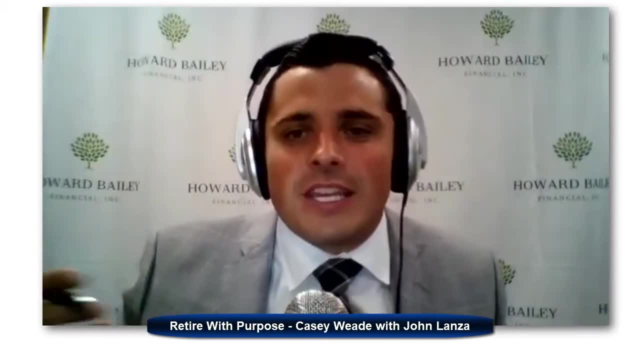 Every time they put anything into that jar, every time they have to make that decision, you know they're making a smart decision right, Because they actually know what they're doing. especially at the younger ages, I think you know it's difficult for them to continually keep that visualization in. 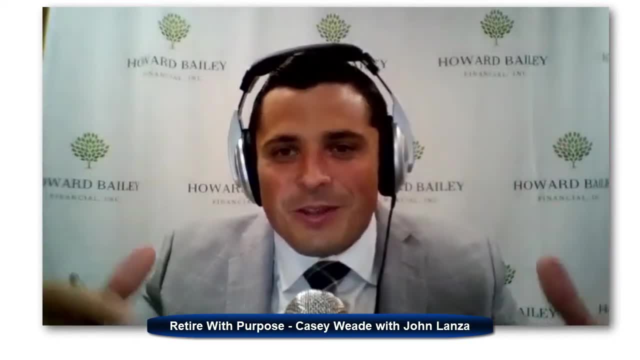 their brain. So we keep that jar right in front of him Every morning he wakes up, he rolls over and it's right there. So he's thinking about it every day. Yeah, you're doing it totally right, Because that's what you want. It's a good reference point. So when you're doling out the allowance you can always point You say here's your three For him. he's probably just getting $3, $1 in each jar, right? Well, you know, we started with $3 and I thought he wants to save for a lizard. You know that lizard is, it's, you know, probably a $20, $30 lizard, And if he gets a dollar a week going into a save jar for a three-year-old, that's a lifetime. And so we actually just say: you know, why don't we bump it up? Just a little bit. So we did $6 a week and then we do $2 in the save, $2 in the spend and $2 in the spare jar. But as I do the math, I think you know we just kind of have to reevaluate that every year, right? 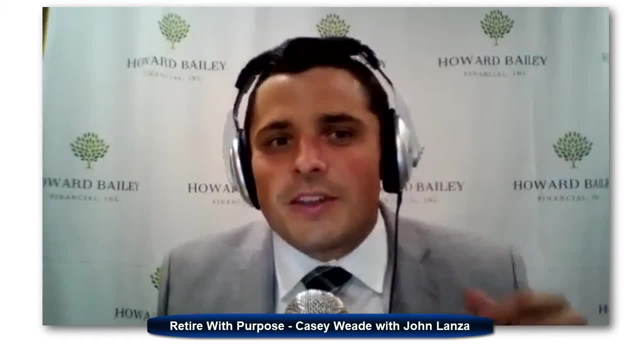 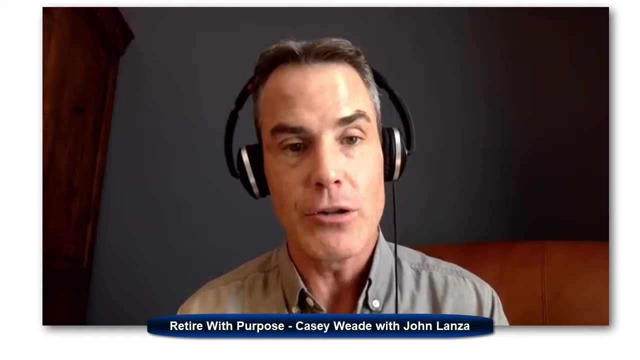 Do a little annual review, as you kind of laid out in your book. Yeah, You know. the other thing you can do is when it's a goal because you've recognized, yeah, for a three-year-old they're going to lose track if it's going to take them, you know. 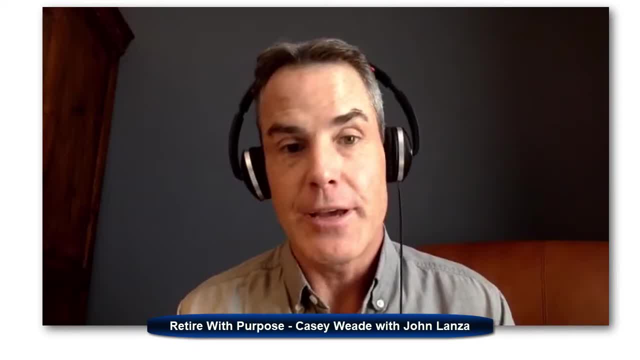 a few months to do it. You can do a matching too, And a matching… Well, we're definitely doing matching ultimately, because he still is going to need it, He's going to need a terrarium, He's going to need food. 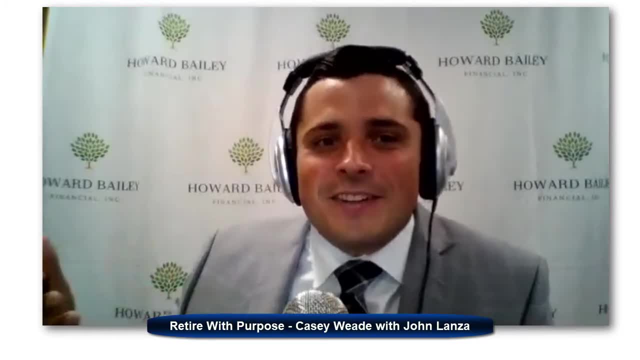 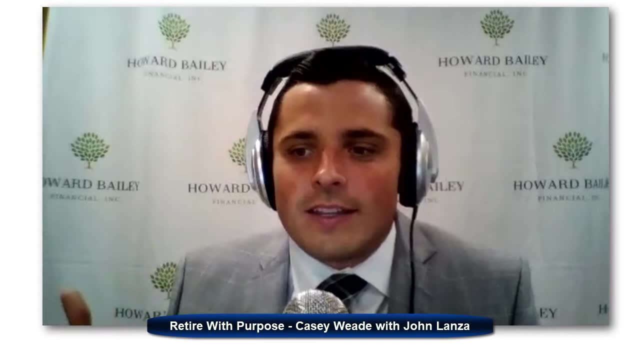 That's true, But in the long term it ends up being a great doing. I think having a pet right gives them the ongoing. it always gives them something. If they want to keep that pet alive, they're going to have to continue to save in order. 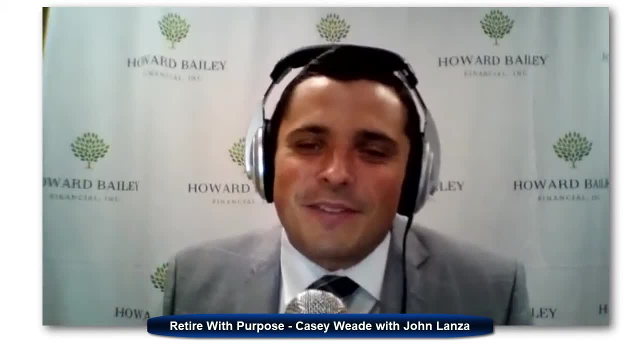 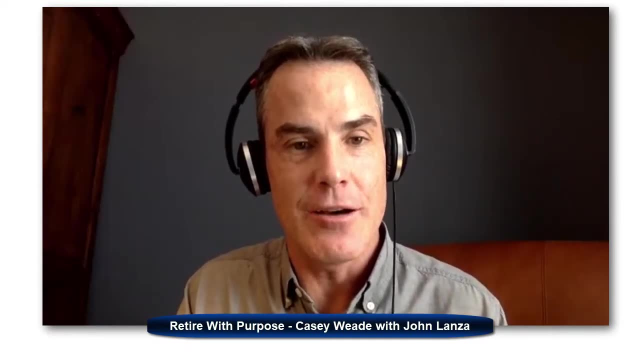 to buy the food and everything they need to take care of it. Yeah, See, this is what's so great about it- is the lessons that you are going to be able to teach him as he goes through this process, because he's going to get the lizard and 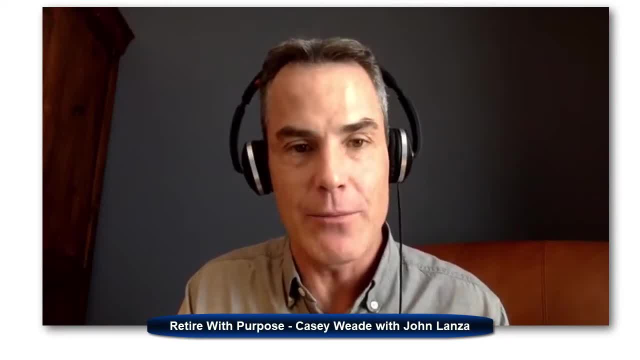 then he's going to have to get food, And you're being smart about it, which is, you're not going to make him be responsible for all the food. You want the lizard to live, and so you'll help him out with that, Of course, 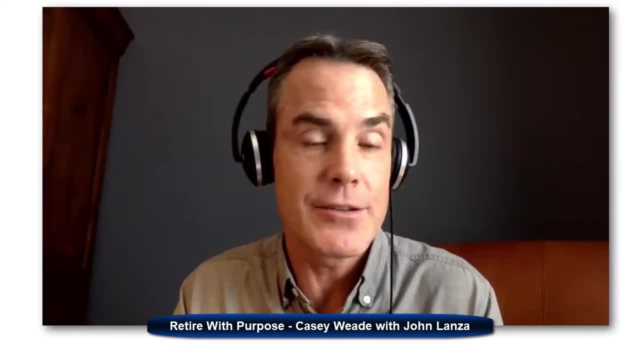 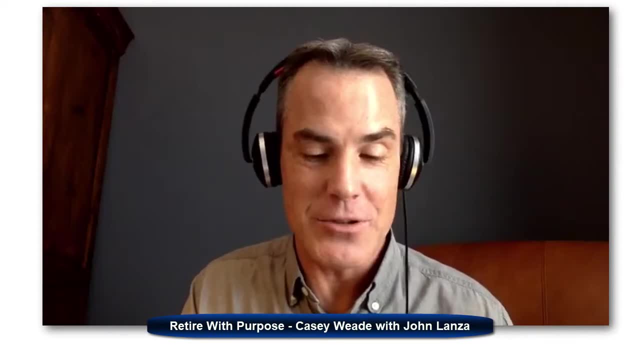 But you can have him contribute some of that money, some of the spend money, to the lizard, And then you're… That's a lesson, Because I was… Yeah, Yeah, I was one of the first people…. Then we're on creating a budget, right? Right, That's really what you're getting at. Yeah, And the kid… Because I remember when I was a kid, we had dogs too. We don't have a dog now because my wife is allergic, but my kids definitely would have roped me into getting a dog, because I roped my parents into getting a dog and then 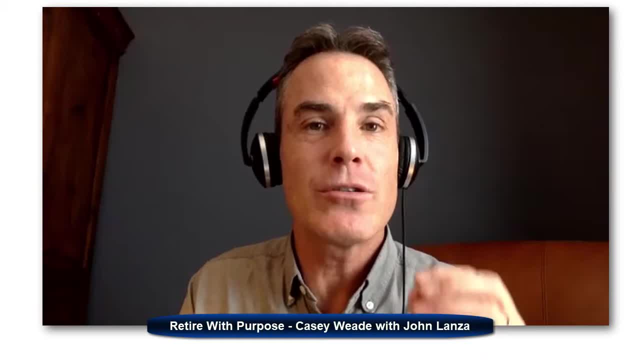 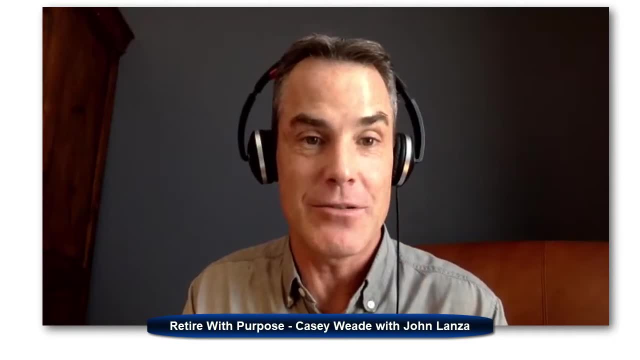 I didn't really train the dog And so you're from a very early age making them understand that there is a mundane…. I mean, pets are fantastic, But there is a part of it that's not that much fun. And all the lizards watching them eat is kind of fun. 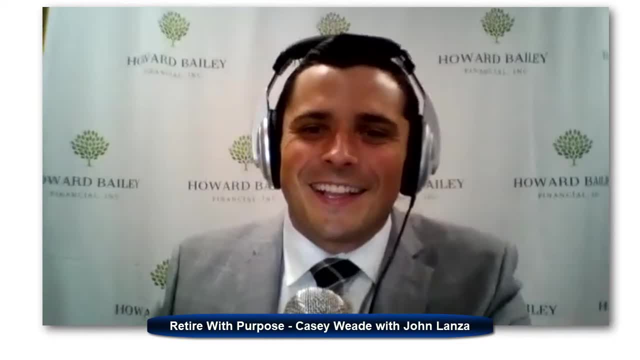 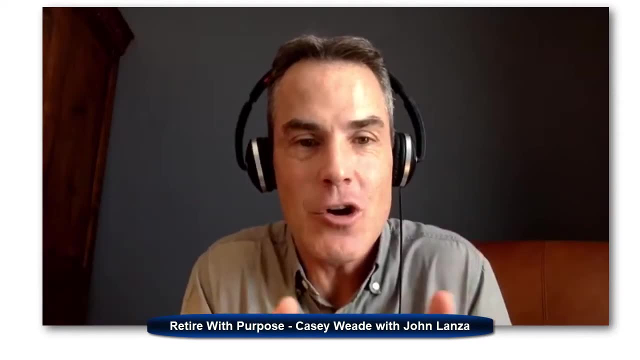 Yeah, But having to do it day after day can… It's something you have to remember when you're having a pet. So it's opening up all these kind of conversations And so much of it starts with money and the back and forth that you're going to have. I've just found the back and forth that I've had with my kids about money and talking to other parents about the back and forth they have. It's really a huge part of why you want to start this allowance process from a young age, because all these kids, all of our kids, are being exposed to money by the time they're. 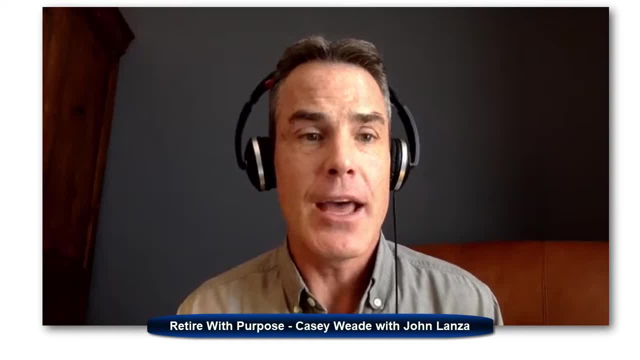 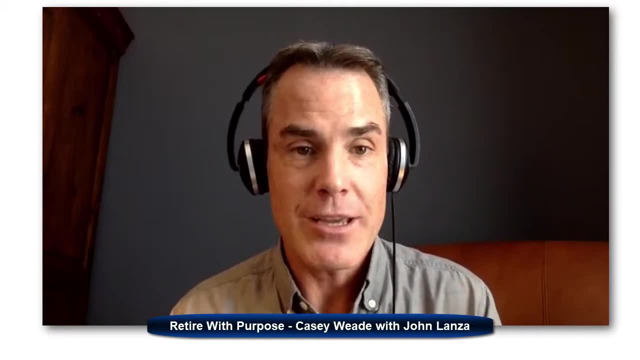 two, because some people will watch this and say three-year-old allowance, And I've even said I think five-year-old five is a good age, That's when we start our kids. But I have no problem with three years old, because before they're two they're learning. 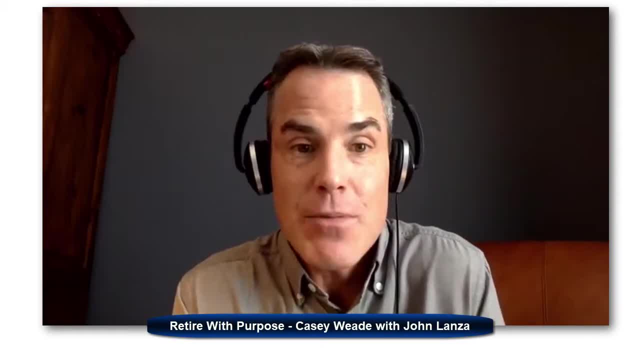 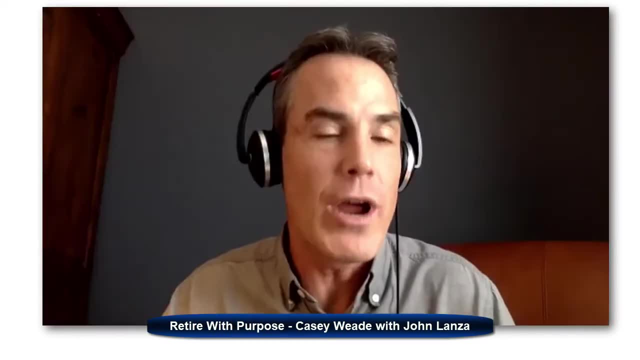 about spending. They're learning about consumption. You can't escape it, Even if you keep them away from media. there's billboards, It's just out there And so, if nothing else, first of all, you're aware that there's only so much. he's going. 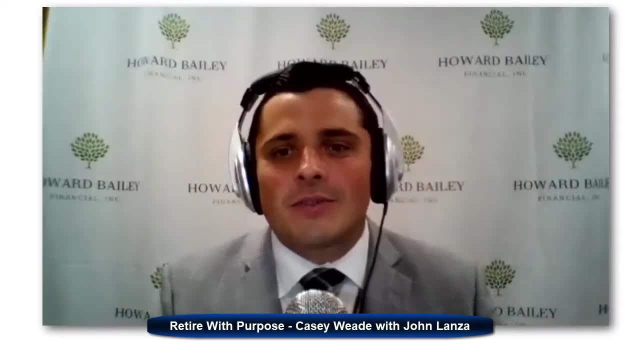 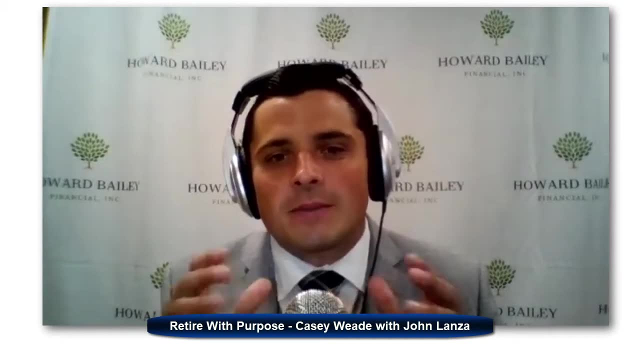 to fully grasp of what's going on. Absolutely, We're really struggling with the share jar right now. That's been our biggest obstacle. So we've got some landscapers, We're doing some landscaping work in our house And he is dead set on giving that share money to his new friends that are playing with the. 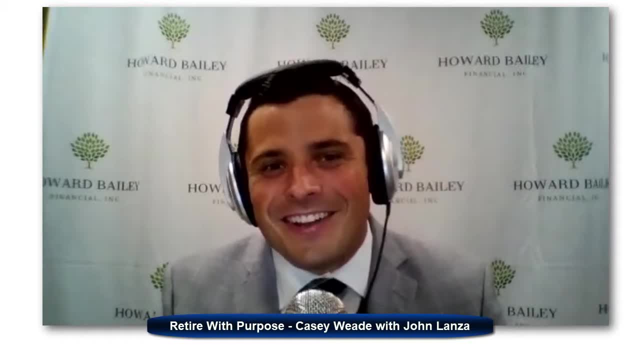 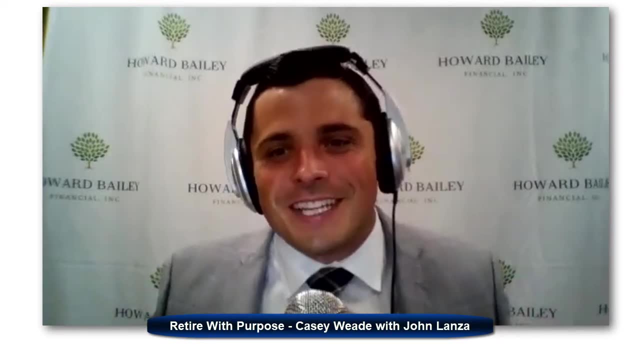 new trees out in our yard And I said, buddy, we've already paid them. I think they got paid enough. Why don't we? And it started with the church. He wanted to give it to the church. He said: why don't we go back and revisit the church? 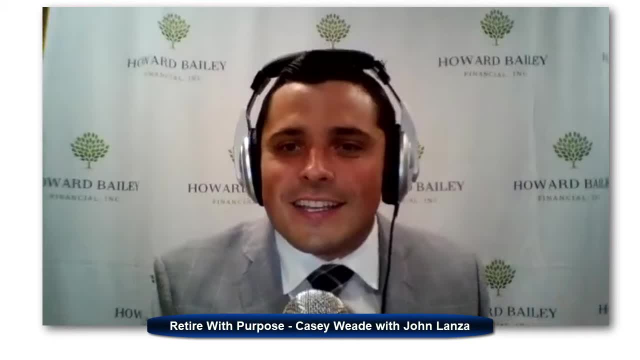 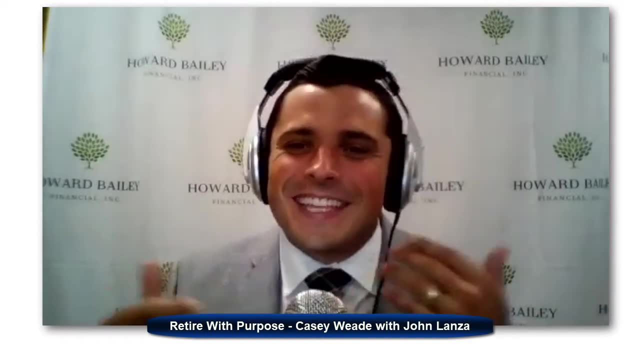 You know, I think why don't we wait till Sunday, And I think that might be a better use of those funds. But that's something that is such a great conversation that you get to have even with a three-year-old where they have difficulty grasping the concept. 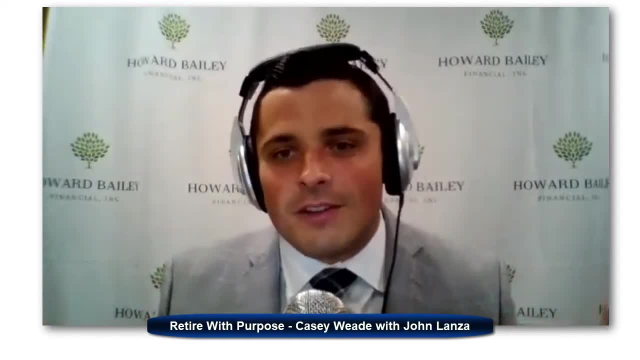 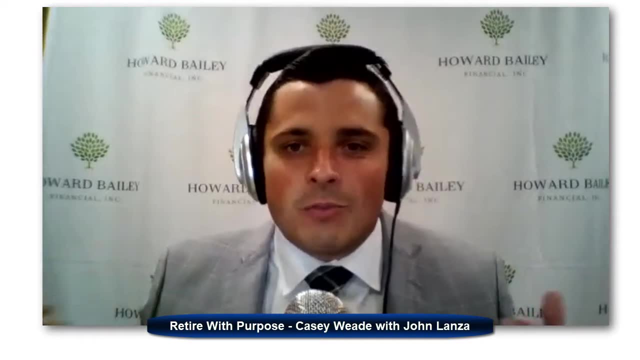 That's how they learn, And so I think that's a great conversation. Yeah, And that's how they learn is to have adult conversations with children. I think that when you treat a toddler like a toddler, he ends up being more like a toddler. 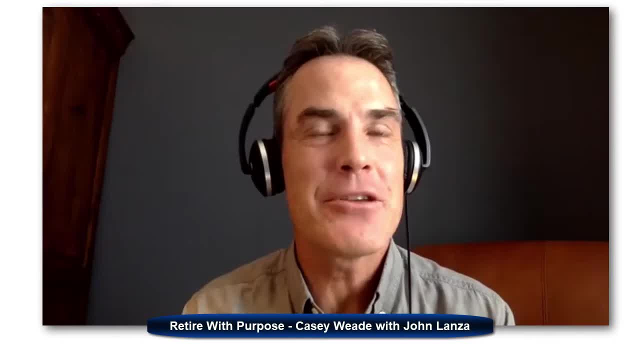 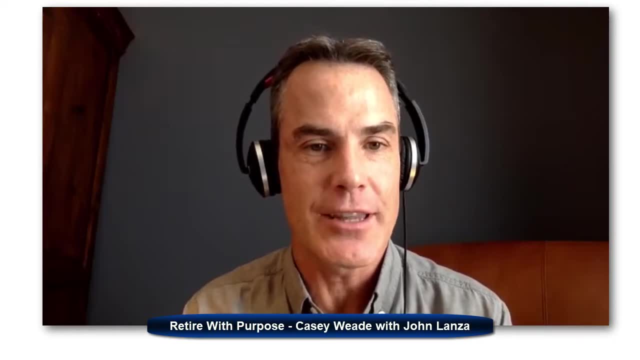 when he's an adult. No, you have those conversations just knowing they're not going to grasp the nuance of the conversation, but you're introducing them. You know, now your son is going to be familiar with these concepts of share and save and 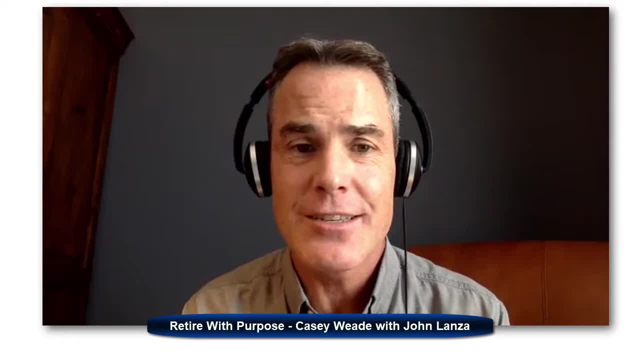 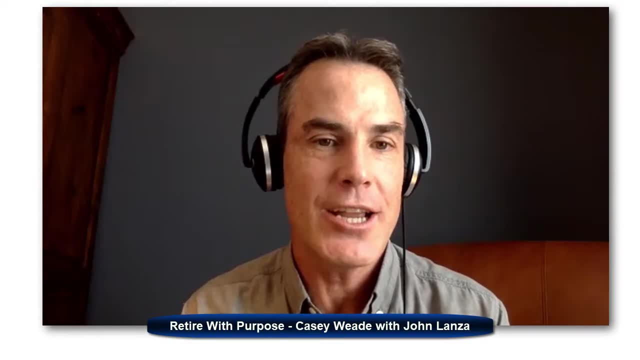 spend smart. He doesn't know what the heck delayed gratification is. He obviously doesn't fully understand charitable giving. But kids are naturally charitable, You know. that's just human nature And I think it's such a great impulse to see that he wants to help these guys out on some. 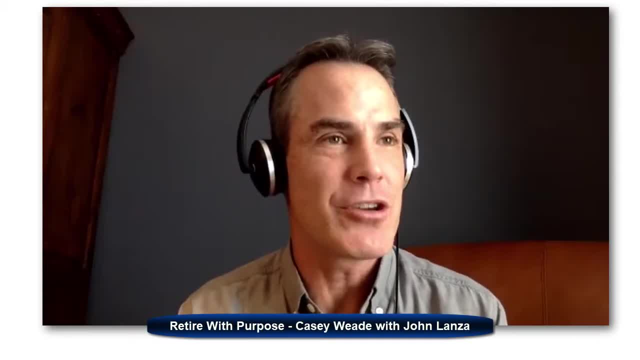 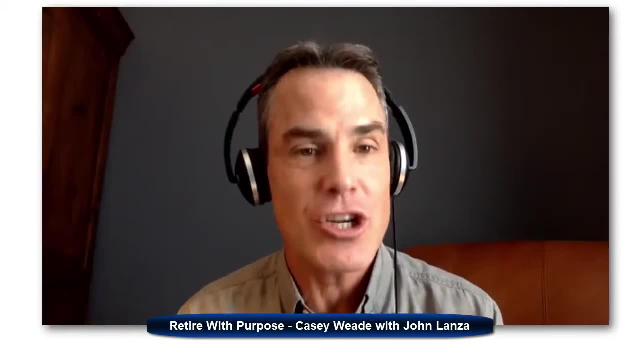 level. I was thinking, you know, maybe there's a way that he could, you know, buy some… Get him ice cream, Yeah right, Yeah Right. I mean, that's such a great impulse to reward. That seems like it would be a great use of the…. 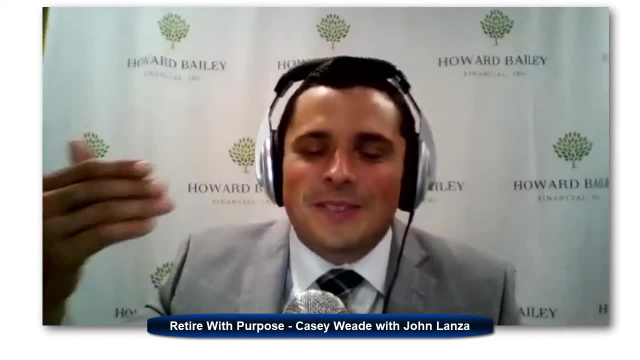 Yeah, And now they get to go out and you take them to the store. You take them to the store, You can count the money out, right, Yeah, Yeah, Well, you helped me there And now I have something to take home with me. 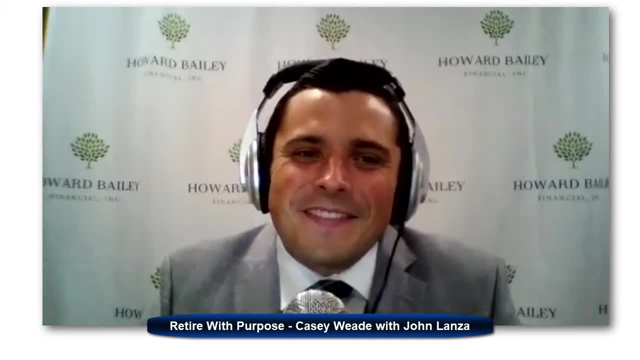 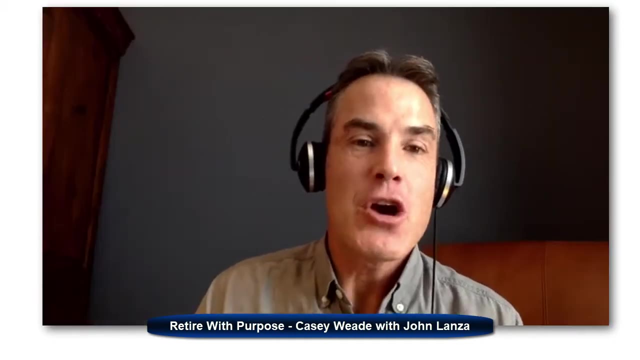 I think you helped yourself. That was a good idea. I have another question that came from one of our fans that I think is perfectly along those lines. Bruce Johnson asked the question: by what definition do you describe money to a toddler? That's a good question. 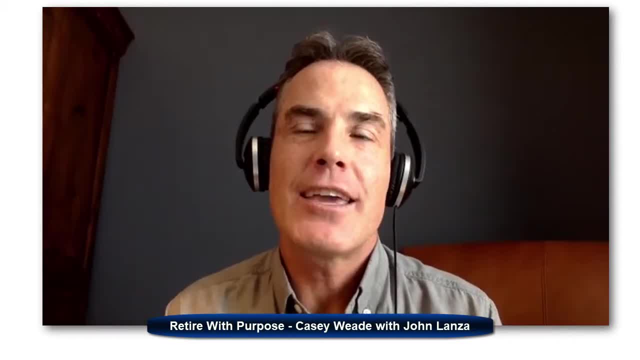 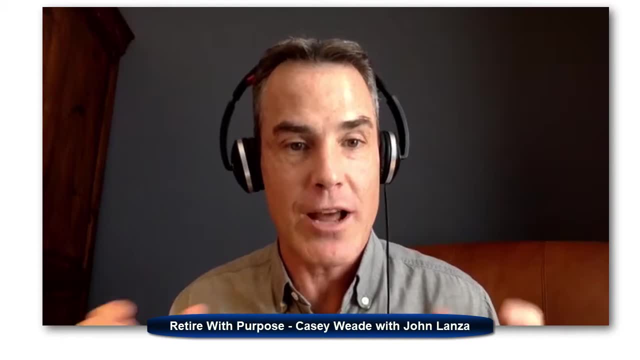 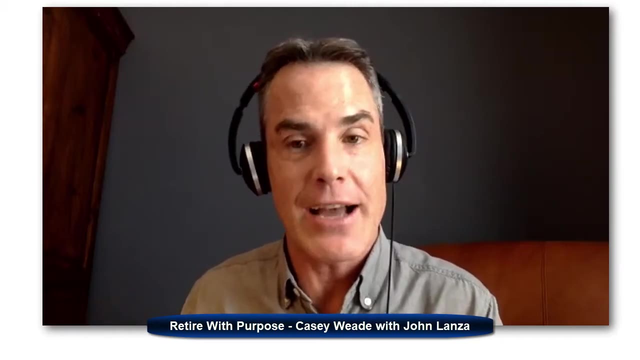 Well, description of money. I guess we tend to talk…. So there's a term called emergent literacy that we're all familiar with. If we're not familiar with the term or the phrase emergent literacy, we're familiar with what it means and that is why we… how it impacts us. 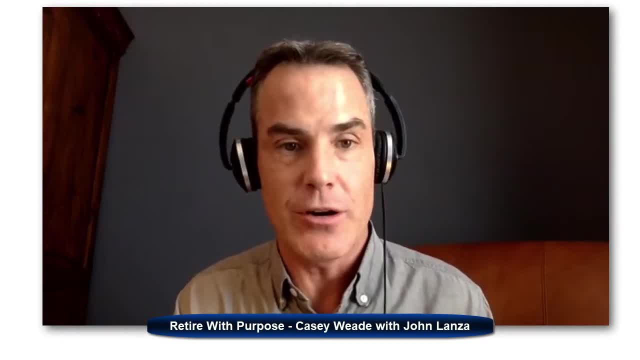 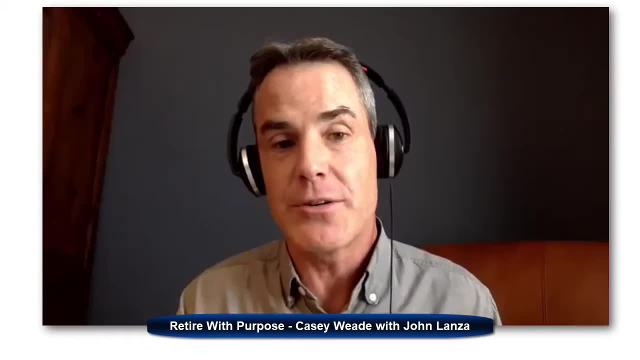 So we read to our kids from a very young age. You know I mean my kid. you know I was reading to her the first week. she can't understand anything. Yeah. But we now know emergent literacy. we now know that the building blocks for literacy 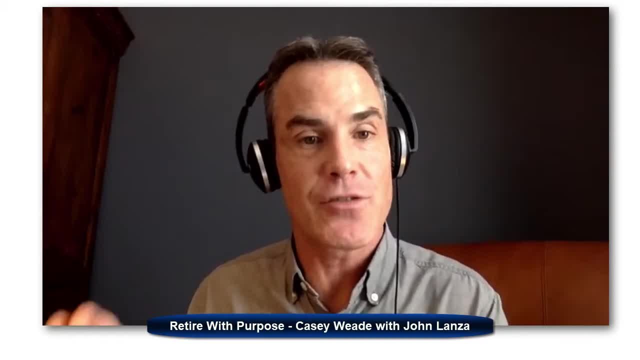 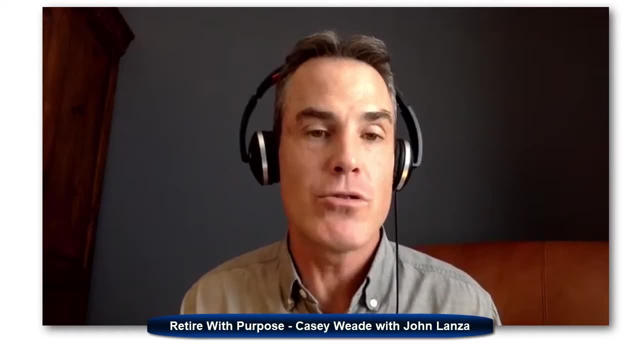 literacy come from exposure to language. the building blocks for later reading and writing come from that. So there's another term in financial literacy. it's called emergent financial literacy. So it's really exposure to these terms. So the sharing and the saving and the spending smart. 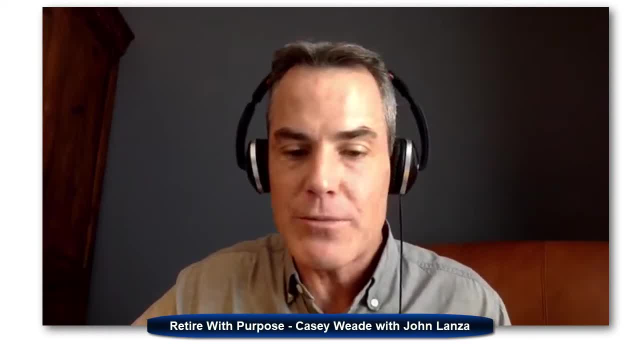 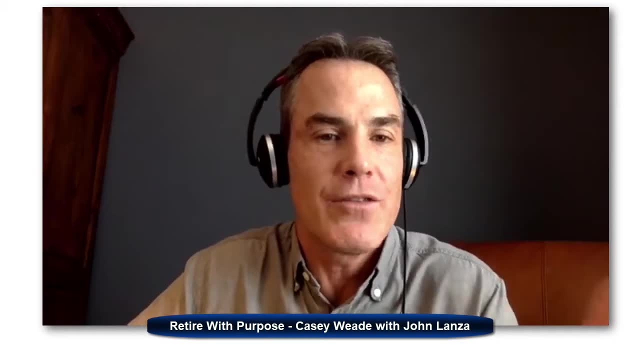 So with regard to money, because I mean I was just having… I just did a podcast with another CFP and he was saying: you know, it's so inherently confusing, I'm sure, to your three-year-old, Like why is a dime smaller than a nickel? 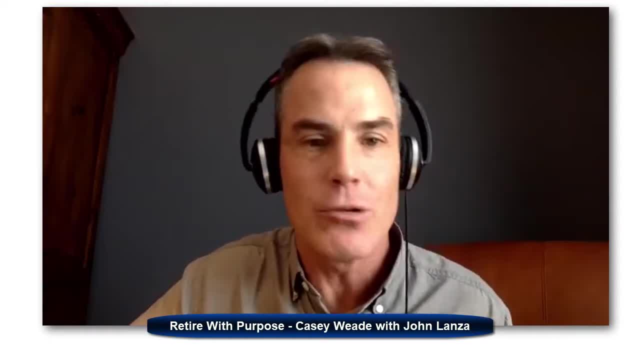 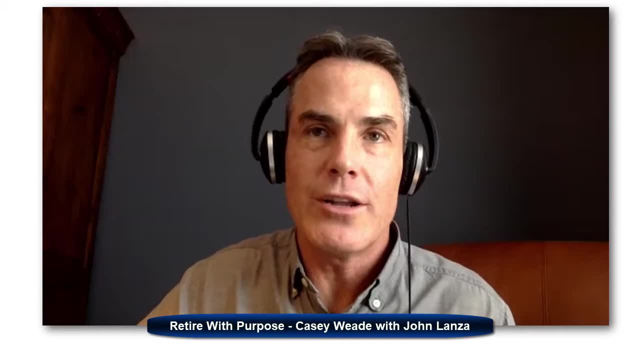 Yeah And worth more. that makes absolutely no sense, right, Right. And so I think, in terms of description of money, it's really you want to…. I don't even think so much, because kids are going to learn how to you know you're. 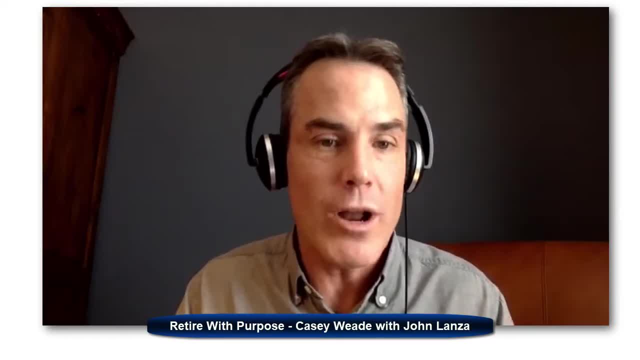 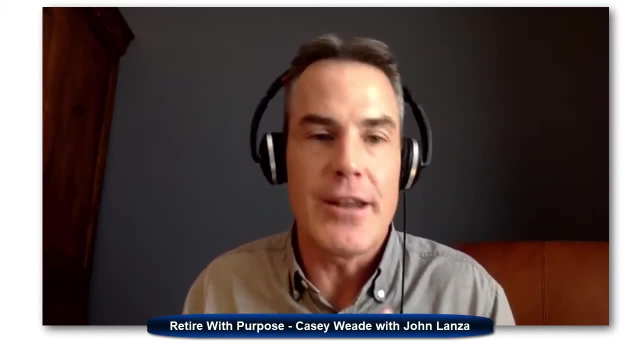 going to have conversations with them. they'll learn it in school what money actually is in terms of the physical. you know thing that they are, you know the colors that they are and the denominations that they are. Those, I think, are less important than really…. 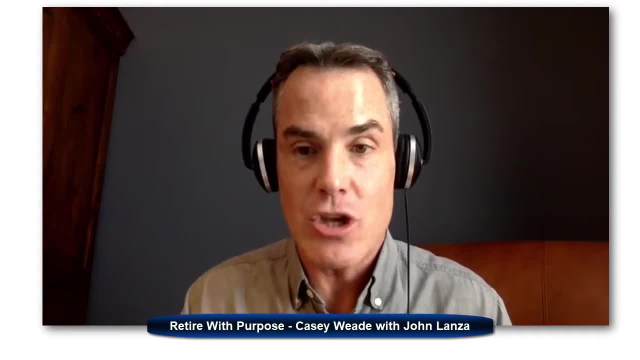 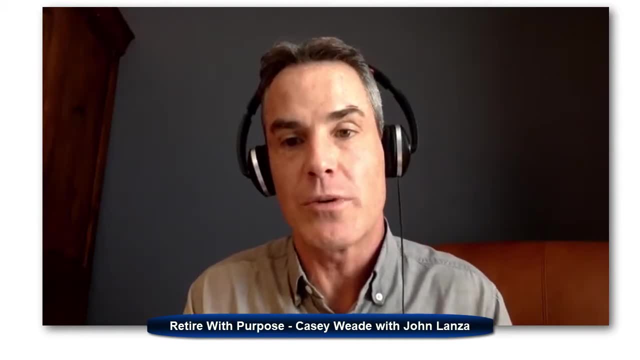 just the understanding how to use money as a tool. So, getting them as soon as you can, getting them to understand that, okay, these things are worth what they are. but what does that mean? What it means is: okay, well, this dollar is going to help you buy this particular thing. 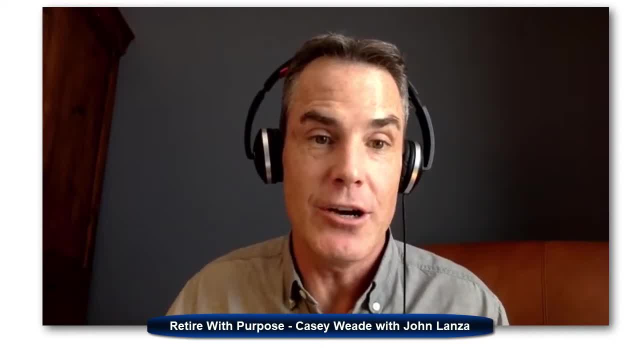 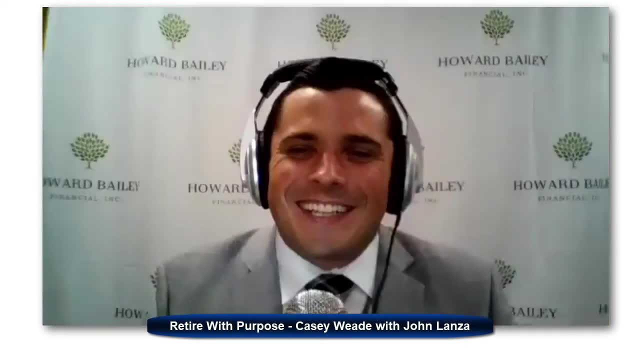 and more of these dollars is going to help you buy a lizard, you know. And even more of those dollars can buy your dad art lessons, so you don't accidentally get a squirrel, Exactly, Yeah, But that's the point. So I think hopefully that kind of answers that question, because one of my pet peeves- 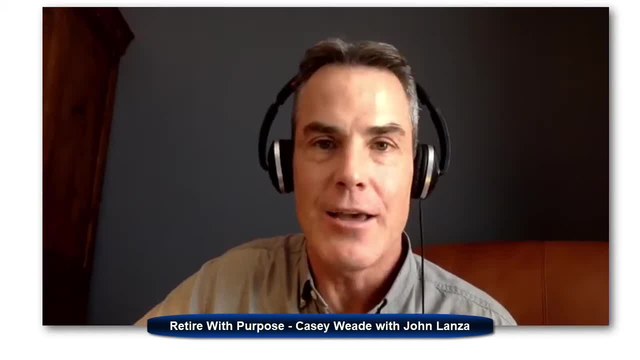 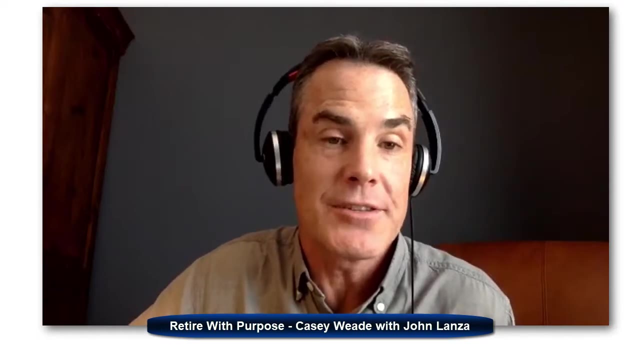 with schools is that we spend so much time in the schools teaching kids about the- you know, the math of money, and almost no time teaching them about any of the philosophy of money, which is another reason that we really have to, as parents, take this on, because it's 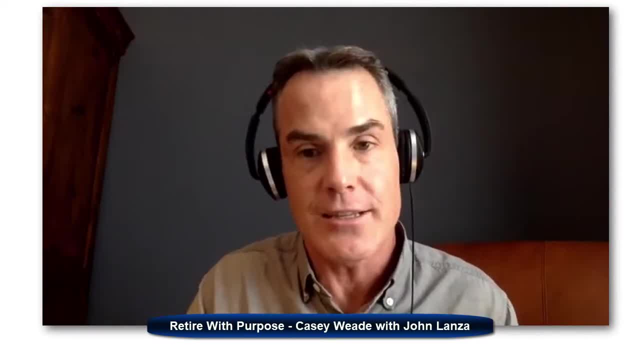 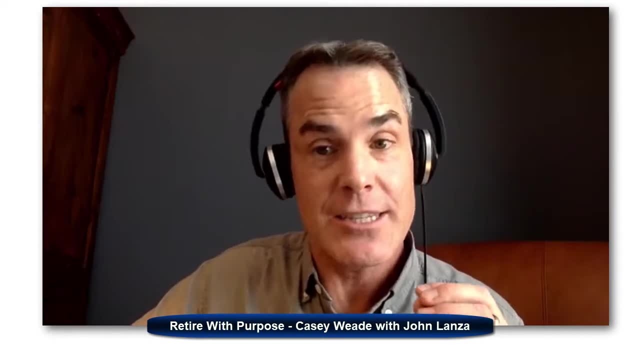 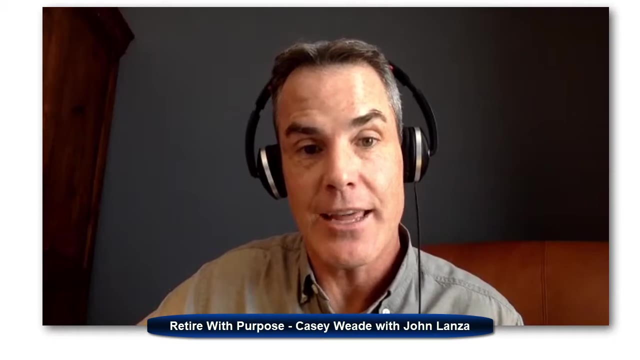 generally not taught in the schools And there are different rules in different states and some schools. some school systems are doing more than other school systems. But even if a school system is teaching financial literacy itself, the only way a kid is going to learn to become money smart is with money. 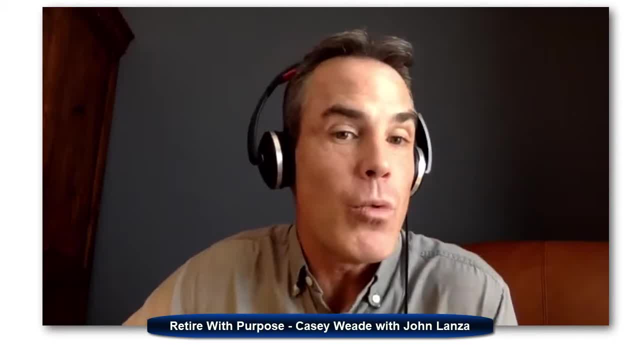 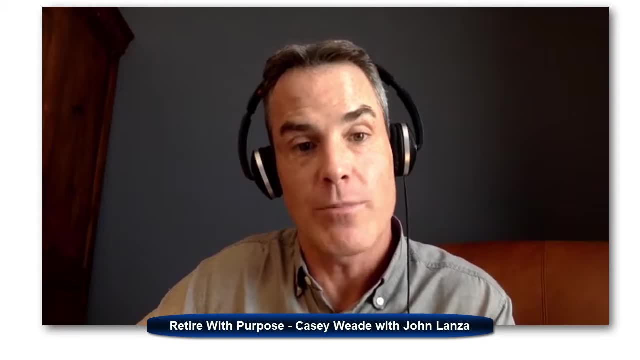 They have to practice with money, And so that's why, as a parent, you want to take on this role of being a person who's providing an allowance, and with a purpose, a why behind it. That why behind it is to teach them the basics. 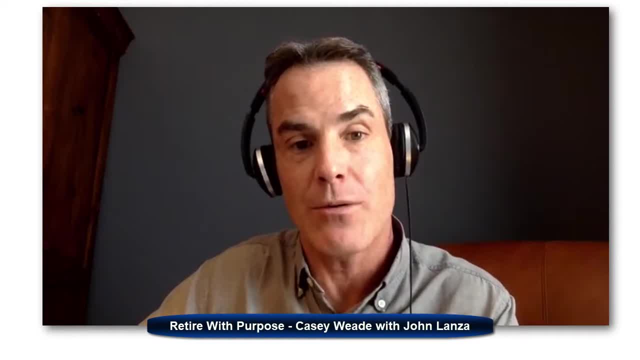 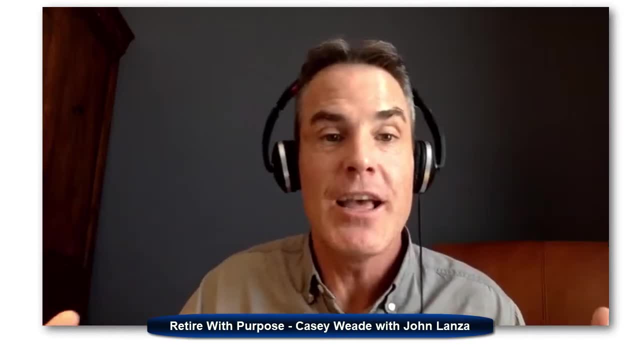 So money to understand, to use money as a tool, how it can be used, and then to teach them about the sharing and the saving and the spending smart, and then I keep harping on those basics. But the reason I harp on those basics is kind of goes back to what we talked about in the 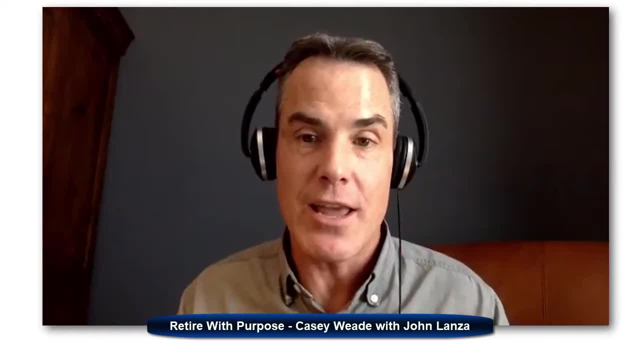 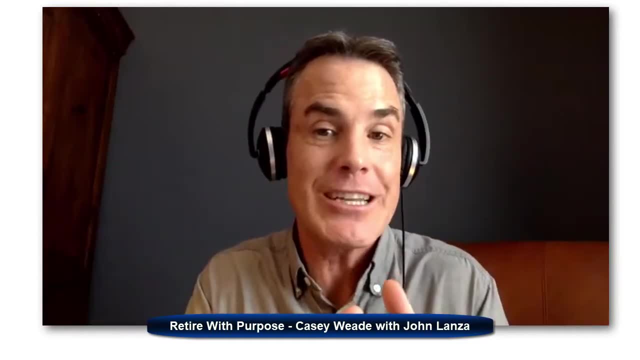 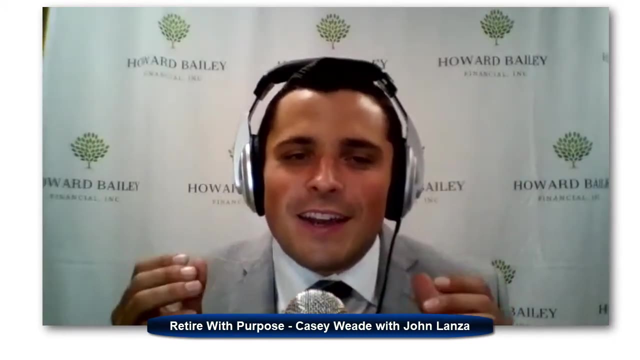 beginning, which is that money can be so intimidating because there's so much complexity around it, But it doesn't need to be intimidating, particularly for kids, because you can simplify everything down to the basics, Absolutely, Yeah. So one of the quotes from your book you had said, and this quote just really struck. 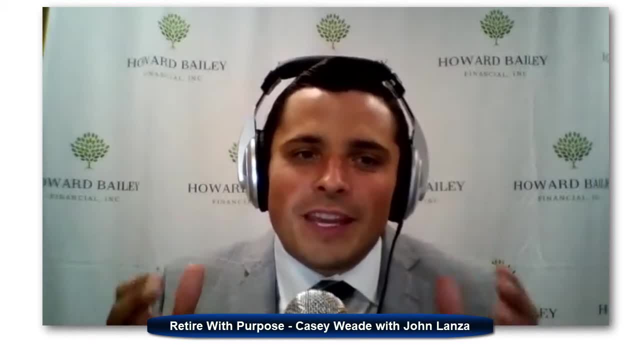 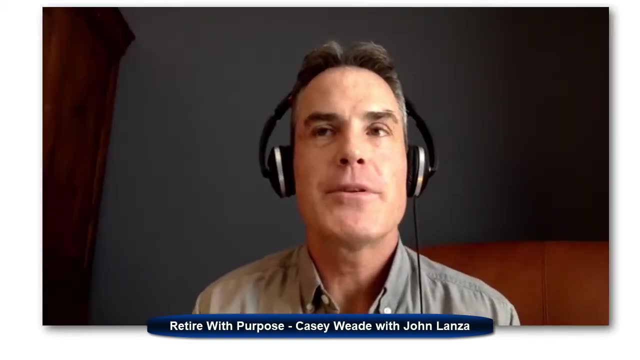 me. It said: a money-empowered person knows money as a tool and uses it to craft a meaningful life. What does that mean to you? Well, yeah, The purpose behind that statement was that I don't want people to get caught up in this. 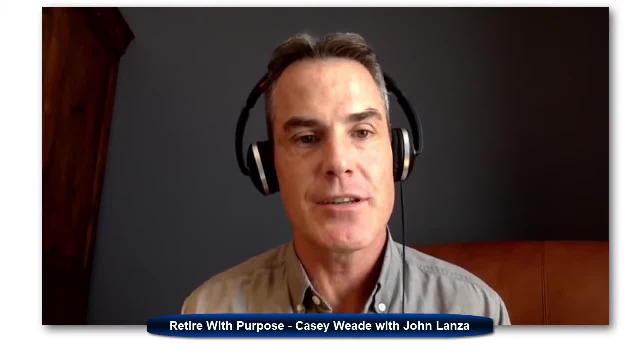 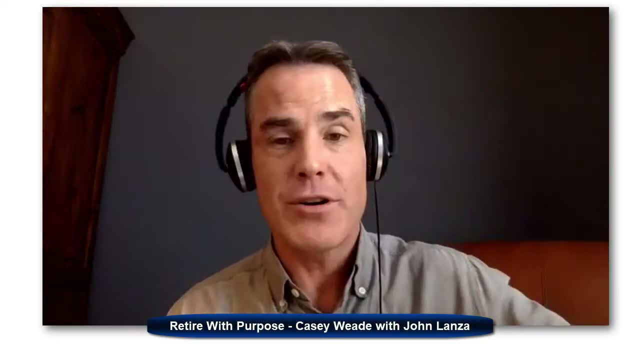 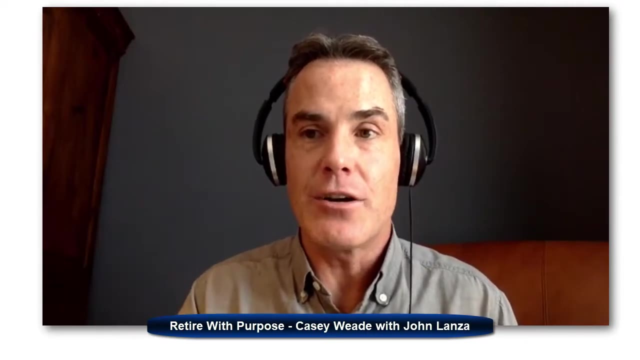 isn't about. wealth is different for different people, So this isn't about amassing any particular amount of money, And one person is going to have a different definition of wealth than another person. But the key here is that both those people- whoever those people are- they have to achieve. 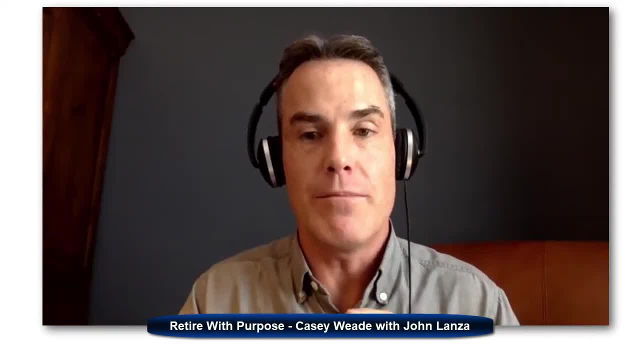 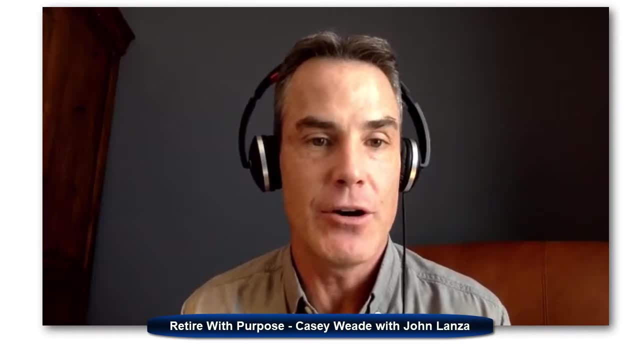 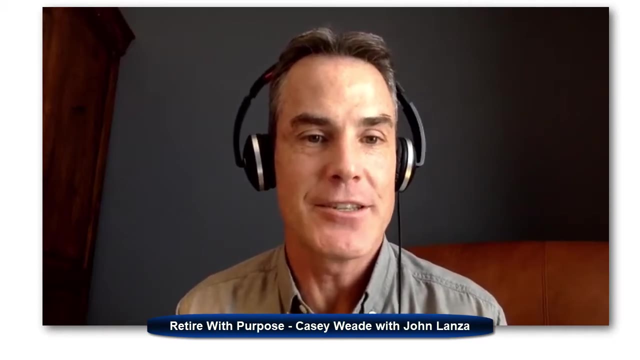 that money, empowerment, where money is doing for them what makes meaning. We're all ultimately here to live a meaningful life. Yeah Yeah, There's a great book that Viktor Frankl wrote- I don't know if you've read that- called The Search for Man's Search for Meaning. 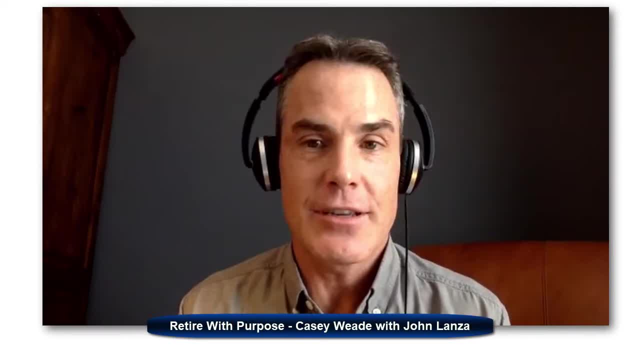 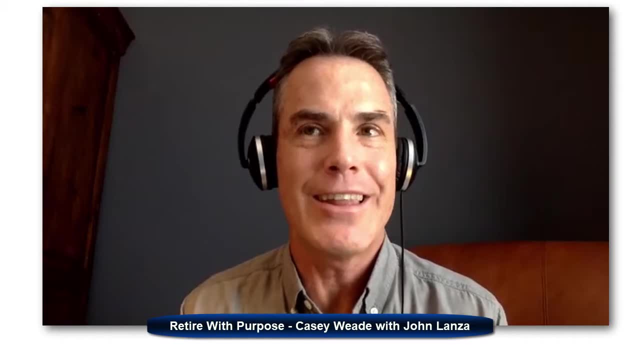 And it really does get at. I mean, his obvious thesis is that that's why we're here. We're here trying to figure out, kind of what it's all about, but really more than that, what we are doing here. What is our purpose? 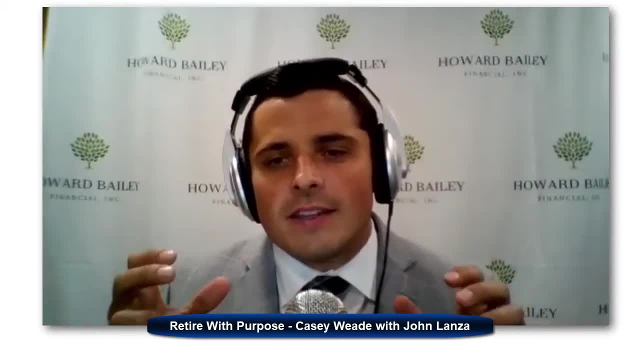 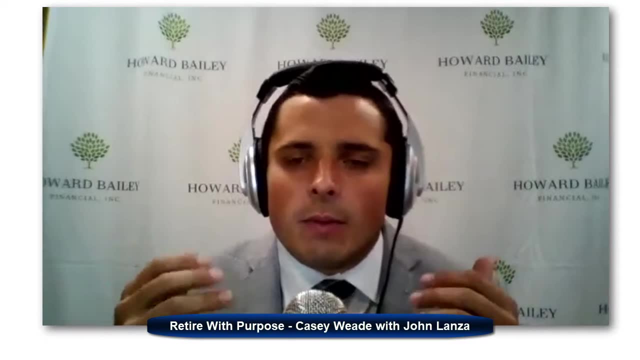 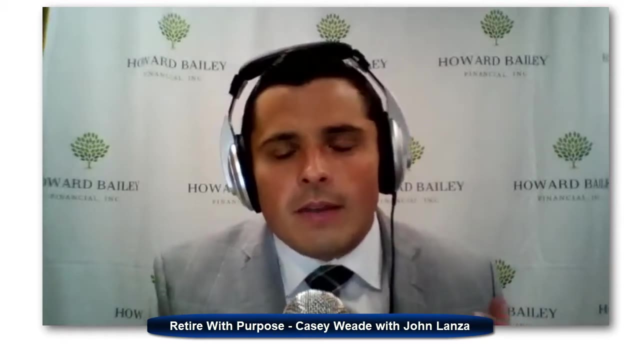 Well, I wonder how we lose touch with that over time. Yeah, You know, I'm meeting with individuals that are in their 50s to 60s, either preparing for retirement or already retired, And it's gotten to a point where the conversation for me, I want to start at the purpose. 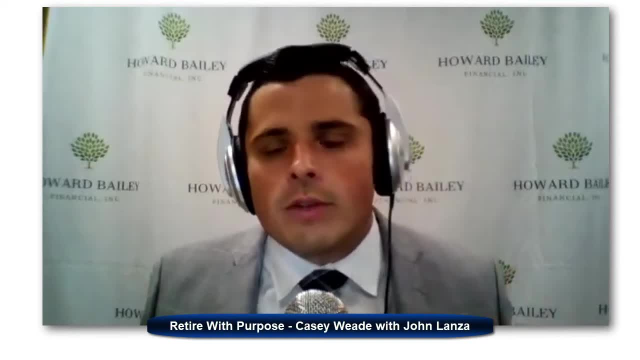 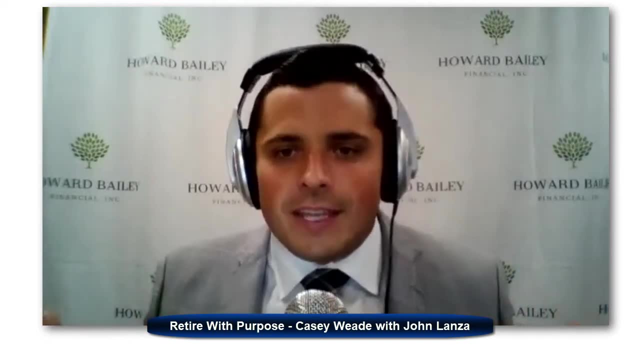 What do you want these dollars to accomplish for you during retirement? What is your retirement all about? What does retirement mean to you? And let's use these dollars as tools in order to defend against that purpose At all costs, and defend that at all costs against the major risks we're going to face. 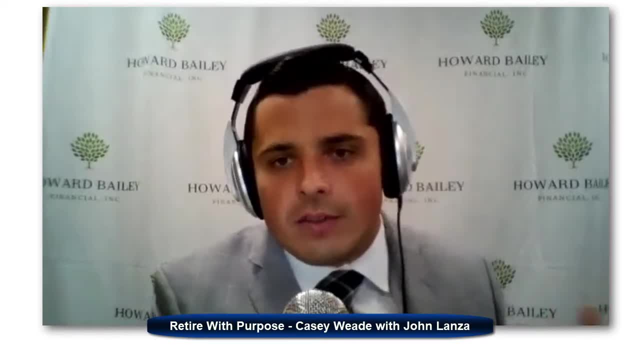 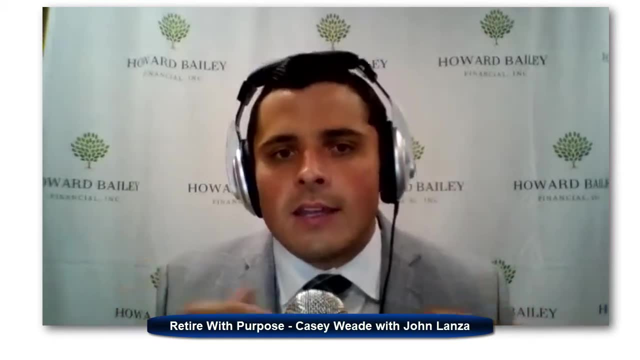 and then work our way into the tools and work our way into the individual investments or the products or services that need to be used in order to ensure that we're protecting that And, over time, it seems like we've been conditioned that it's about the product. 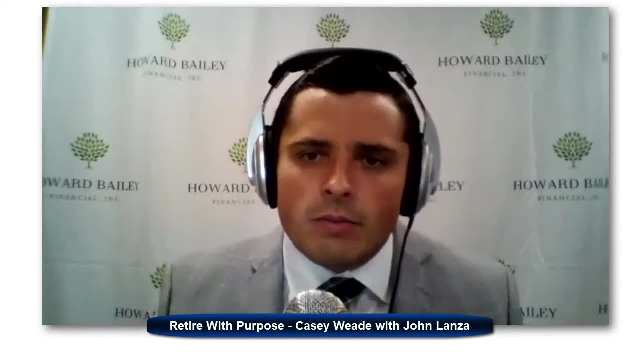 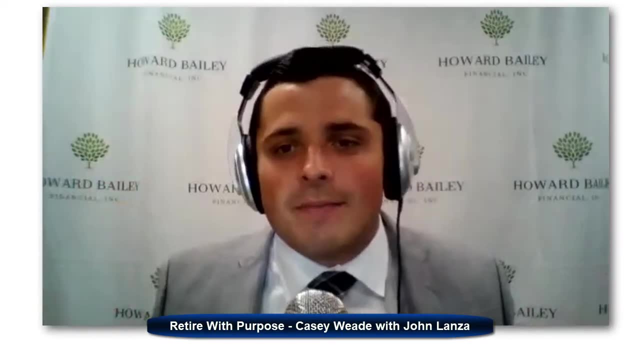 It's about the investment: What's going to get me the biggest rate of return? And I want to talk about stocks, I want to talk about ETFs, I want to talk about mutual funds And, in the end, it's not about that. 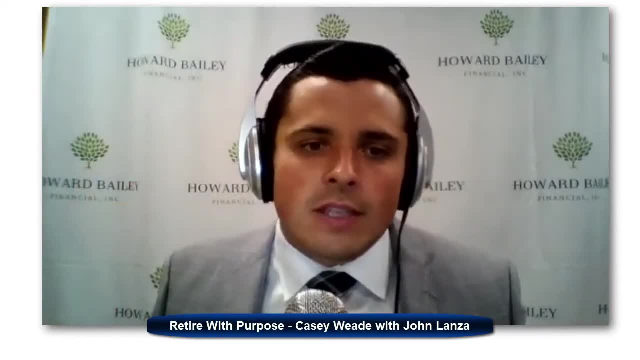 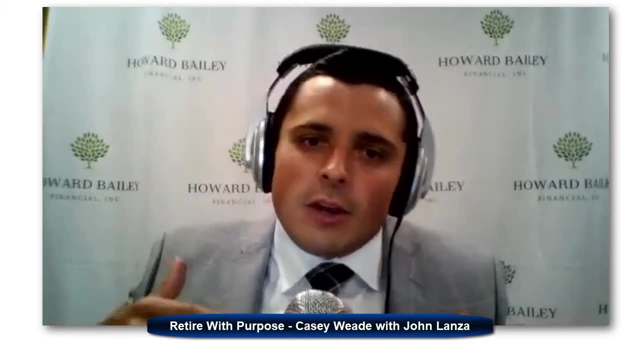 It's not about the tool. We might say, for instance, I hate the stock market. Well why? It may be the best tool to help you keep up with inflation over the next 20 or 30 years as you're in retirement. 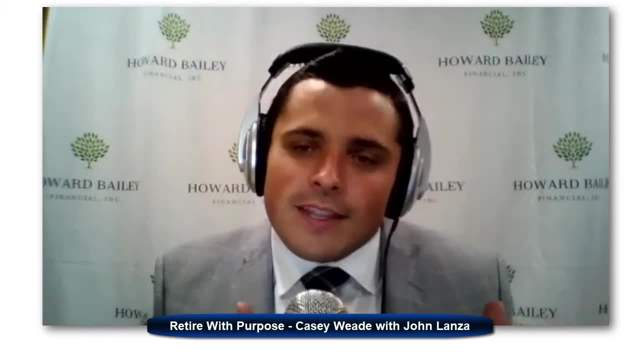 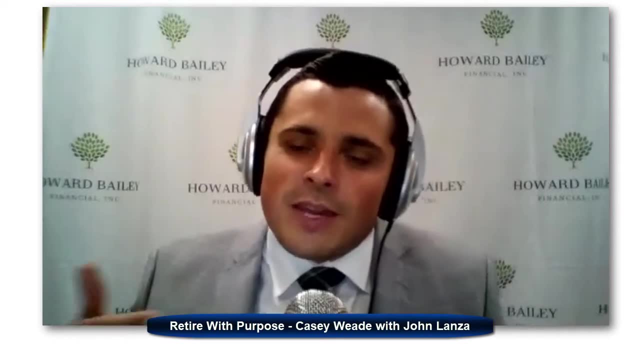 Or we might say: I hate annuities. Well, that's okay, but that is the only vehicle that's going to give you a guaranteed income that you can outlive. And if you had a guaranteed income and you had inflation protection, you're going to 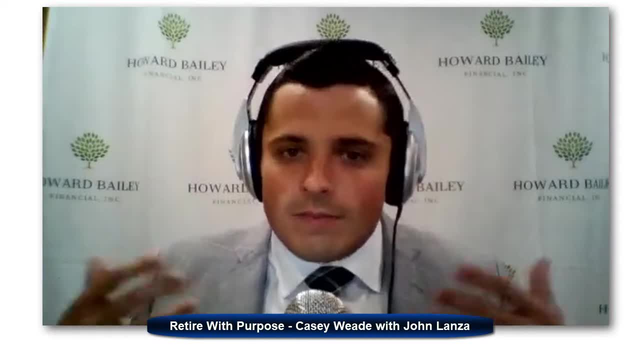 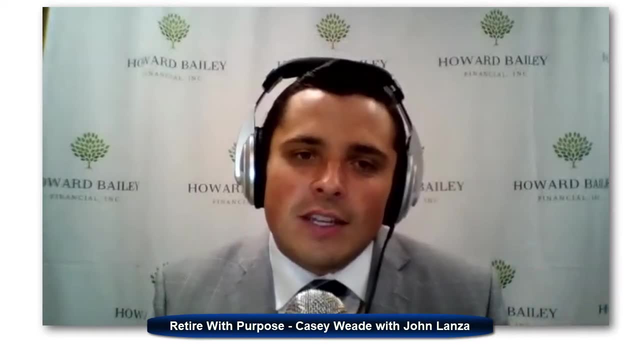 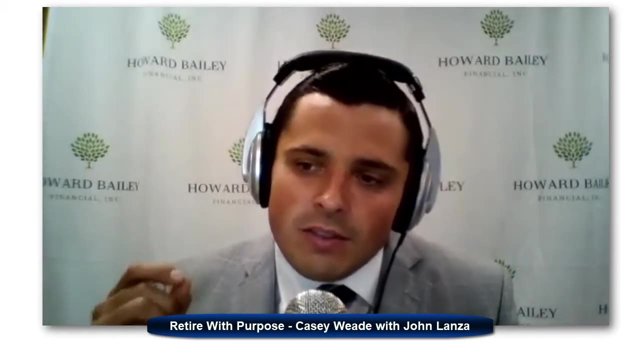 have inflation protection, and we did it with the most efficient tools. now you're living your purpose. I just wonder how we, over time we must just get conditioned to forget that money is a tool to create a meaningful life and we just start thinking about the money all the time. 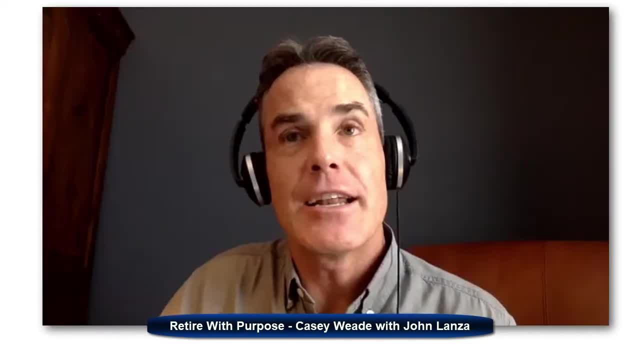 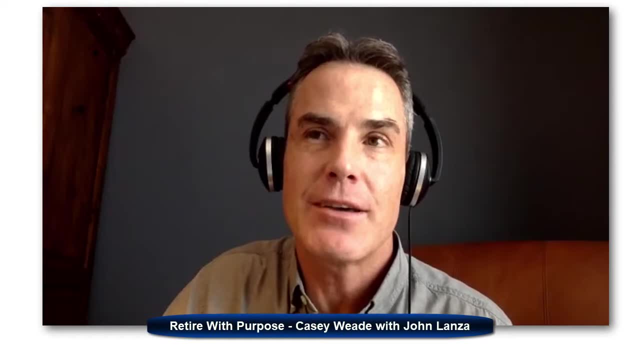 and not what it's creating in our lives? Yeah, And it's a great question. I don't have the answer to that, But I put a…. I think about it a lot Because I… One of the things I want to get across to kids- and when I talk about products, I'm 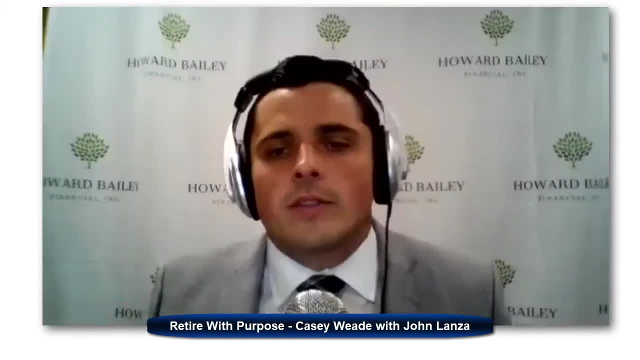 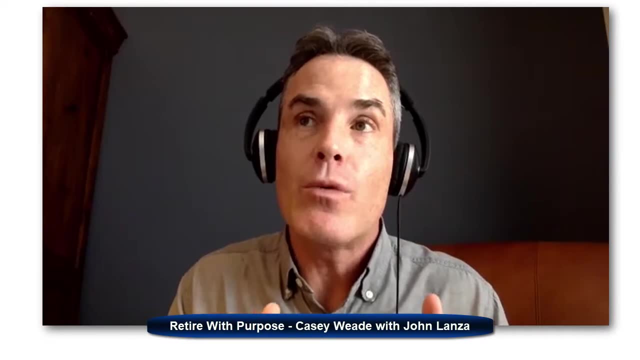 talking less about the financial products, but actual things that you purchase. You purchase, And I think one of the…. But what you brought up is just as relevant, What I really want them to understand, and they're not at this point of understanding. 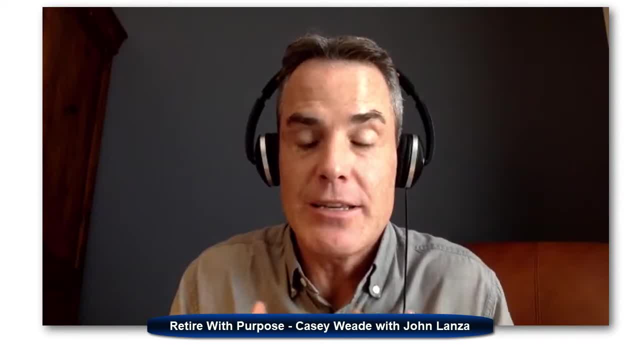 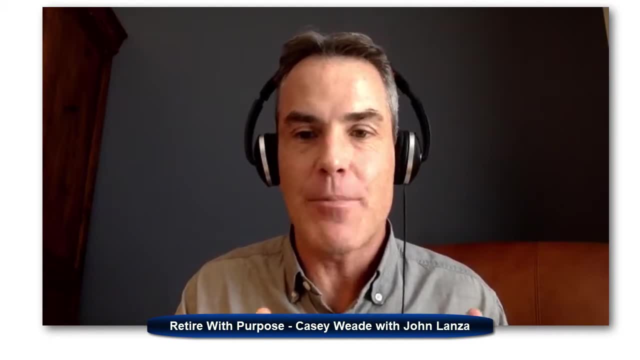 yet- and this has been a process for me- is that I feel like a somewhat reformed spender, in the sense that I still… Like, for example… For example, I'm a runner, so I have a watch and I want to upgrade my watch for…. 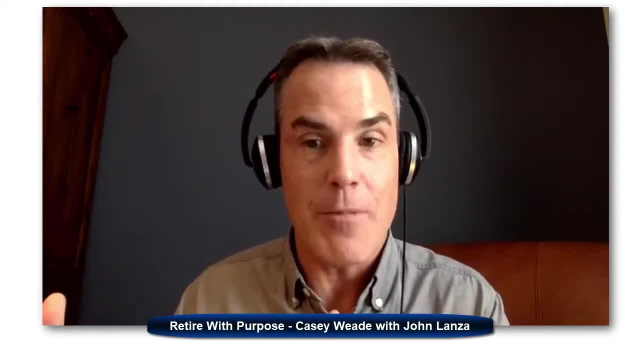 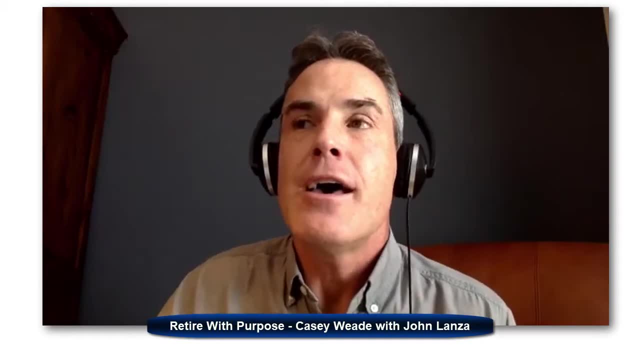 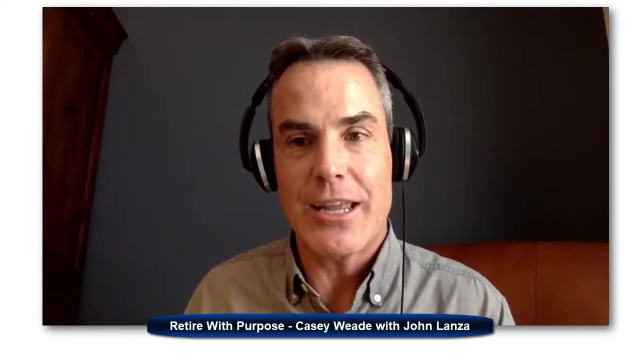 I want to upgrade the watch because I want to get a certain type of map on the watch And so there's a practical side to it, and then I'll sell the current running watch that I have right now. But I realized in my research that I'm not so sure that what I'm trying to accomplish. 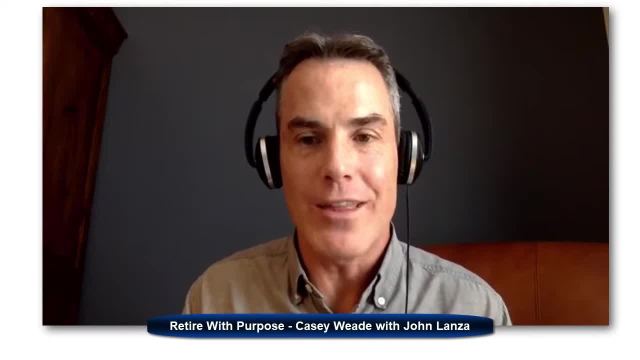 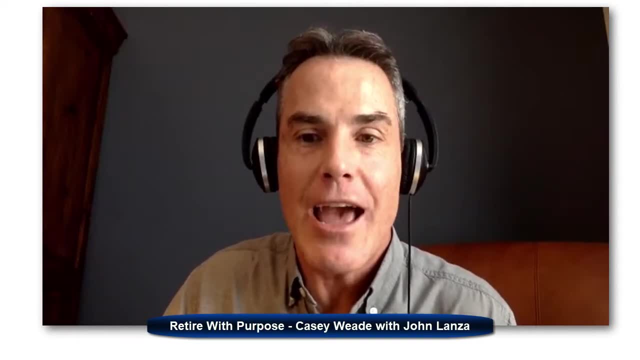 getting the map on the watch is really going to work for me the way that I want it to work. But then I realize… I'm feeling like, oh, I really want that watch, But like… And it's only having been around for…. 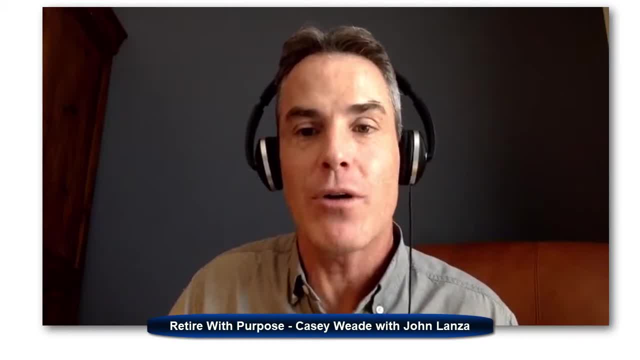 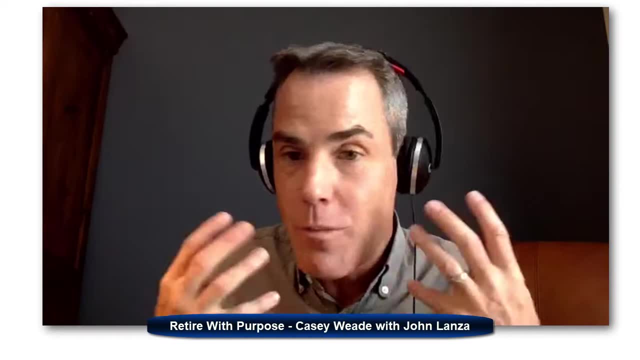 Having gone through so many purchases that I realized that I do not want to make that purchase for any other reason than the practical reason, because the excitement… Because I get the same dopamine rush from a new product that everybody else does. We all do. So it's important for us to recognize that. 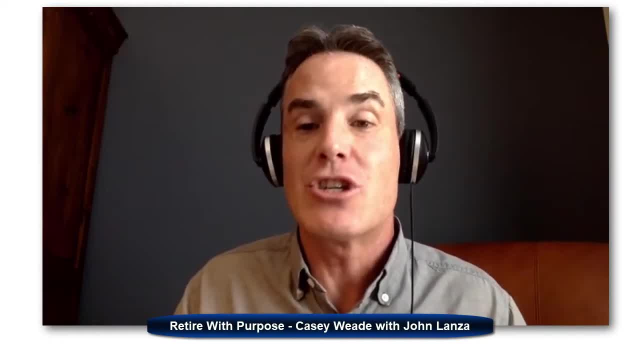 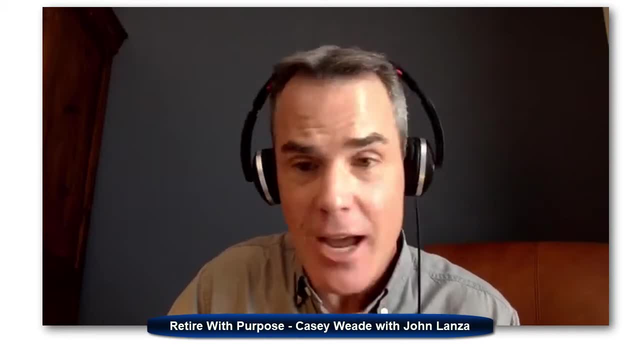 And it is just like… It works just like a drug, but it's just like a drug: The effect is fleeting. And so my point here is really: I want my kids to understand. So every time they get something and they get excited about it, or you know, for example, 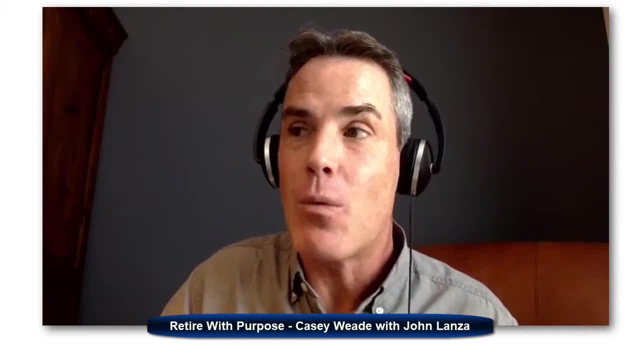 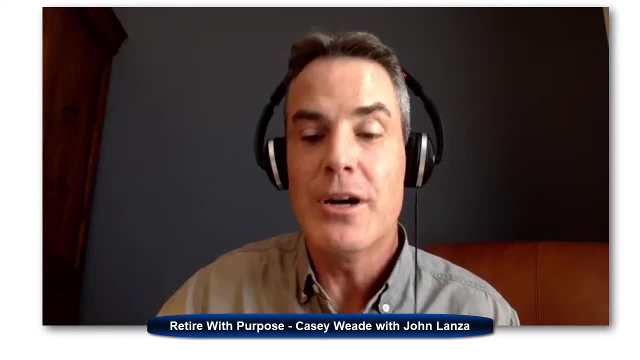 my younger daughter wants to get a new phone for her birthday and I… One of the points I will make- and it's not necessarily that it's going to change what her approach is or what she wants to do- is the excitement you get from that purchase. 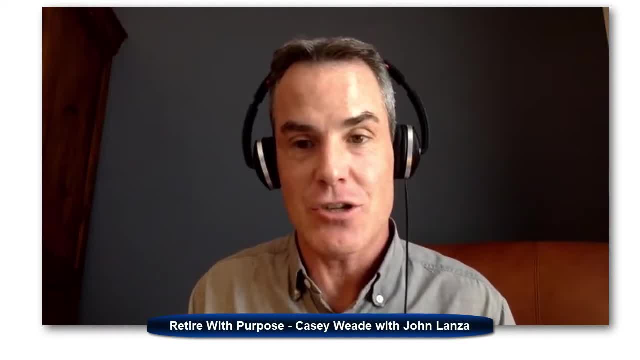 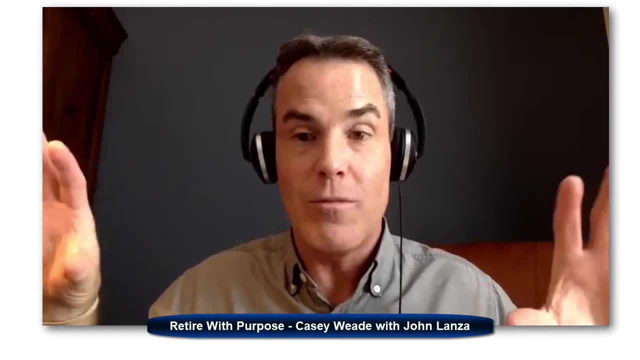 is going to be fleeting, And because what happens is- and this is described in a terrific book called Stumbling on Happiness- it's just like when you get a new car. So if you look at people who have bought a new car versus people who are driving their, old beat-up cars. there's no happiness increase from driving the new car over the old car And the reason is that when you get your really nice car, that now you're not comparing that car to your old car after about you know, two weeks or a month or whatever it is. 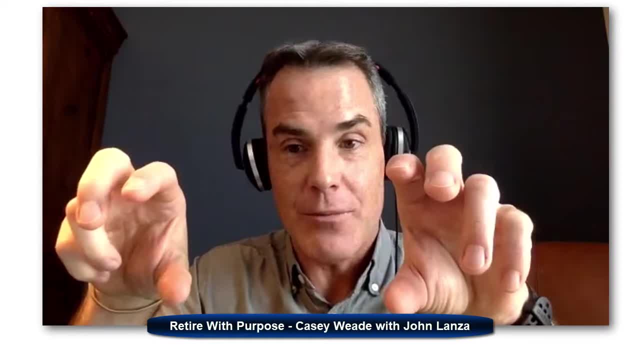 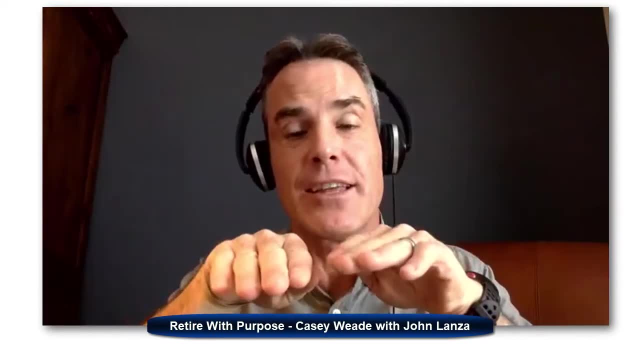 You're comparing that car today to that car yesterday, And when you're stuck in traffic, it's the same feeling. There's nothing… There's no better… You, basically you, habitualized to that car and I'm using car as an example. the point: 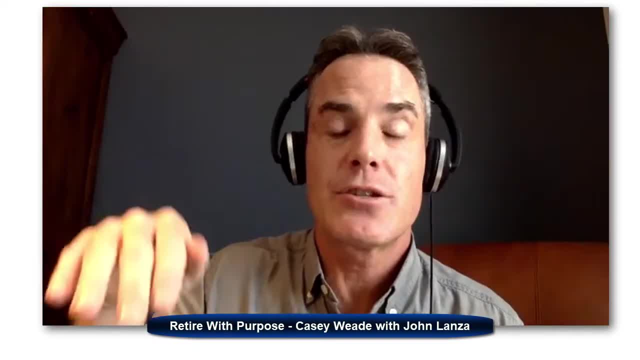 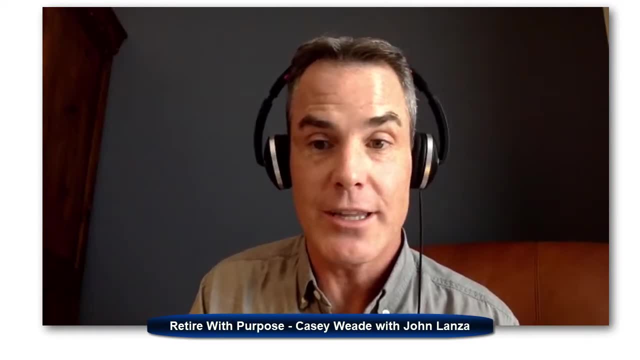 is really any kind of purchase, And so- and this gets to your point about meaning- is nothing that we do with the money in terms of purchasing these things is going to lead us anywhere, towards our? you know, I like to look at it as we're kind of going towards the mountain, which is a term that 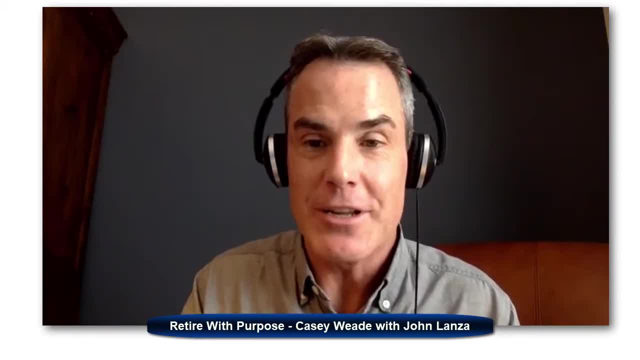 I heard from a guy named Neil Gaiman, who's a writer. He's like… He's a great writer. He's a great writer. Neil Gaiman said: you know, if I can't see the mountain, how can I see the sky? 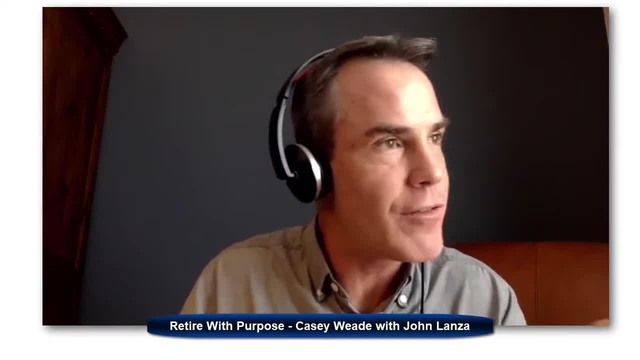 But if I can see the sky, how can I see the mountain? And every time I feel like I'm kind of going off. he was talking about his mission, his purpose in life, And every time I feel like I'm kind of walking off towards somewhere where I can't see the 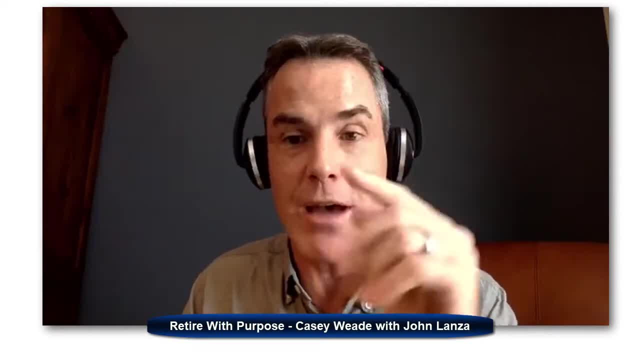 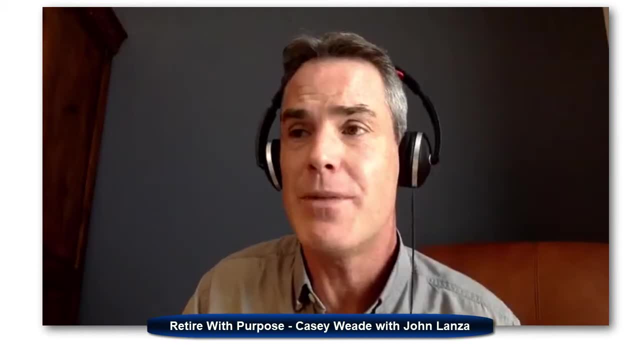 mountain, I know I have to stop, turn around, focus and look at the mountain, And that's how I feel. that same way if I get caught up in a purchase and I'm like, oh, I really would like whatever you know, that watch or whatever it might be. 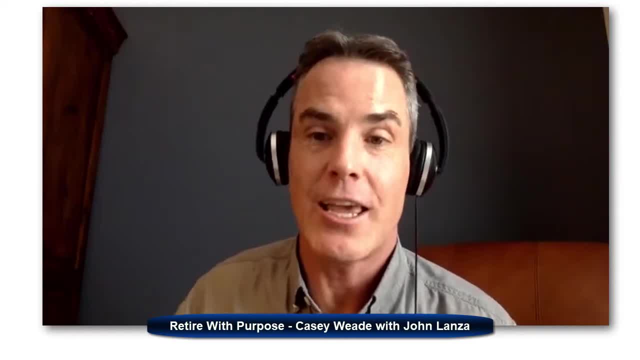 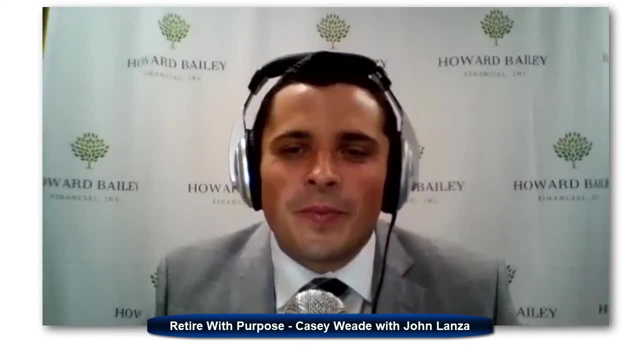 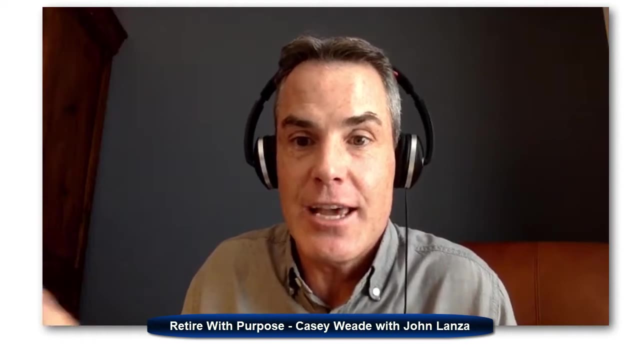 You just have to take a breath, And a good, practical way of taking a breath- and we've instituted this- is this waiting period. So if you want to buy something, as a kid starts to amass more money, for example, in their spend smart jar, they could suddenly be able to purchase something for $100, and it's not something that they've been saving for. 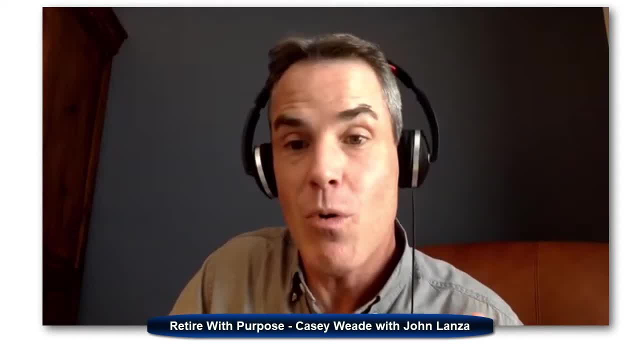 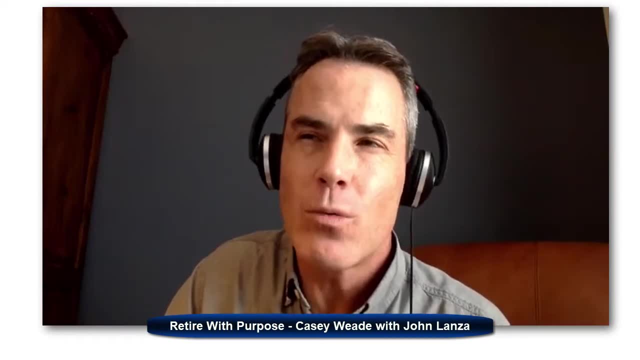 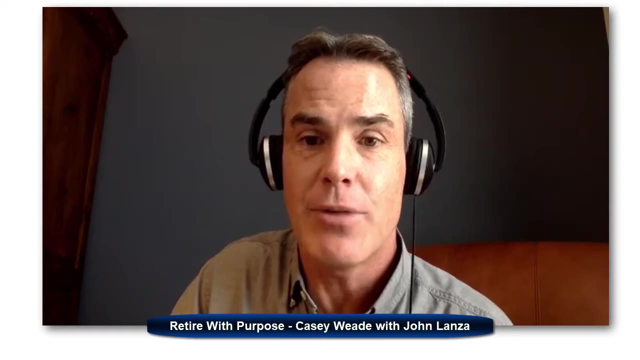 But if we institute something where if it's $50 or more they have to wait a week, And if it's $100 or more they have to wait two weeks before they get it, And it's a way of – it doesn't mean that they're not going to get it, but it means that at least they've put some thought into the purchase and it's not an impulse purchase. 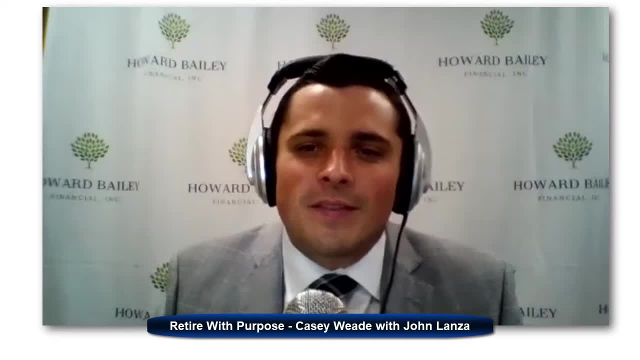 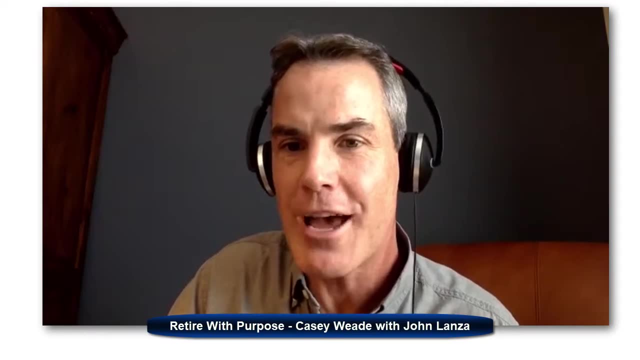 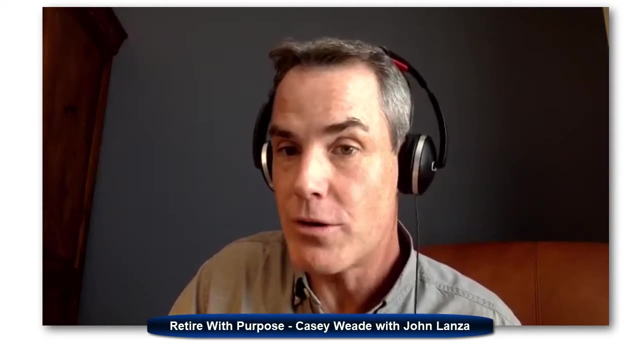 It still might be an impulse purchase, but it's a little less of an impulse purchase And it's again not to say – if your kid does this and they purchase something that you don't agree with after that purpose, after the time has elapsed, don't feel like you have missed the boat or that your kid is a profligate spender and there's nothing you can do. 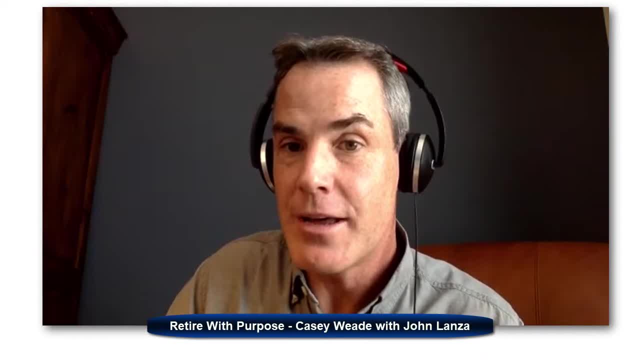 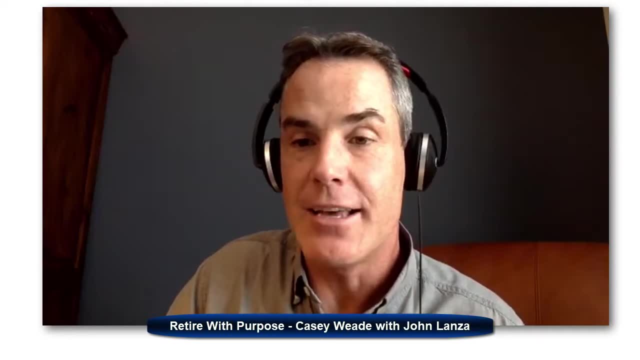 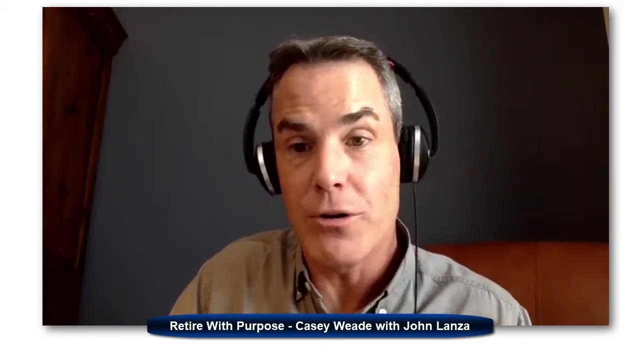 Okay, Because you've gotten a message across to them that they now have a reference point for thinking about as they get older. And these are all reference points And, as a friend of mine and a guy also involved in financial literacy, a guy, Bill Dwight, said – because he's got kids that are now older. 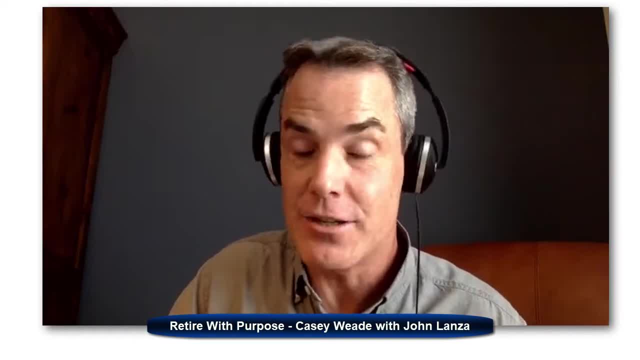 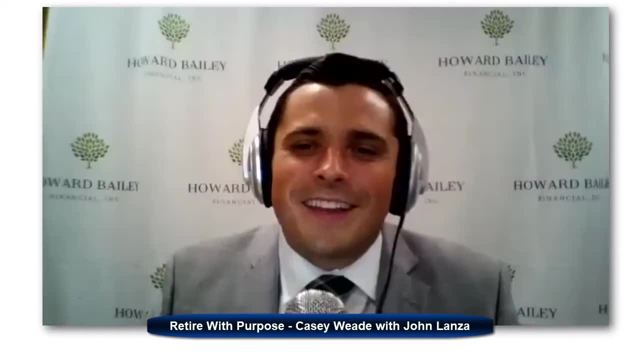 He's now a grandfather. He said they're listening, They are paying attention and they're certainly watching, And the messages do get through. So stick with the messages. Well, I think you're helping Children create meaning out of the purpose, out of the purchase. 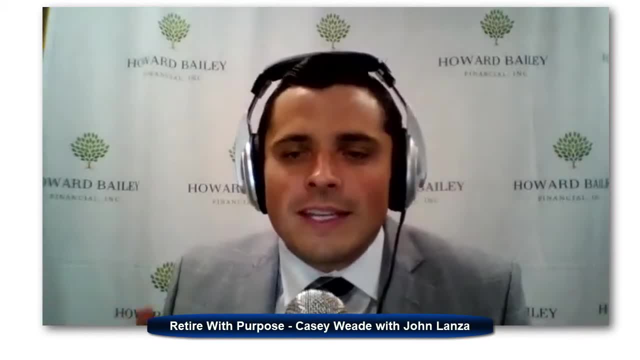 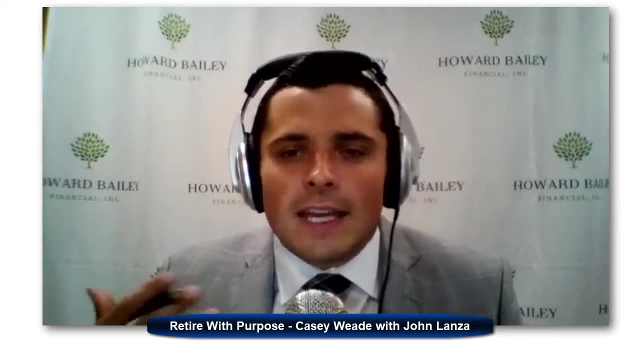 Is this a meaningful purchase And then we can ultimately make the decision? I was wondering as I read that part in The Art of Allowance. we've got a three-and-a-half-year-old. He's got his spend jar Last night. we're getting ready to go to a market with a little concert and food trucks. 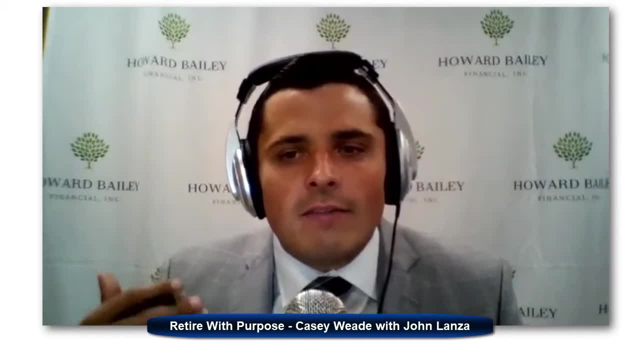 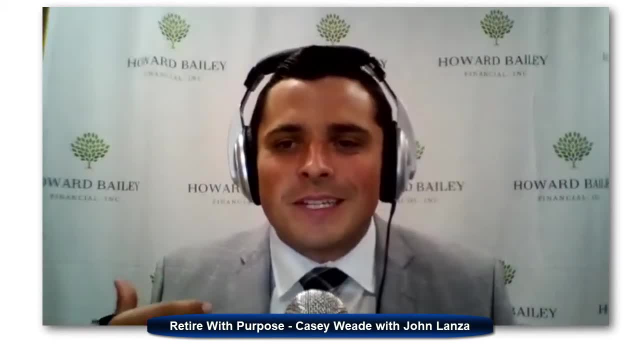 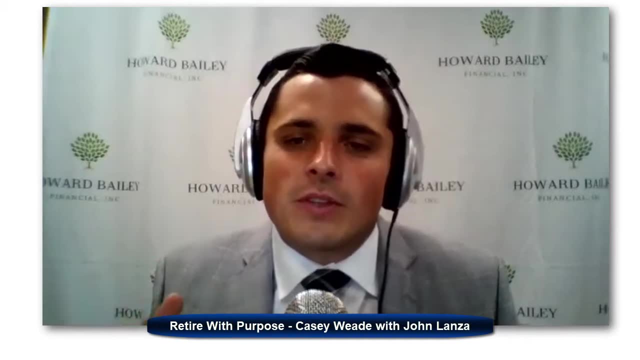 Right, Right, Right, Right, Right Right. When we get there, there's probably going to be the opportunity for him to buy some ice cream or buy a soda, And so I said, well, maybe we should just fill up his wallet full of the spend money. 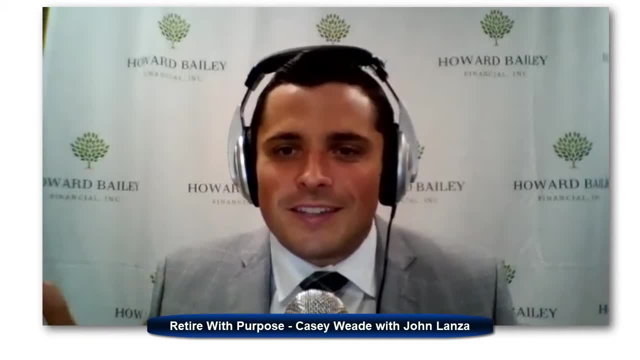 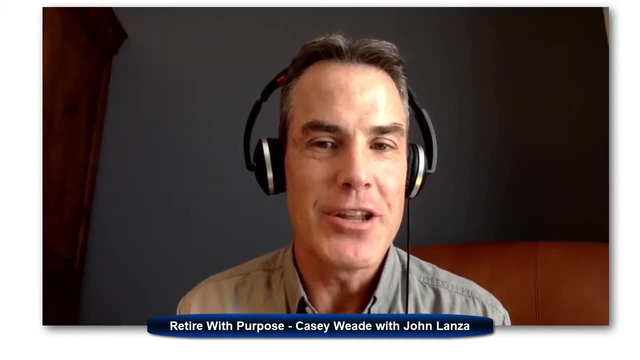 And then when we get there, then we can have this conversation and determine if he should be spending it or not. Does that make sense? Yeah, it does. And because you're introducing him to this kind of opportunity cost and the scarcity of money because he's going to get to a fair and be like I want it. 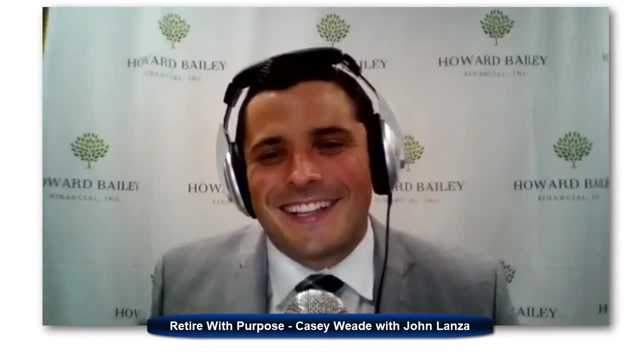 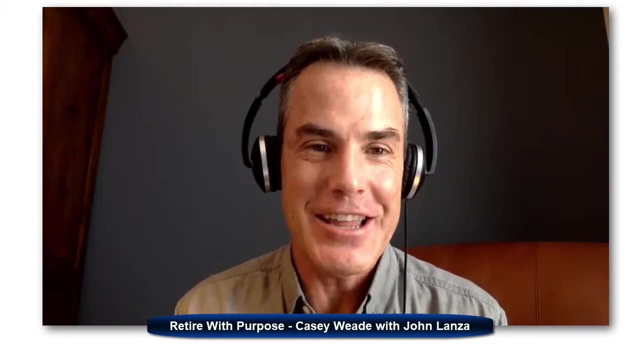 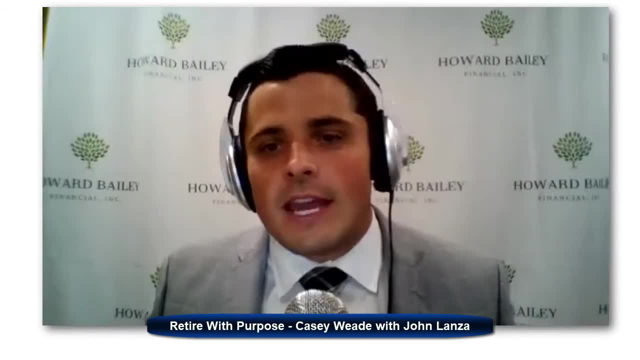 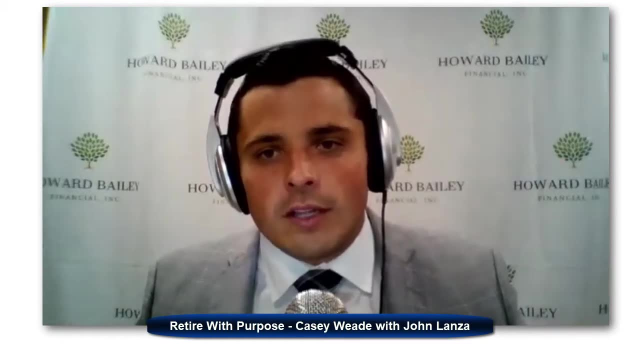 for those things where we'll be at the counter at the grocery store and he'll say: I want that. He'll want a piece of gum or he'll want a candy bar. and I'll say, did you bring your wallet? And he looks at me and goes no. 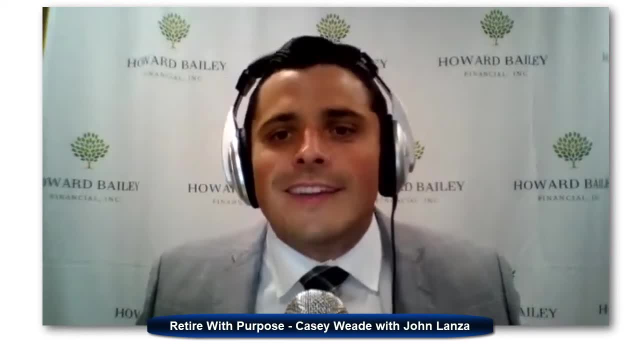 And I say: well then, And then next time you bring it you can buy it. And it goes so smooth. He gets it. He's like: well, I don't have my wallet, So I can't buy it. 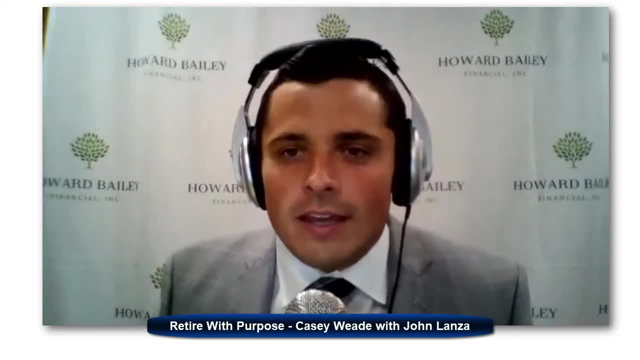 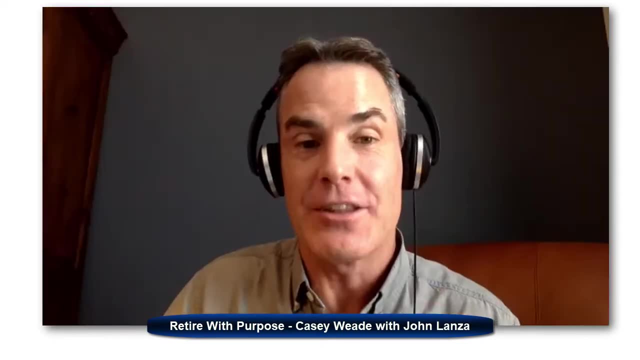 Now I have heard recently he'll say: well, don't you have your wallet, dad? Yeah, but that's my wallet, That's my wallet. Well, this is – and you're getting at the key point, which is – and this works. 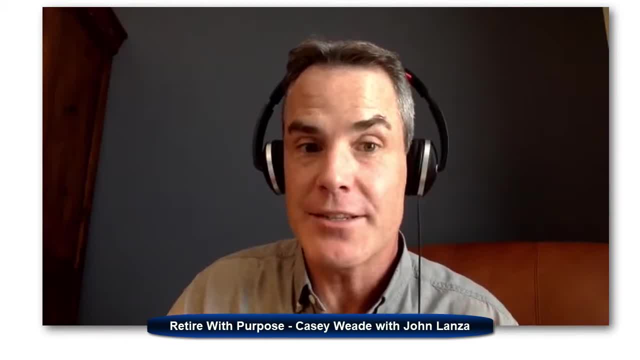 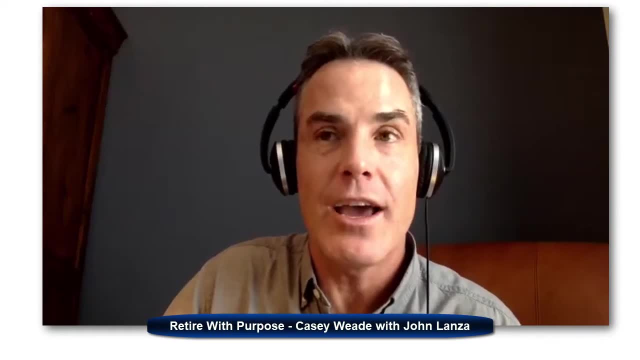 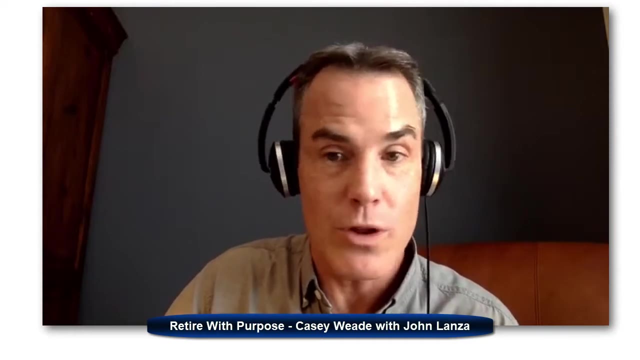 out well here, because you didn't necessarily have to say no, Like he realized – Exactly, I didn't just have to say no, There was reasoning behind it. Yeah, And this is why all this really pays off, is that? – because in some cases, with my kids, there was a tantrum or two when we went to the store and we wouldn't buy them something that we would have bought them before they had their allowance right, And so we had to kind of go through that tantrum. Once they go through one or two of those, you're pretty much done with the tantrums. for that, because they realize you're not going to cave and you've already established that with them, with your son, And that's – it's a wonderful thing. And the other great – the other real positive here is that they start – they treat their 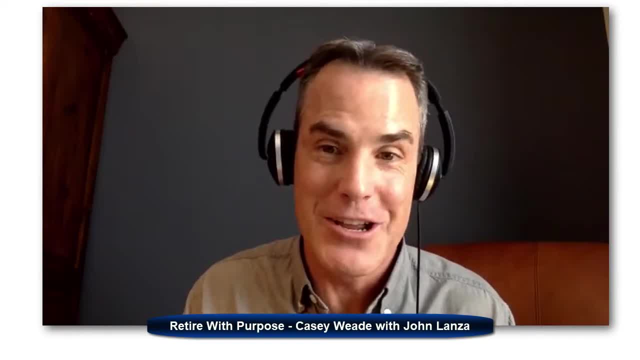 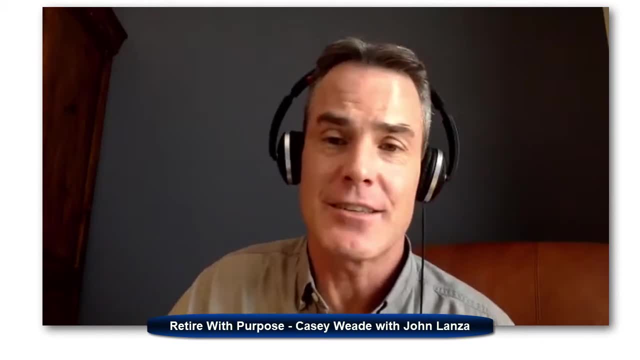 money like it's gold versus your money, which they – and they really think about their decisions I still –. even my 15-year-old is constantly negotiating with me. He's like: I want to go to Jersey, Mike's, Will you pay for it for lunch for me? 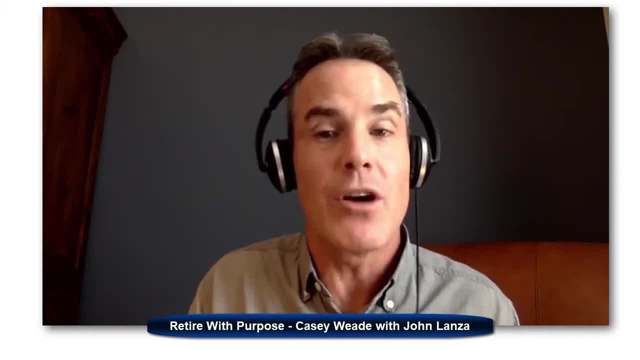 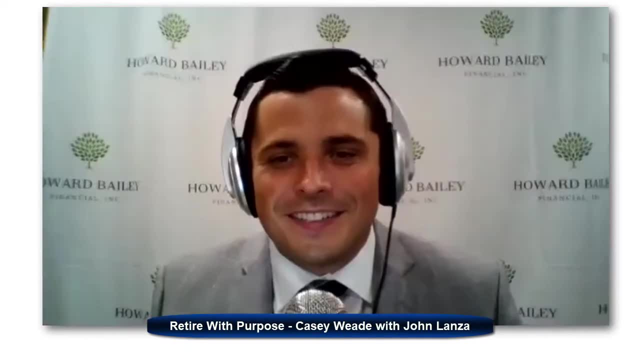 Because I didn't –, we didn't – so yeah, Yeah, Yeah, Yeah. So the way that our food works is that they typically – we will buy the food that they can make for lunch right? So if they play their game right, they don't have to be spending much money on it. and then 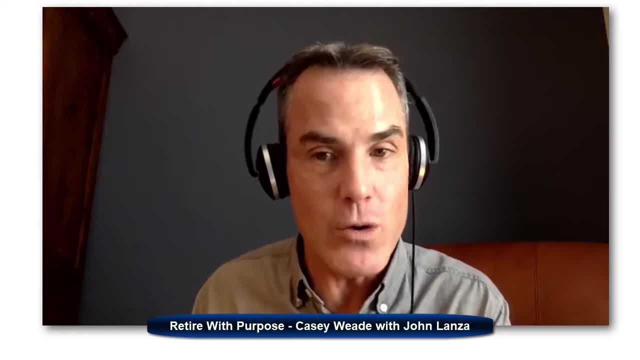 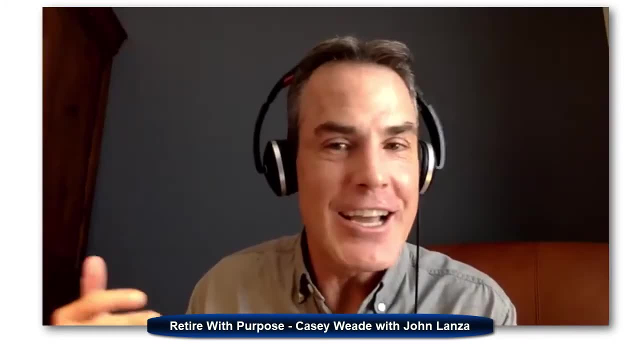 they can use – the money that they've budgeted for food is the food that they get out, right? Well, I think – yeah, Go ahead, Oh, so – but there's still – it doesn't mean that there's not a back, and 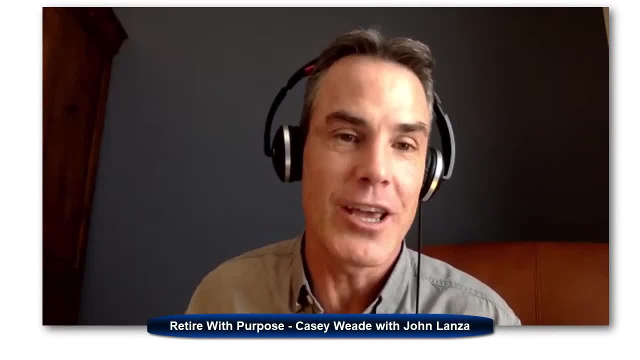 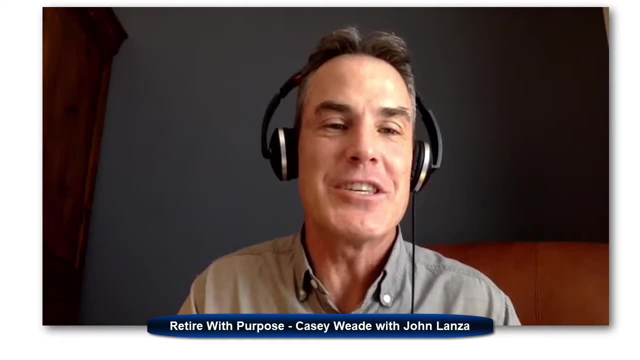 forth and yesterday I told her. I said you know what? Yes, You can get the Jersey, Mike's, because I forgot to get the food. You can get the food that you asked me to get, that you would bring. It was easier to say yes in this case and it was a one-time only thing and again, that's. 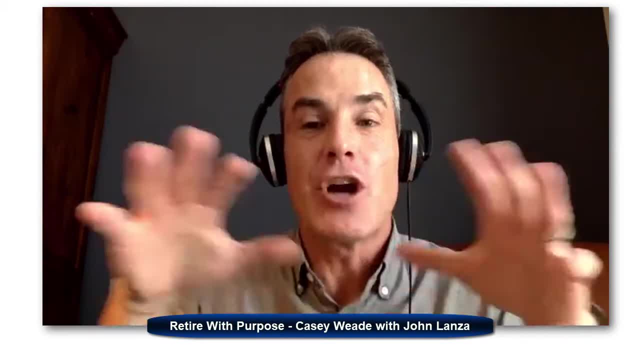 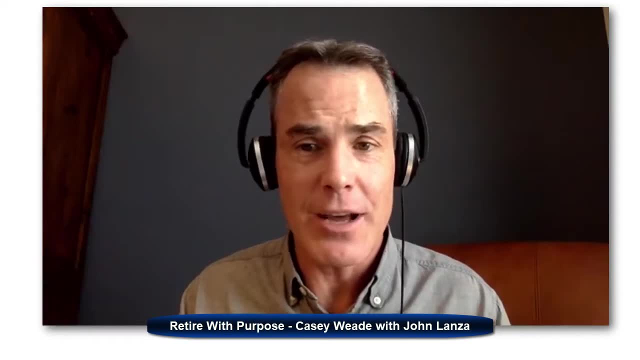 why like these – that's why the – it is an art. There's an art to the allowance, because you can make decisions like that and just say, it's fine, I'm not –. that doesn't mean that the next time she asks she's going to get it. 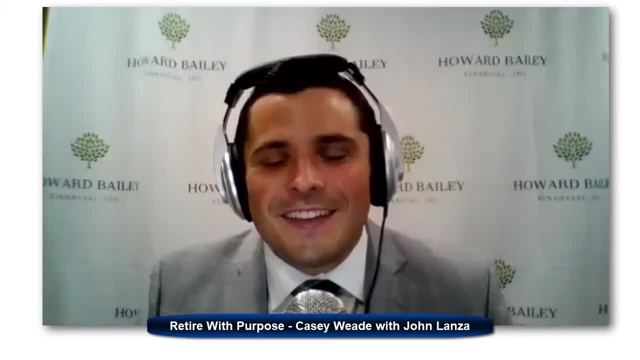 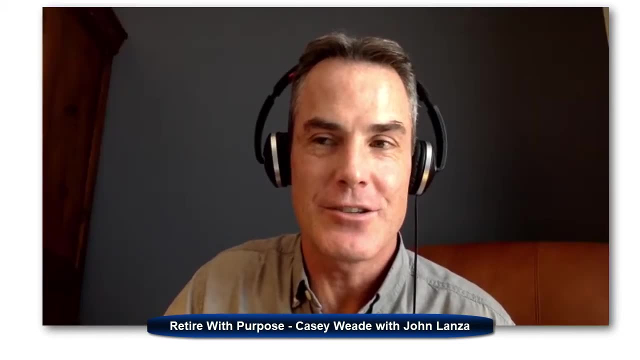 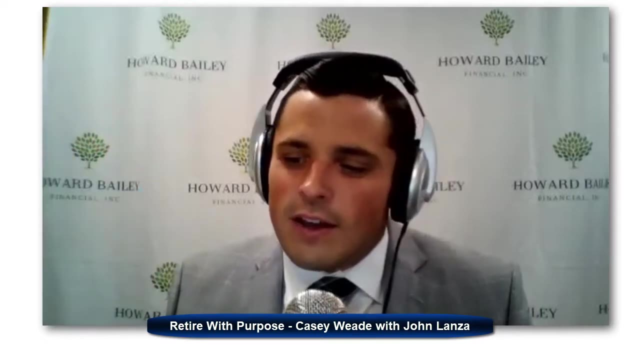 As a matter of fact, it most likely means that she's not going to get it. Well, I think – Yeah, Yeah, So you know, be open to doing those kind of things with your kids. Yeah, I think you wrote the – that leads me into a point, because you wrote the book on, really. 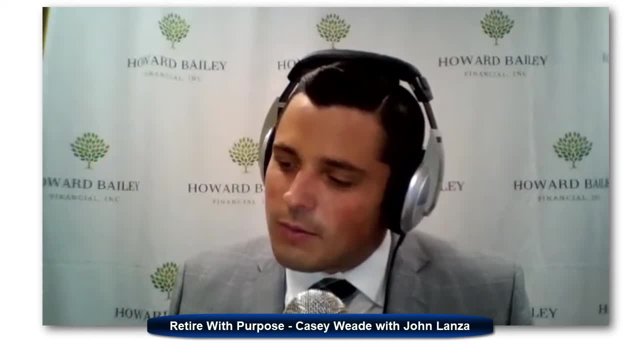 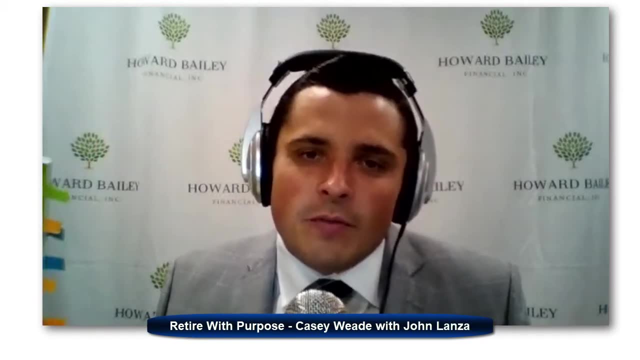 a practical guide to raising money-smart, money-empowered –. I kind of felt like it was aimed at parents. However, I feel like it also is applicable to grandparents. Now, from a parent's perspective, I think many times we go, okay, well, we can walk. 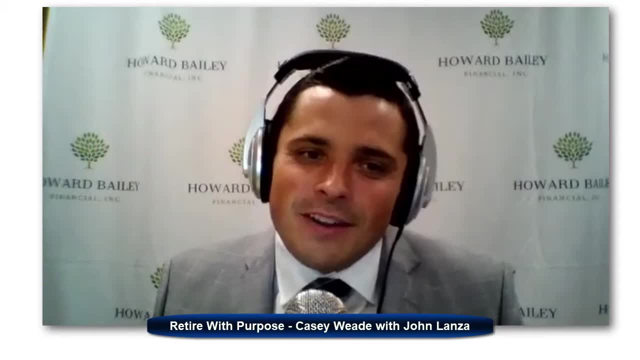 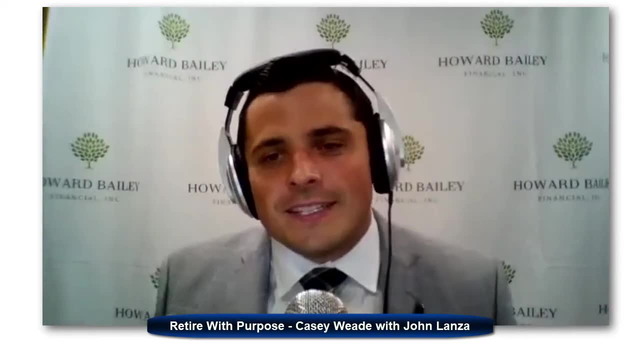 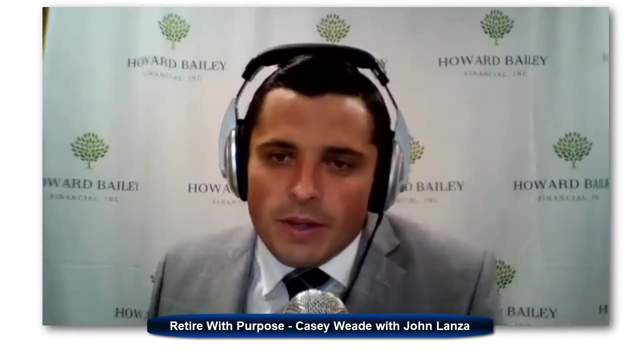 through that line and say, no, That is grandma. Is grandma going to also say no, or is she going to cave in and now we kind of create some animosity and some issues that way. So how do we have that conversation as a parent with our grandparents to make sure they're? 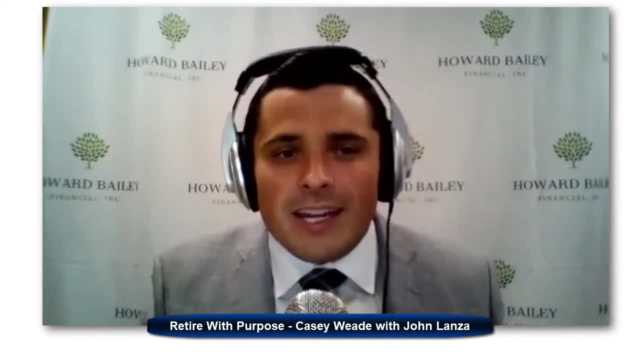 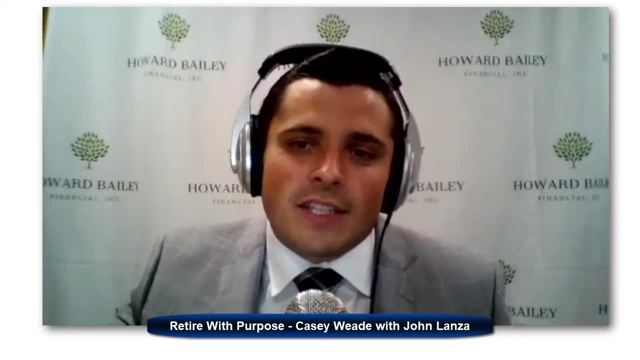 following the things along the lines that we're doing and I don't think that conversation is nearly as difficult as it typically is, maybe for a grandparent that wants to have that discussion with their child about how their child – you know, how their child. 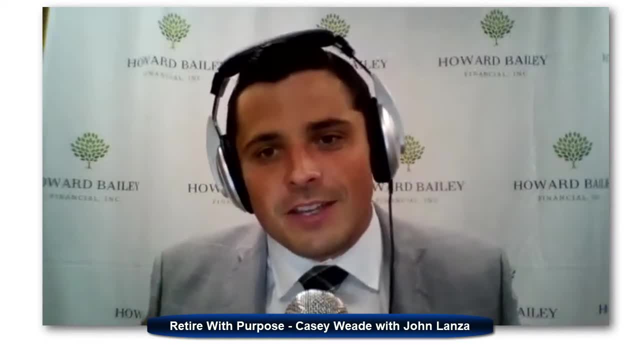 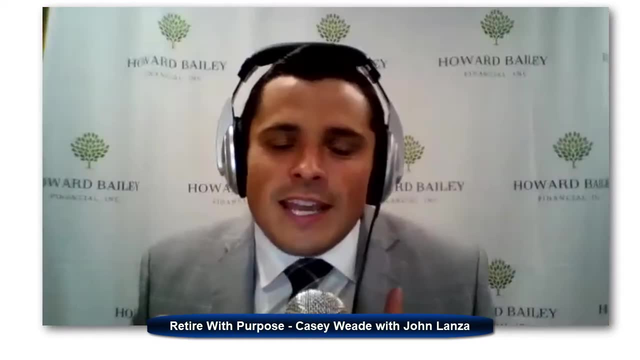 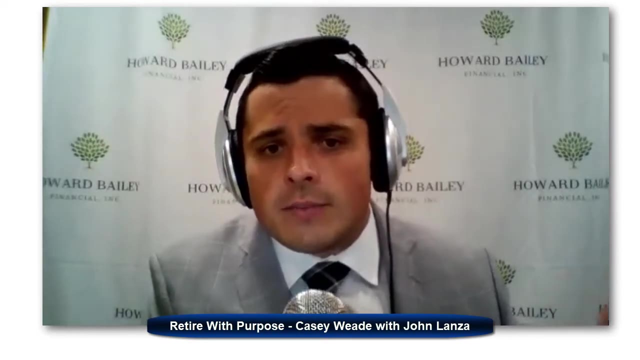 you know now we're trying to tell our kids how they should be raising their kids. Well, that typically doesn't go over very well. How does that grandparent have those discussions? How do they approach this money-smart topic with their child about raising a money-smart? 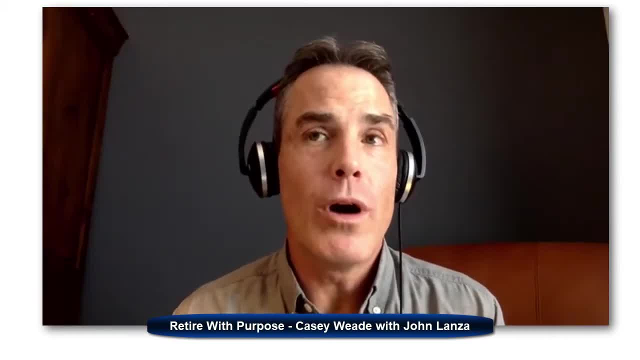 grandchild. Yeah Well, I think you know one way is to – not to be mercenary about it, but you know, providing them with a resource you know, And so one of those things can be, you know, a child. 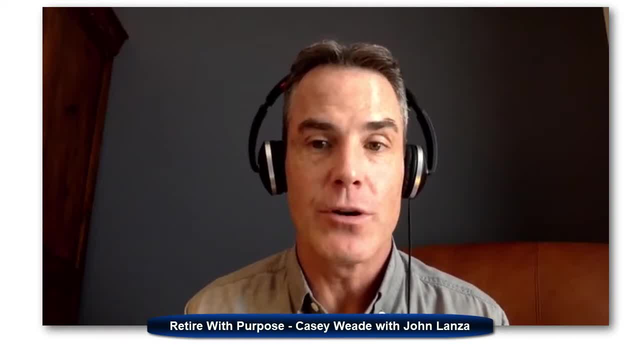 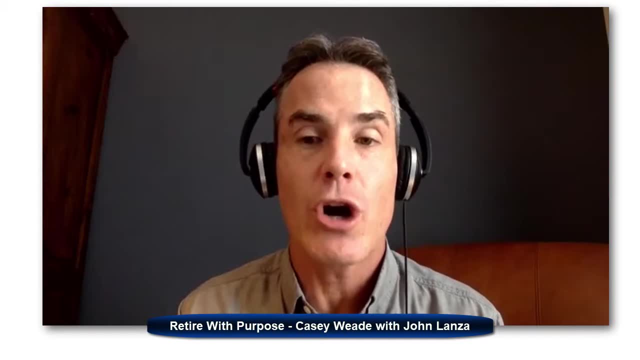 Yeah, Yeah, Yeah, Yeah. You know something like the Art of Allowance or turning them on to a podcast like this. you know something – an interview like this to show them that – because one of the things as a parent, when you're caught up as a young parent where money is not – you know like. 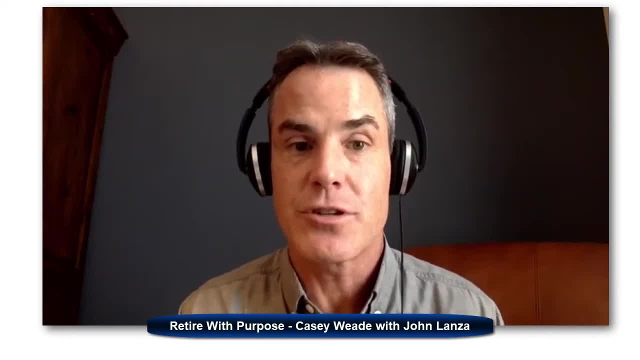 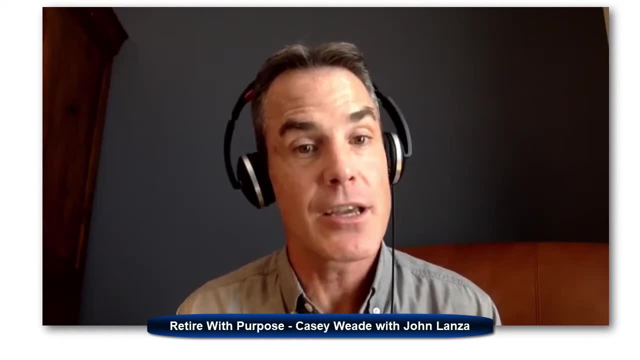 for you it's more obvious: you're a CFP, so this is of interest to you. But for other parents they just have – there's so much else going on. so as a grandparent you can kind of throw this into the mix and say: you know, here's something I saw that. 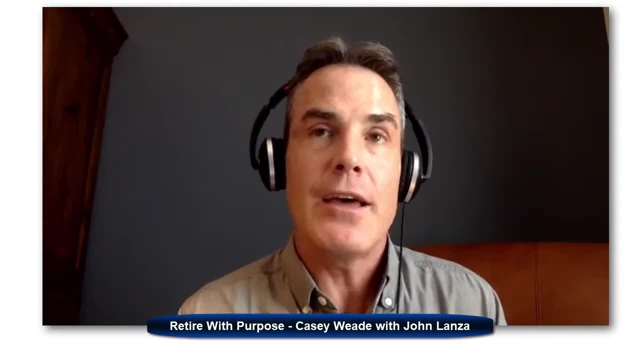 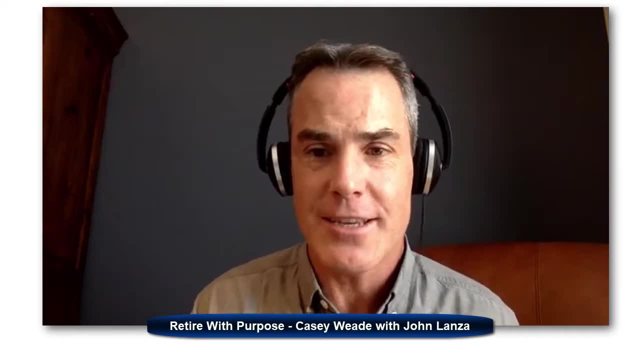 I think you might be interested in. so that's one. And then now, the one thing about the – Yeah – grandparents, and this is when you're a parent and you do start a program, is the Grandparent Bill of Rights, I think, says that they have the ability to spoil –. 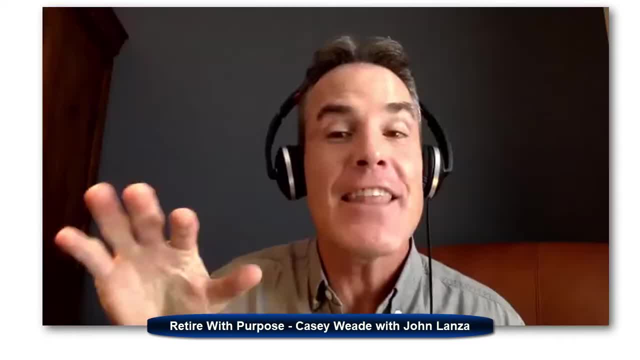 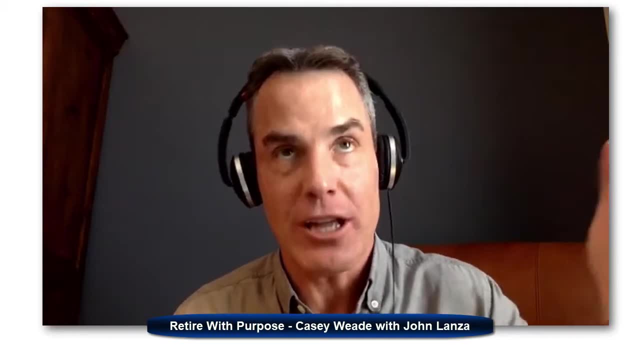 Overwrite anything So they can spoil the kids and that's you know. that's fine. But I think you had mentioned, like, how do you have the conversation? I think you had mentioned the conversation from grandparent to parent. so we talked about. 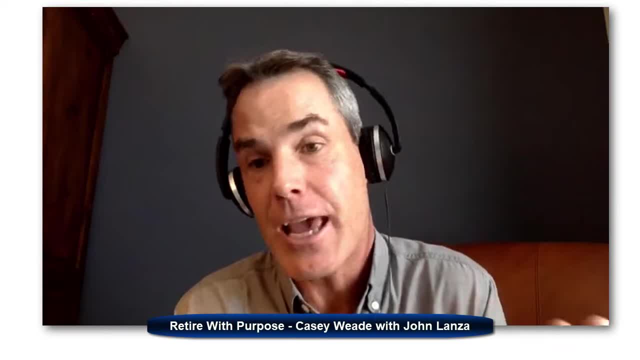 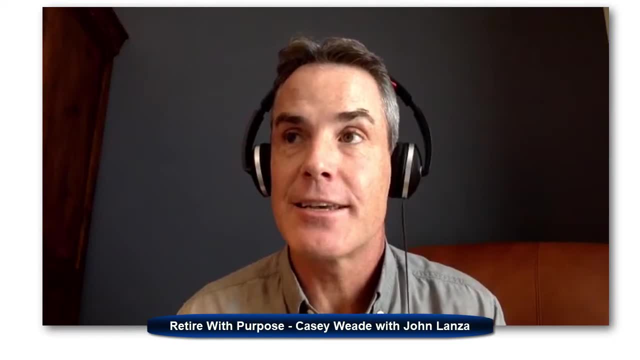 that I think you just kind of nicely present these things and you can't – I don't think, as a grandparent, you can be overbearing about it, because you just have to understand that, Yeah, You just have to understand that your kids have so much else going on. 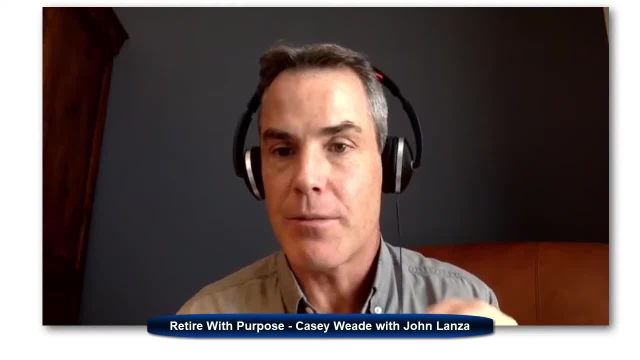 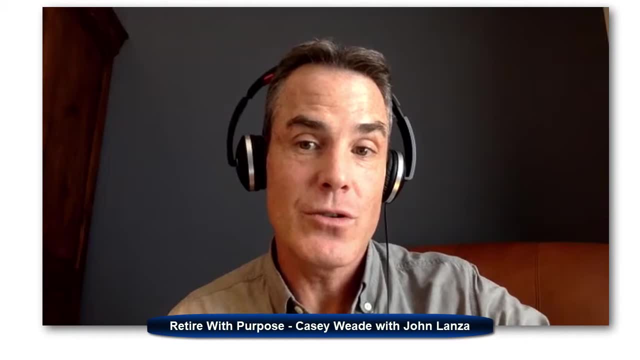 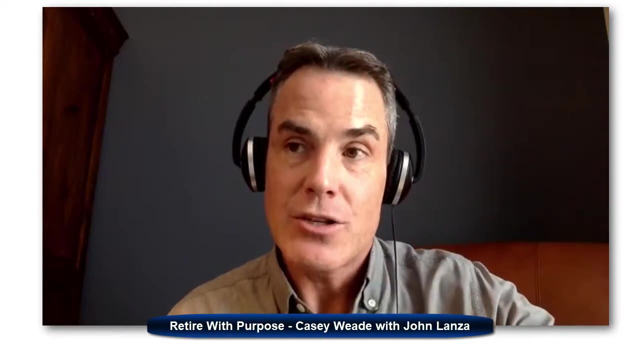 But it's worth finding a resource that you think might alert them to how important this is to start young. So that's one, But then the other way – then it's important for the parents to have a conversation with the grandparents once they've started a program. 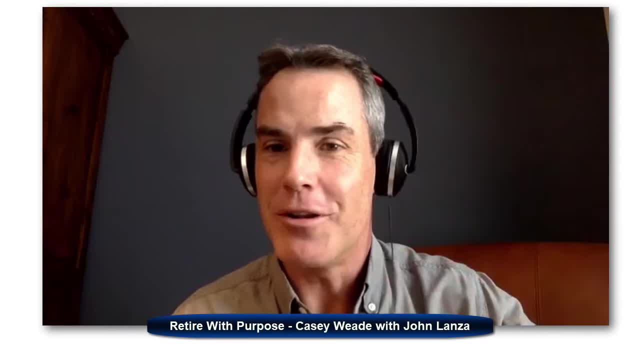 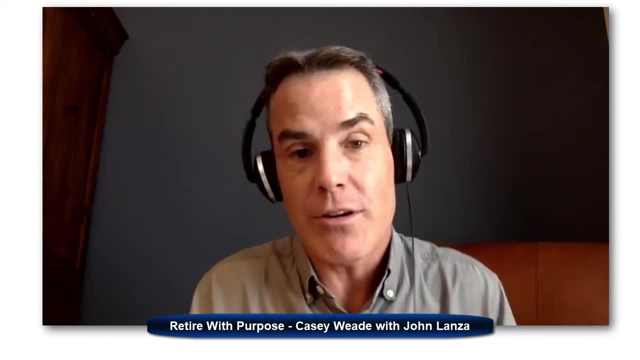 So not to say that you can't spoil the kids, because, again, that's part of the Bill of Rights for grandparents, Yeah. But, for example, my mom got involved and we said: here's what we're doing with our kids. We give them the three jars. 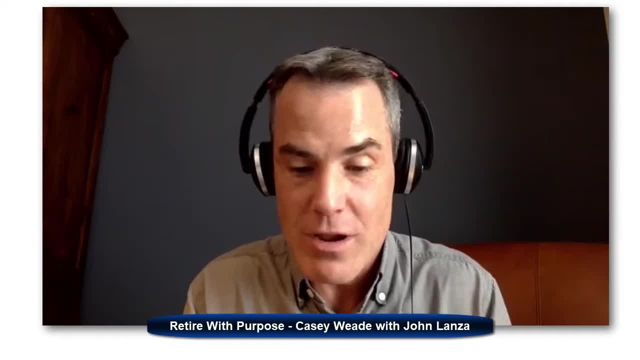 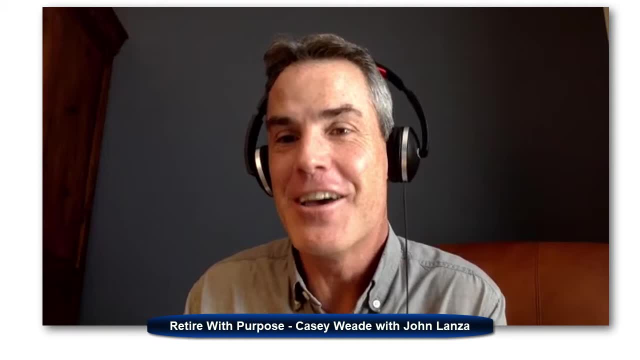 And so she would send them a card with money and there were three $5 bills and one would say $5 on the share – it said share jar. The other $5 had saved and then the five had spend smart and the kids had to put those. 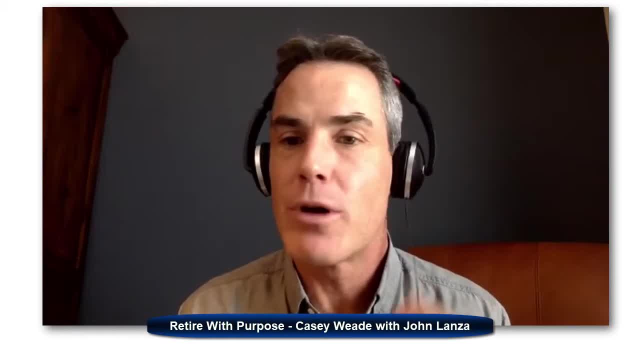 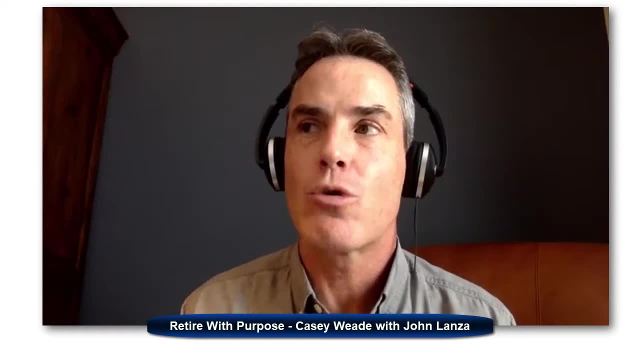 into those jars So you can employ – you can bring your grandparents into the mix on this. And that's not to say – not all grandparents are going to do that, But I think grandparents are always looking for interesting ways to contribute to their 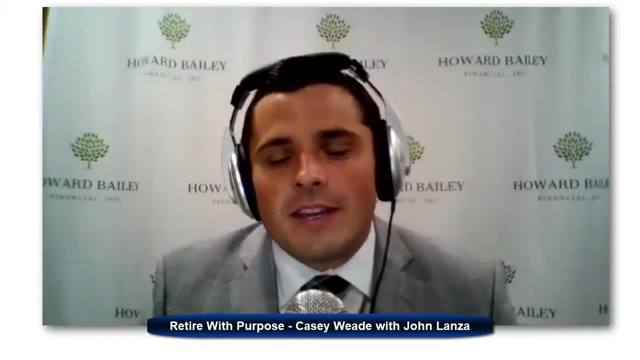 grandchildren, Yeah, Or just have fun with them. I mean, it's a great way to have a conversation with your grandkids. And I was very blessed because I grew up with a financial advisor for a father and an elementary school teacher for a mom. 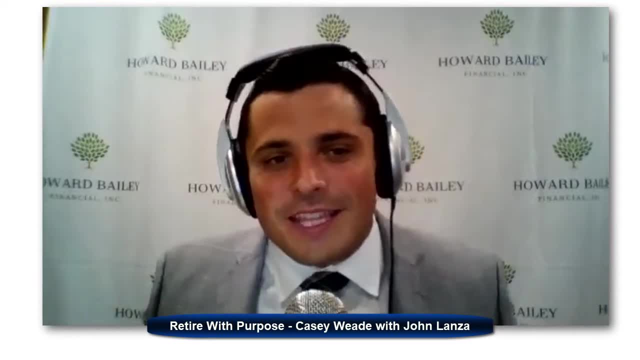 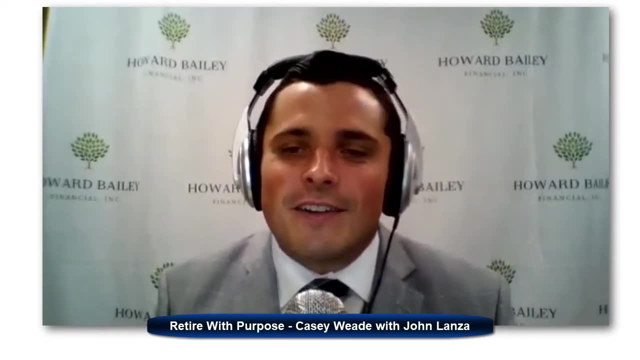 And so they really combined forces in order to provide me with the envelope system. We didn't have jars, but we had the envelope system when I was a kid, Of course, And it was the same way as you've laid out here, and I think it really helped me, as I was growing up. So it was easy to do that, And I know, as soon as I get off of here, I'm going to order two more copies of The Art of Allowance and I'm going to send a copy to each of our sets of grandparents and then 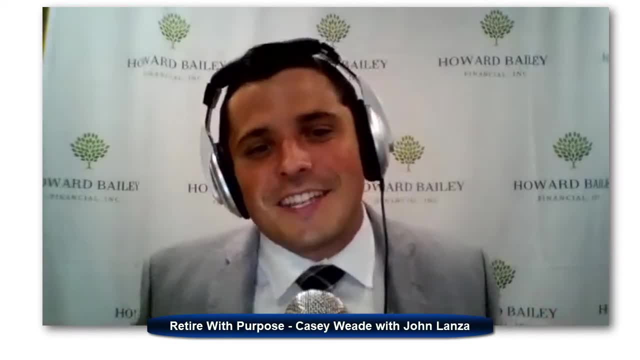 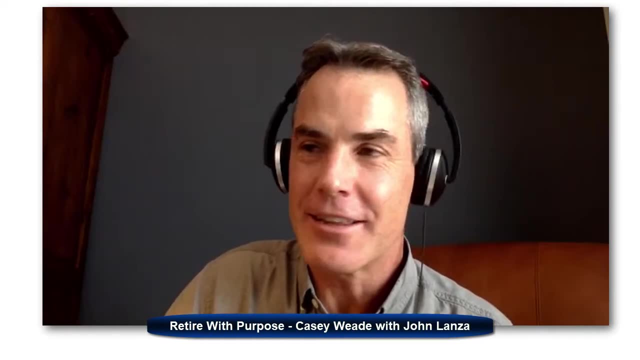 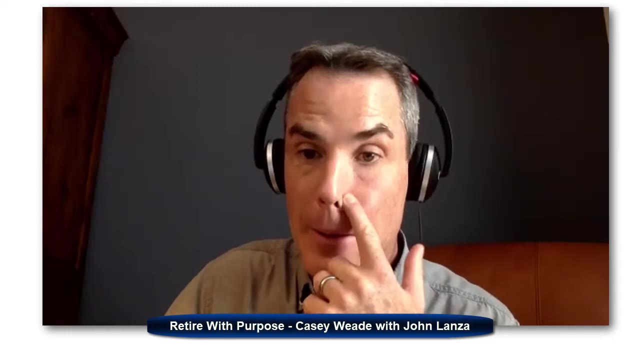 that's a nice nudge, as you had kind of touched on previously. Yeah, Yeah, And I have to shout out because sometimes I think my parents, if they watch this, they think that – I think they did a bad job Sometimes when I say they didn't set up allowance. my parents are wonderful and one of the great. 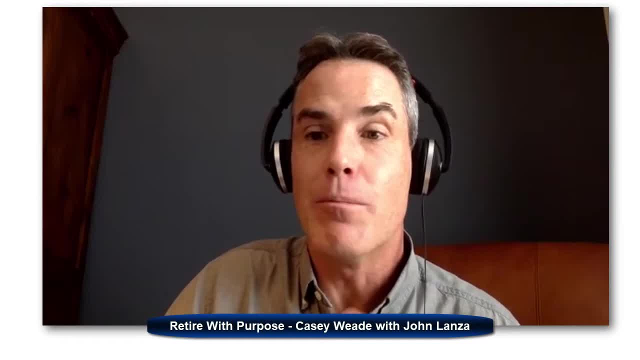 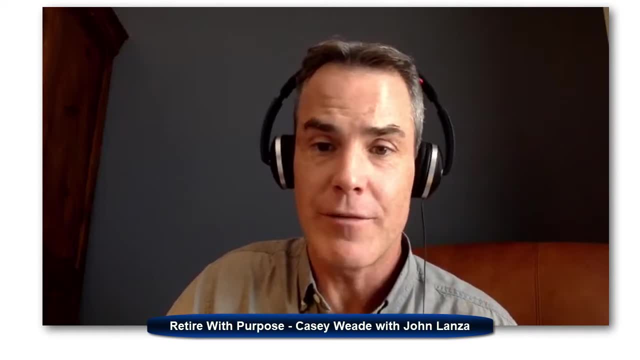 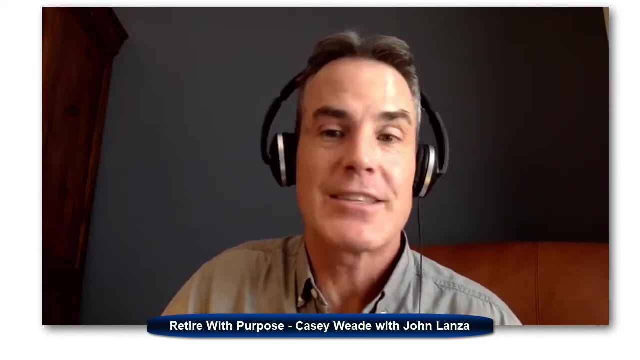 things that they did, both my dad and my mom, is that they're both very frugal And so just their actions, the way they – because my dad always drove kind of beat up cars because he just didn't care, He realized early that – it's the same way I feel. 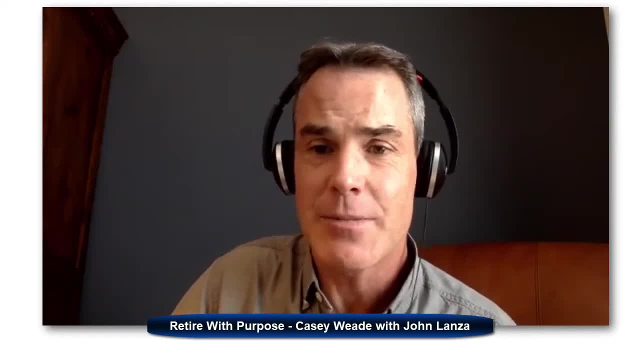 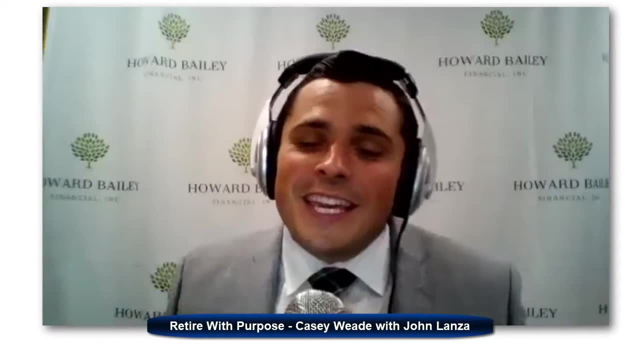 I drive an old 2002 Honda CRV and my kids are constantly asking me to get a new car. and said: you're going to treat a new car just the same as this car, which is – Right, You can't have a nice car when you have kids. You have to wait until they get out of the house. then you can have a nice car. You treat this like a crappy couch. Why would I get a new car? But the point being that my parents really – they were very frugal and so that was. 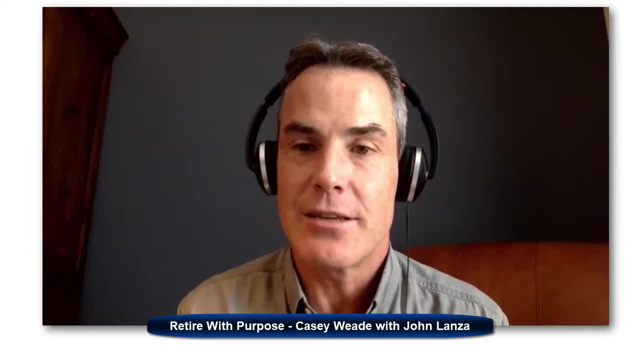 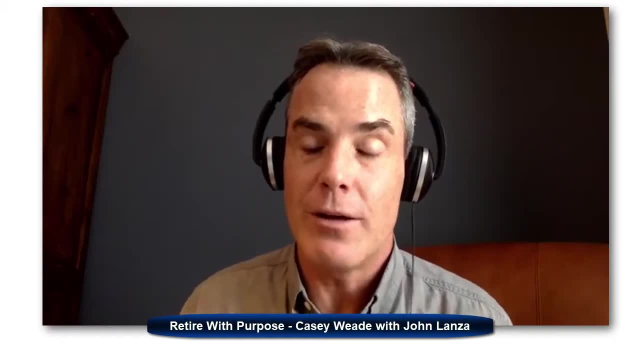 a great example to set, and we try to be as frugal as we can. I think my parents were probably even more frugal, So they did a really nice job with them. Yeah, I think, on that note, we've just lost touch with that kind of way of life that those previous 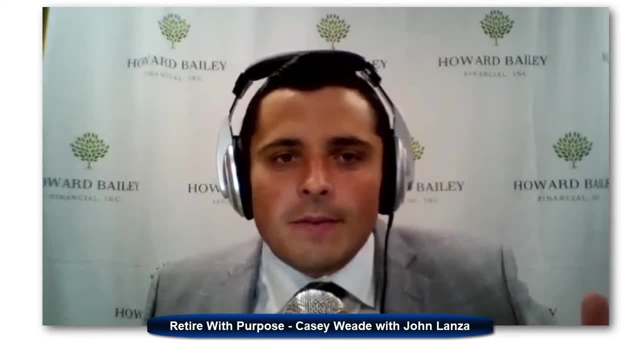 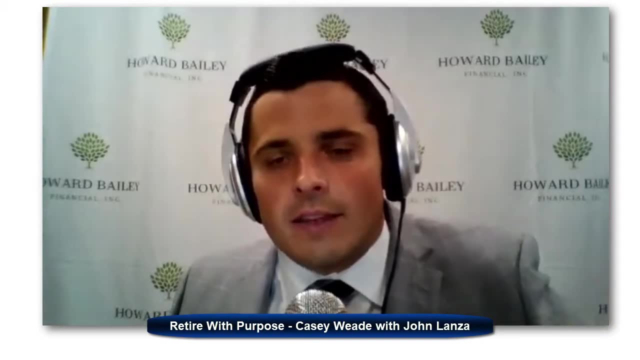 generations had. I mean, you had your parents, but probably their parents grew up during the Great Depression and they still kind of maybe had a – they still had a taste of the Great Depression. They passed that on to you and now I think, this generation of children they've experienced 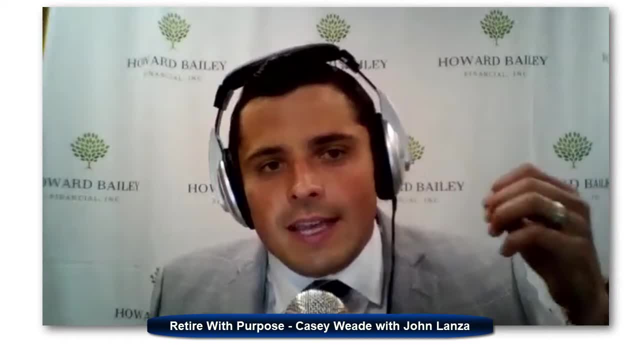 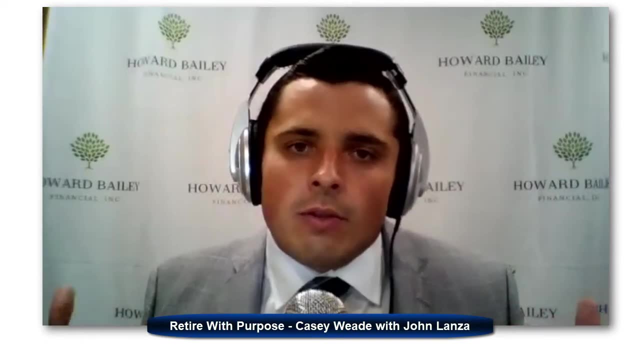 that they're not going – they're so far from that Great Depression and that mentality that they had. I mean, now it's just credit cards and you're always going to get rescued if something goes wrong. I think we saw that through 2000 and 2003.. 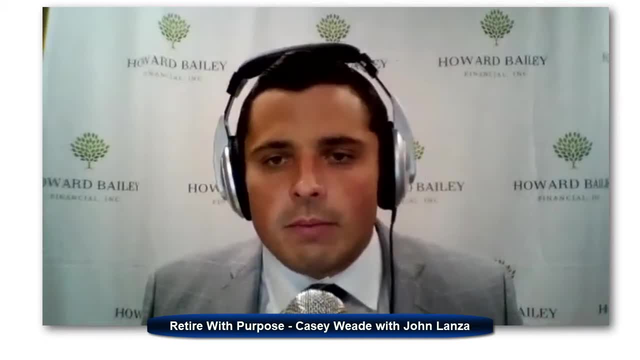 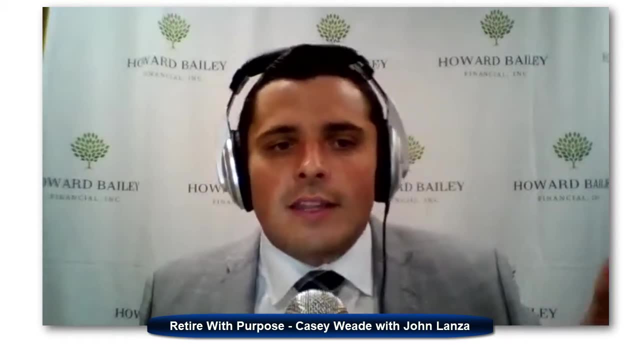 We saw that really heavily in 2008 from the federal government stepping in and bailing everyone out, And so we go. well, I guess we're always going to be okay. The government will always save us, And that's one of the questions we had from our family. 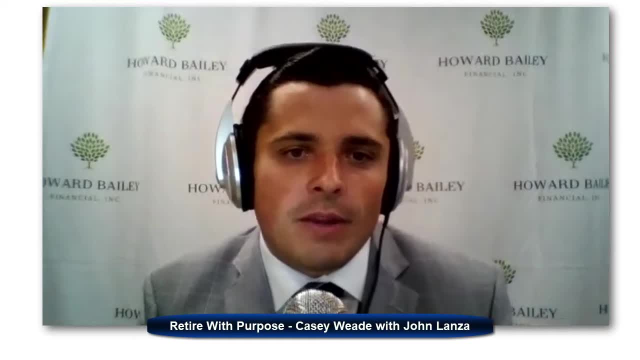 We had John Shadacki ask how can a grandparent inspire grandchildren with an appreciation? John Shadacki is a father of the loan shark. John Shadacki is a father of the loan shark who's been to the bipedal state. 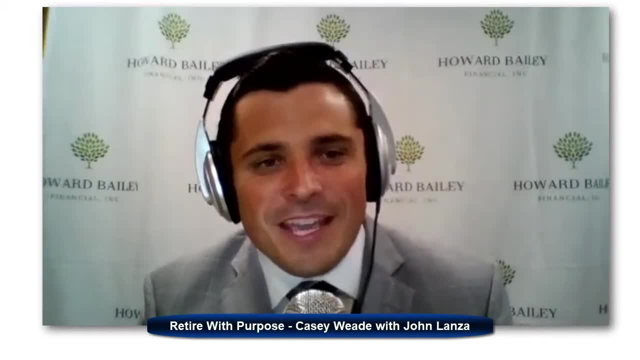 He's the founder of the New England Law Association. The law is an animal. He was an eight-year-old boy and he was a child. He was born a today. He was a white man and he was placed in a middle school and he went to bed with me. 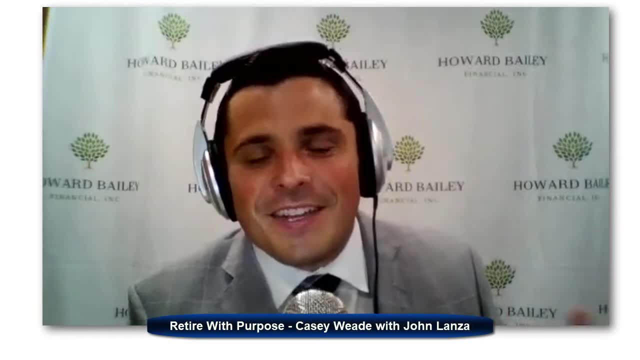 at a young age, and you know, that's why he's so important, That's why it's so important to me. I think all of that's important to them. I think that's why all of us- we're all you know- we're in the process of having 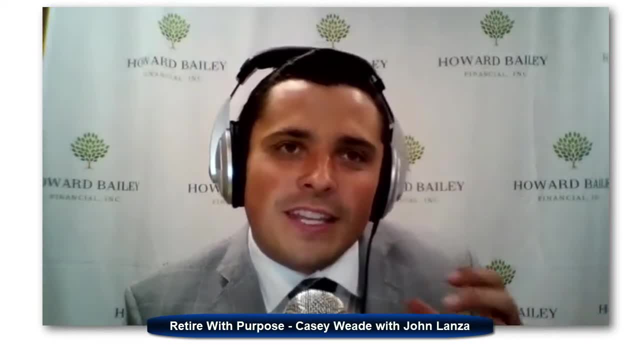 our children born and you know that's why we're rarely the first to look at the law. You know we're just sort of looking to make it. we're looking to come to Europe because kind of get them back to those roots that our grandparents had. And that is why I named the 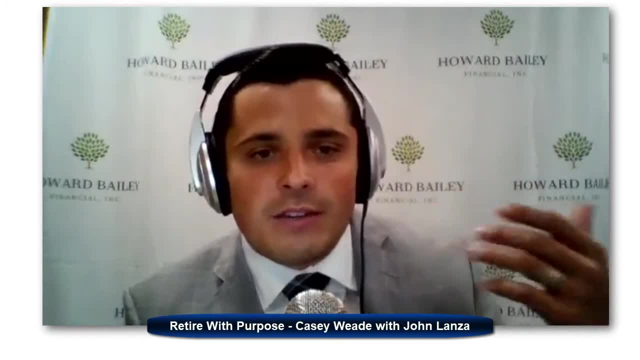 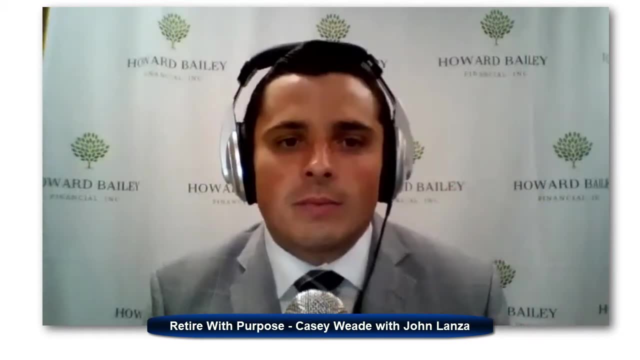 company Howard Bailey Financial is because Howard Weed and Ralph Bailey- they both grew up during that period of time And and they taught me a lot of these conservative common sense principles. How do we get back to that? Yeah, it's a good question And you know, and I, and like we talked- 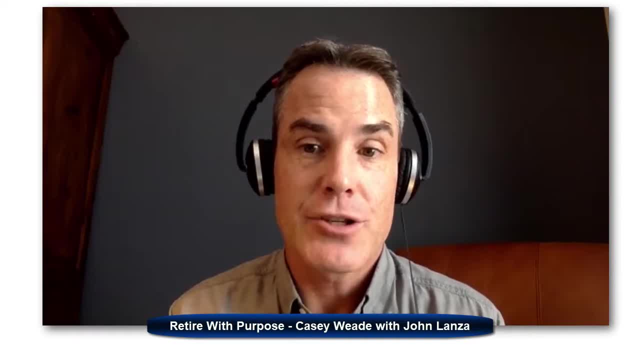 about. I dedicated my book to my grandfather And certainly he was a big believer in capitalism, You know, also believed in the social safety net and on a practical level as well. But you know his two big lessons, two big lessons to me that he that took me longer to heed than it should have. 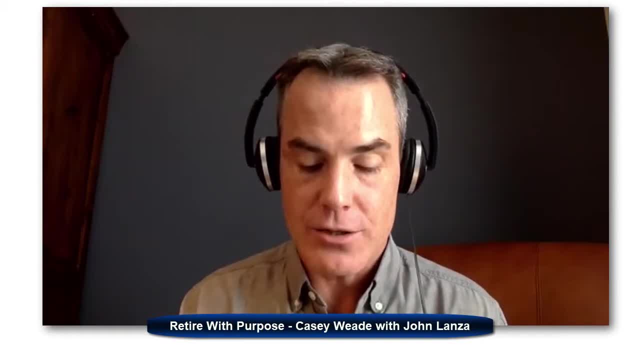 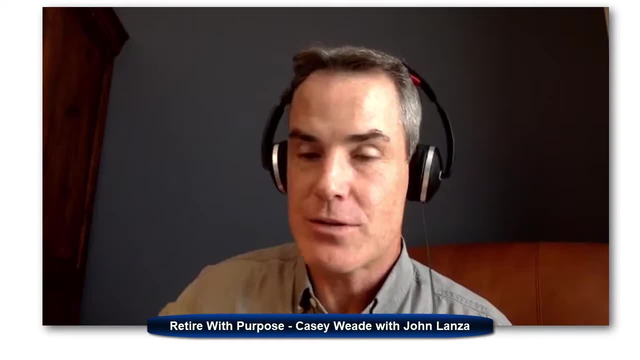 were live beneath your means and to understand the power of compound interest, And it's the reason why we have it up. you know, it's right on the wall for our kids is a compound interest chart, And it's something that we make it up, And it's something that we make it up, And it's something that we make it up. 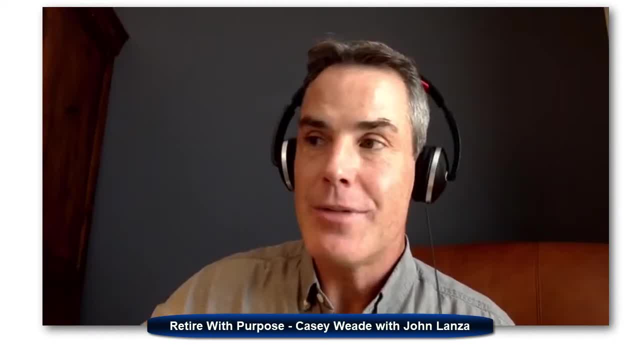 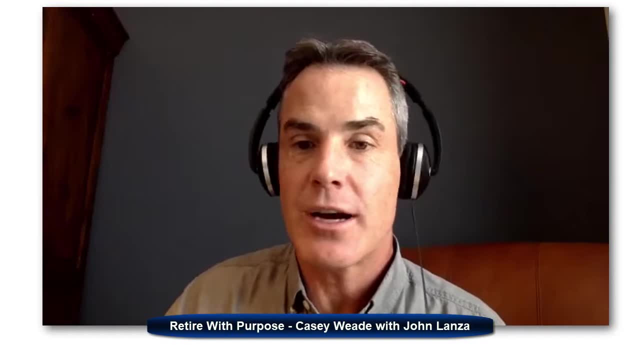 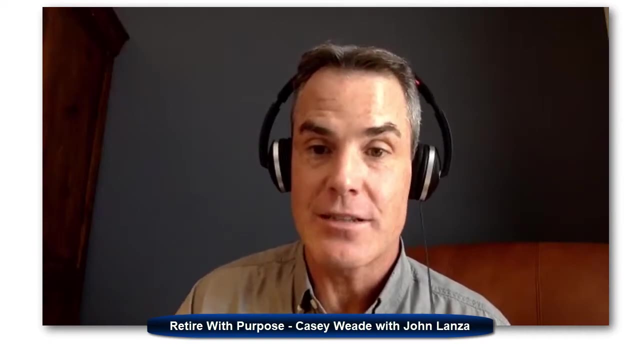 And it's something that we make as a downloadable on our site- a compound interest chart- because it's as powerful a concept as you could possibly imagine And it's one of the things we tell our kids on an ongoing basis. It's like: get that if you get your money invested. 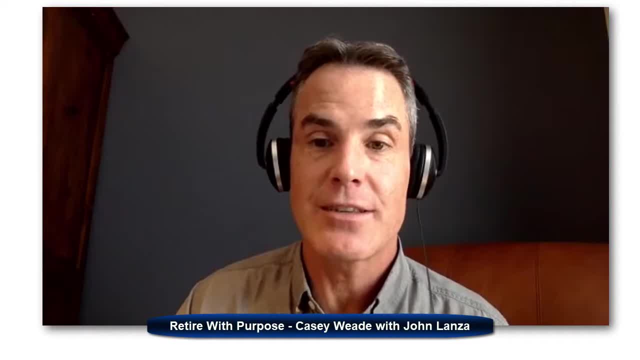 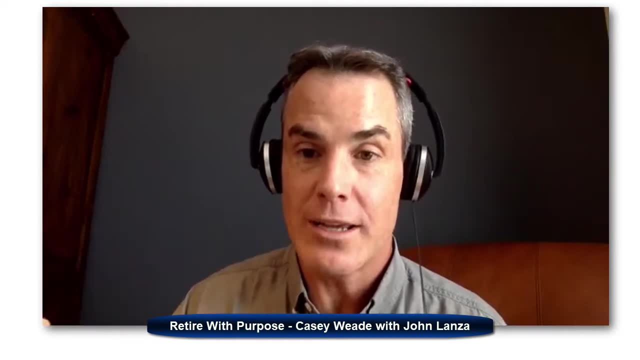 from an early age, before you go to college, you start investing in something as simple as an index fund. you are really going. you're going to achieve money, empowerment really much sooner than than we have and certainly sooner than most of your friends, And that's going to open the world. 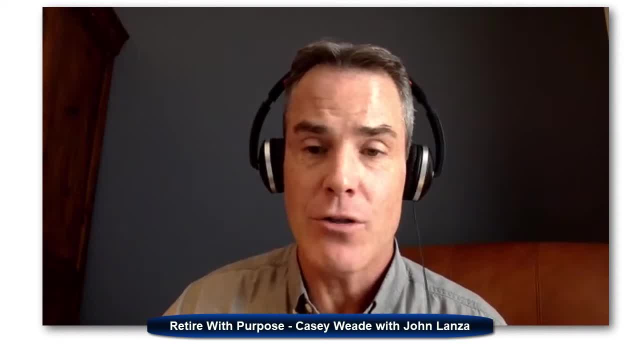 up to you. That's not to say that you're going to retire and go live in a yacht when you're 30 years old, But you will be able to do what you want to do, And that's that's really. that's that is. 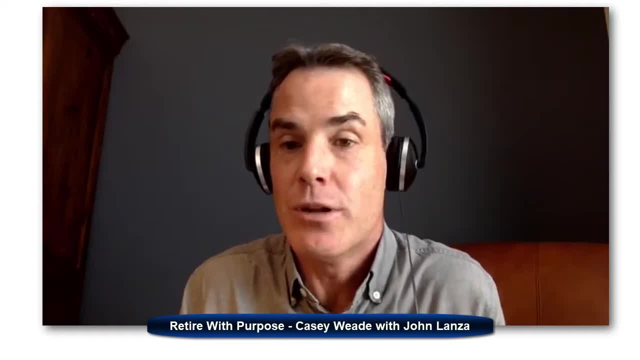 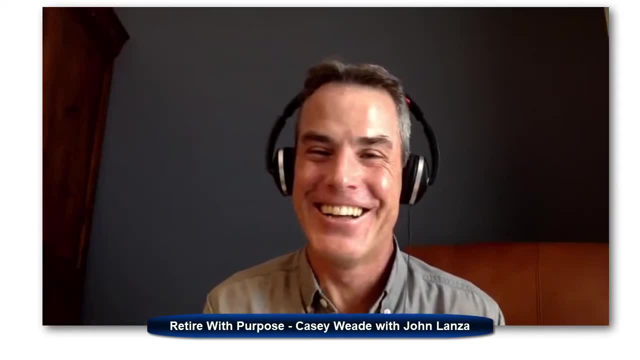 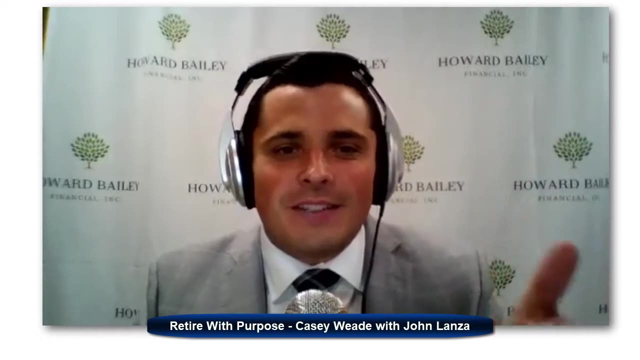 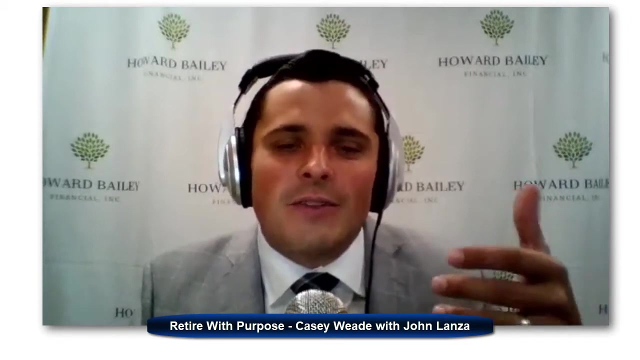 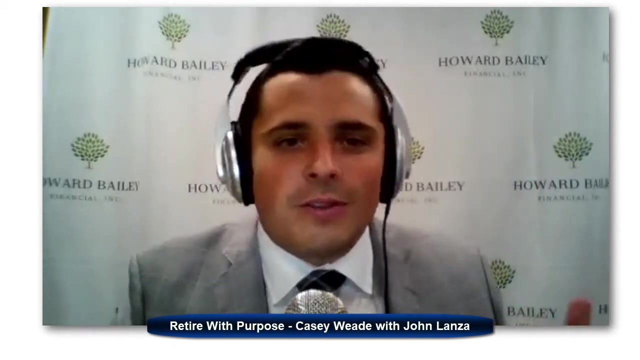 what we, that's what you ultimately want to do is use money as a tool And those two ideas out of the house. You found me out. I figured it out now. Well, that's one of our other questions I think you started on. there was about the time value of money. Bruce Johnson asked: is the time value, is the time value of money, interest explained? How do you explain compound interest to? I mean, I it's, I think it's. it gets a lot easier when they can read a compound interest chart. They're 15 years old. they should be able to figure that out As it's explained and taught by you. However, how do you teach that to a younger child? 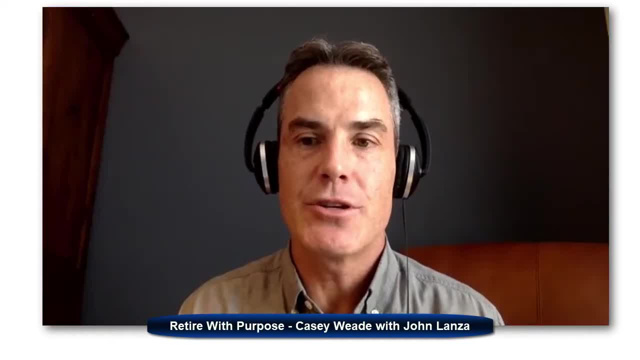 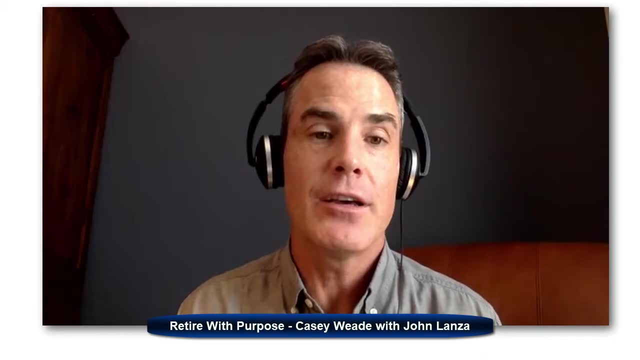 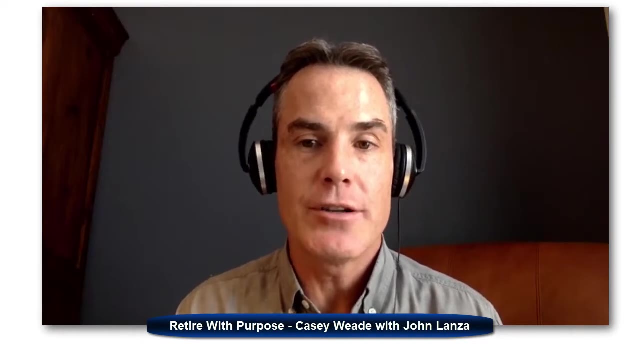 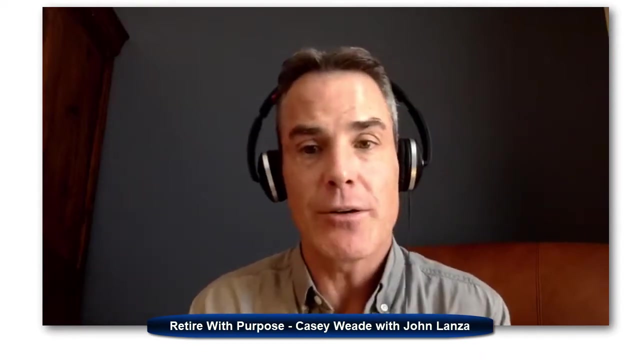 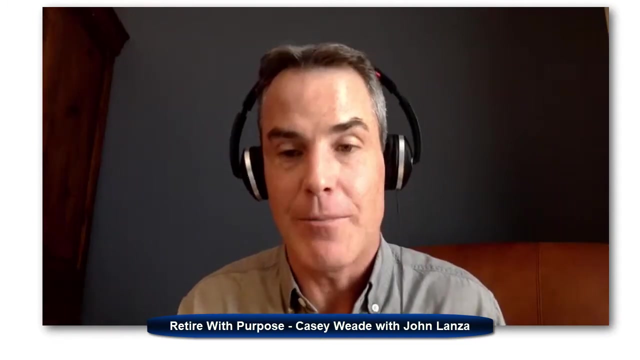 Well, you're not going to teach them about compound interest per se, but you're going to teach them about delayed gratification, And that's that's. that's a big part of it. So that's that's why the saving in a jar with your visualization is so important, because the earlier the kids can learn delayed gratification, the better off they're going to be. And you know like, there's that famous the marshmallow experiment that Walter Michelle did, where the kids come into they have a researcher, have a down a marshmallow, and they say: you know, they leave them in there for a certain amount of minutes. I forget what it was: five minutes. 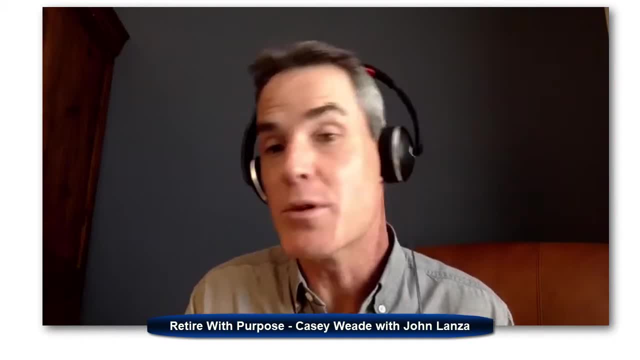 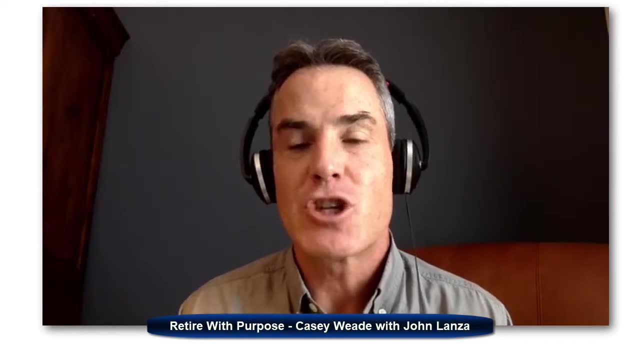 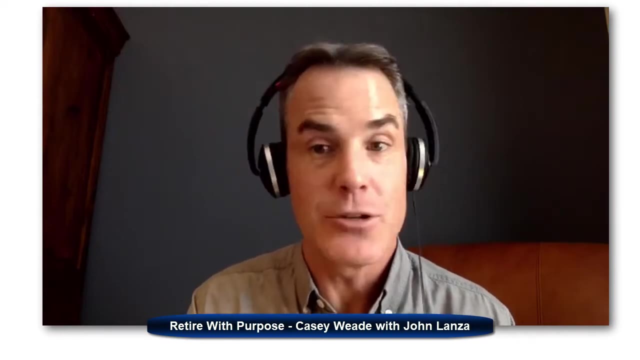 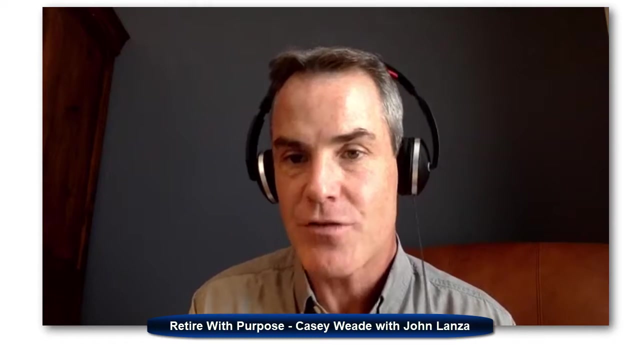 And they say: if you can wait here for five minutes, we'll give you a second. Yeah, I do remember this. Yeah, And so the kid, and they found that the kids who could kind of distract themselves were the ones who are successful at. you know, they just would, they wouldn't look at the marshmallow. you know, there were the kids who just kind of ate the marshmallow, but then the kids who could distract themselves come up with some kind of way of kind of getting through those five minutes and then we're rewarded with the two marshmallows. 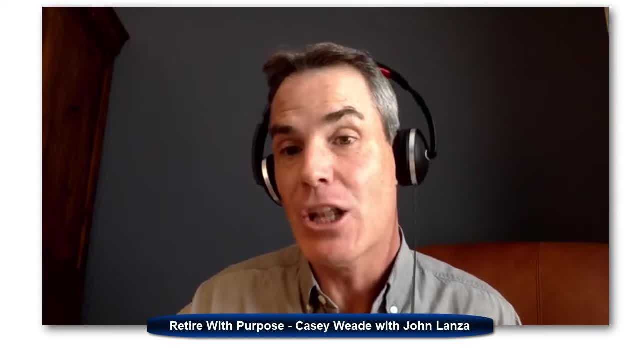 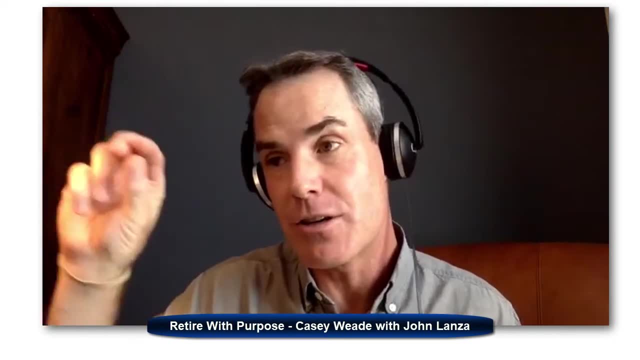 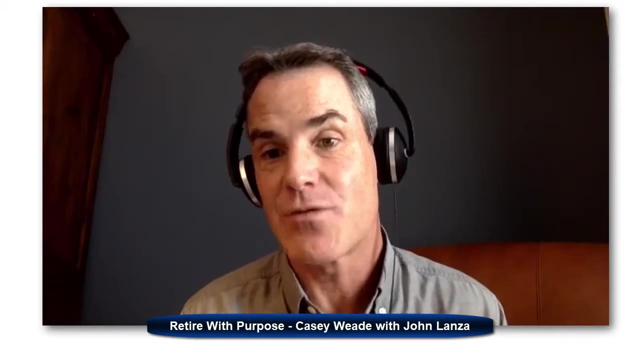 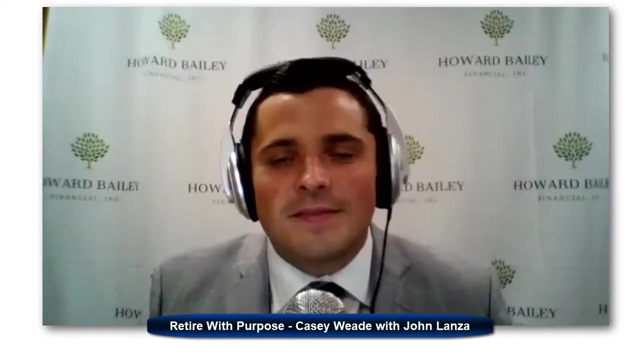 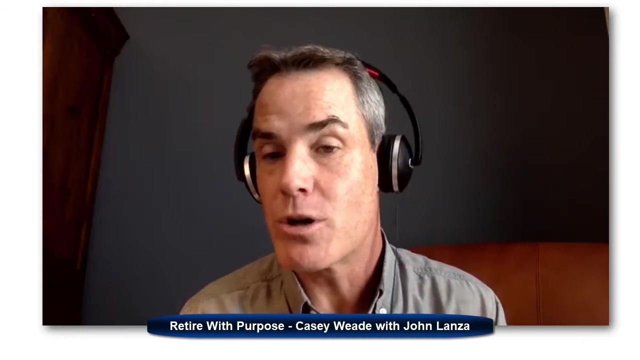 I think more importantly, Michelle went and looked at those same kids when they went to college and and beyond, and he found he did it. it took a few metrics and found that the kids who had displayed delayed gratification had had success, more successful life outcomes. So higher GPAs, lower BMIs. he had a whole- I forget the list of metrics that he used, But the and then the. then the key point is: can it be taught? and it can be taught And that's what we're trying to do with these kids. 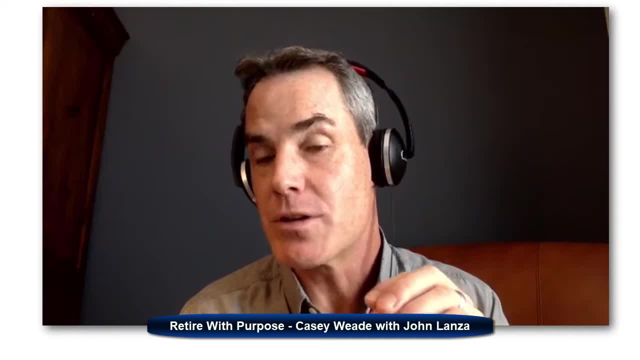 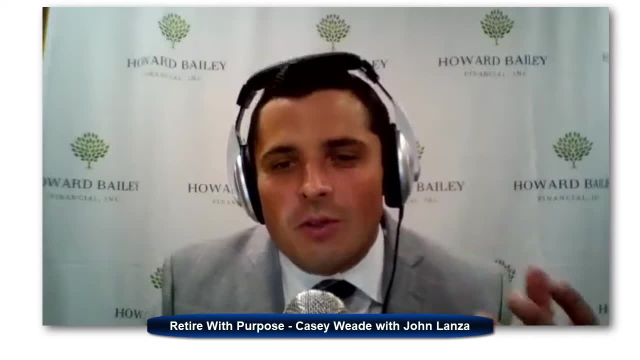 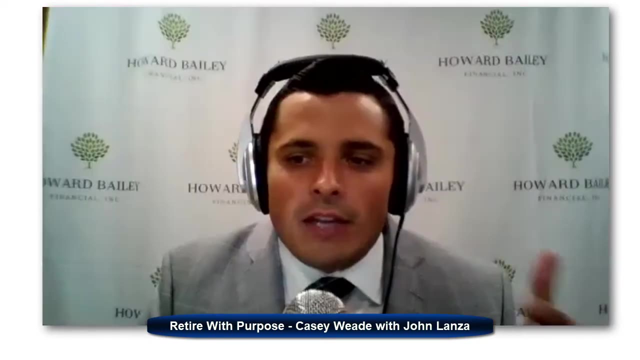 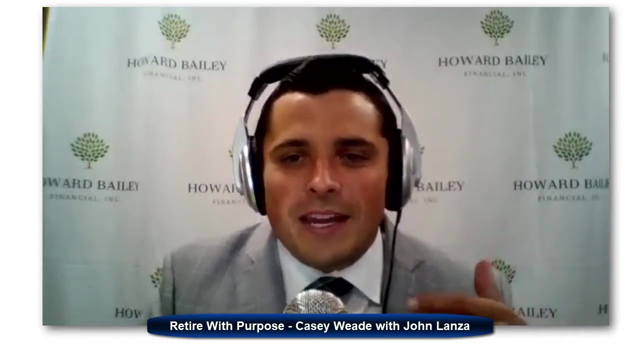 Yeah, with the save jars, what you're doing with that three year old And that's what we start with the five year old And that's what the jar is about. So that delayed gratification is the way, is the beginning. That's the core, right. I mean, that's the core of what you're trying to create out of the art of allowance, And I think you can still incorporate this matching concept in order for them, or like the way you explained in the book, with you know, kind of a 401k match, right. they're getting 4% with every single payment they put in there, where you can teach them the value of compound interest. 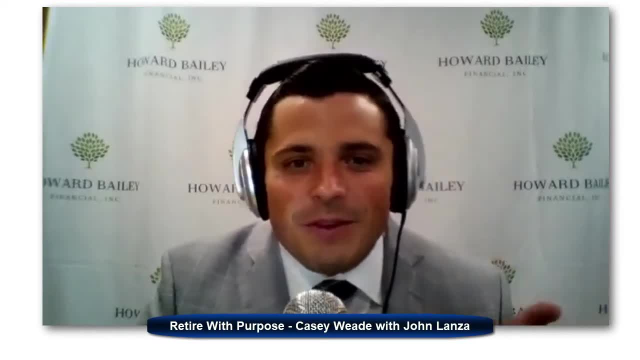 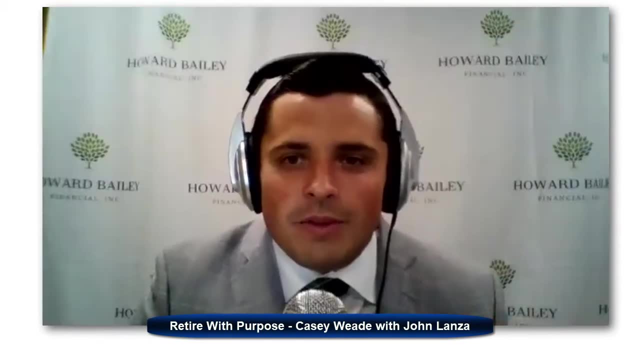 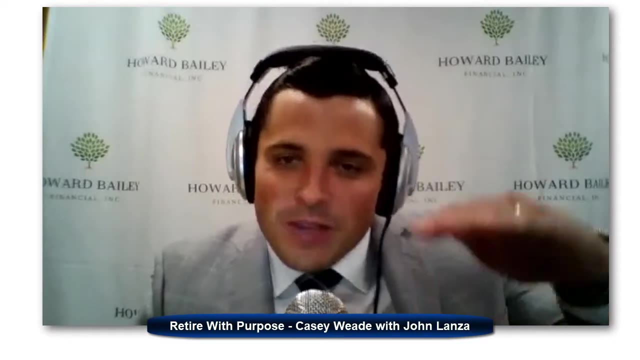 by and that's difficult for them to understand. But very quickly, I think after a few weeks, even with our three year old, I think he's going to see how you know, if he puts in $1, and we put in 4 cents every time he puts in $1, he's going to see, especially when it's four pennies, that jars at least going to be starting to visually fill up so he can visually feel what compound interest is. 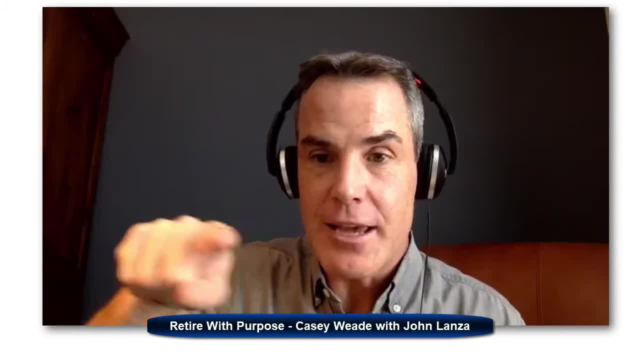 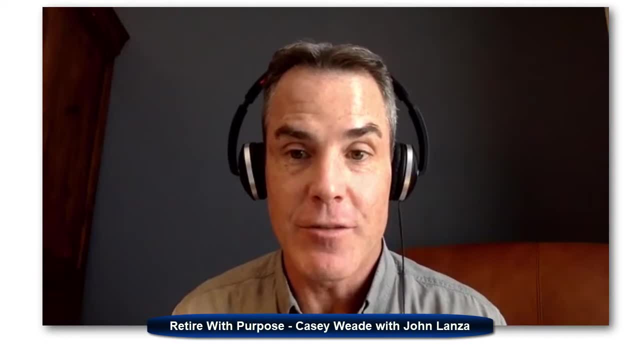 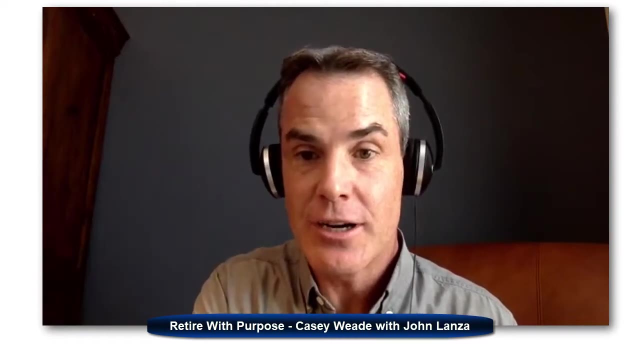 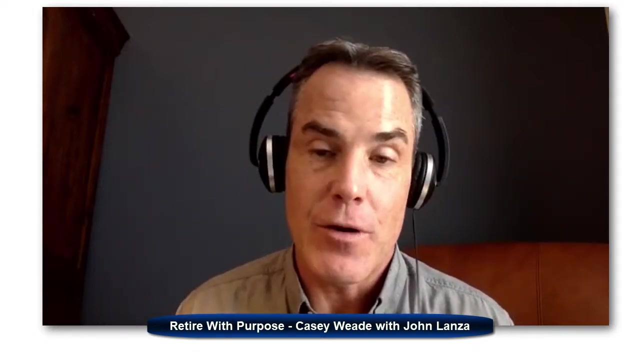 Yeah, that's exactly right. So they're. they're not going to understand the exponential curve of it, But they're going to get exactly. you know what One saving is a good thing for me to do. Two, if I save this dollar that I could put in the spend jar, if I put it in my save jar I get. you know we were we were doing at the beginning. we do a quarter for every dollar that they put in the save jar And for a match, but you can do dollar for dollar. It's really 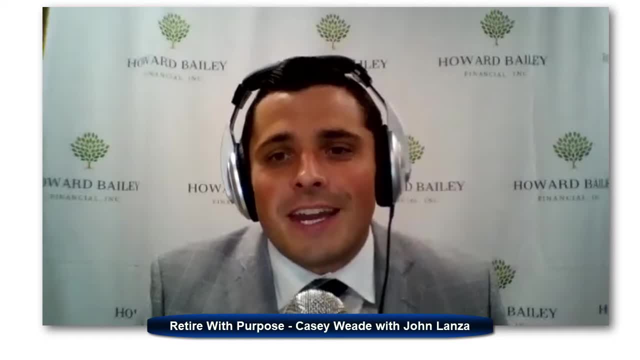 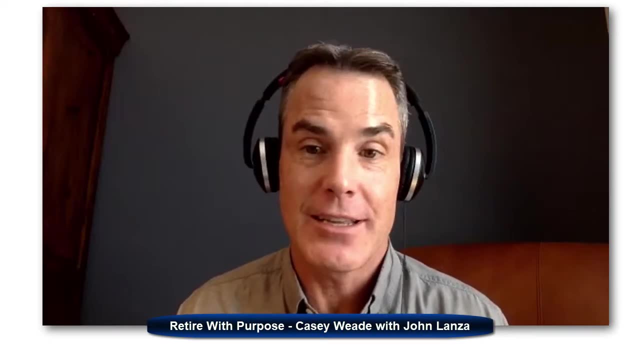 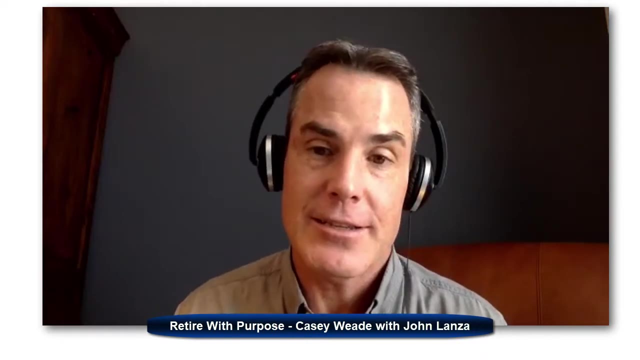 25% match a week is a heck of a match. I'll take that It is a good match, And and and but. but you could make the argument that a dollar match makes sense because, Sure, You're just trying to teach them that saving is a good thing for them, you know, And so that's it's. it's the point of doing a starting. a matching program just makes a lot of sense. 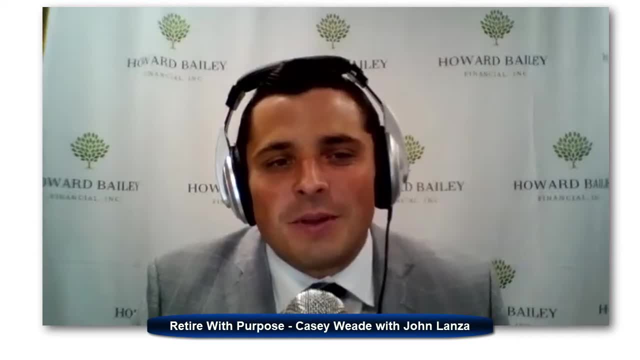 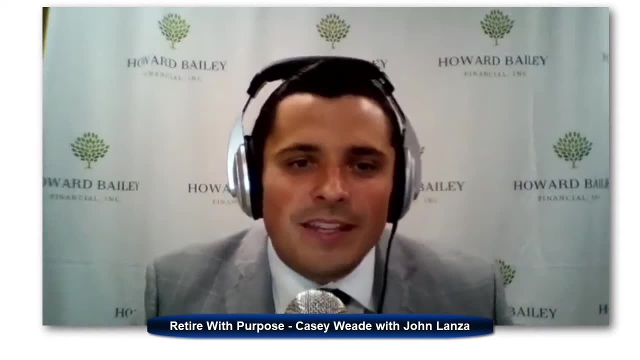 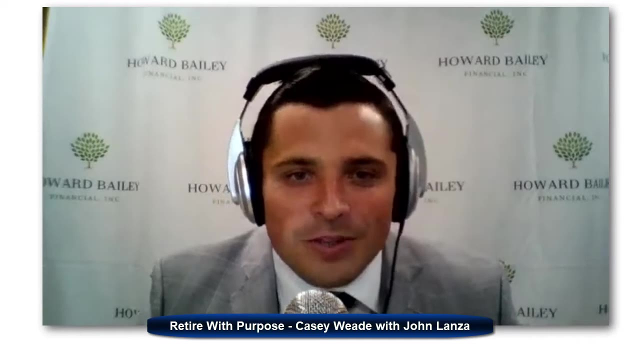 So we've got one last question from our fans. We've got a question from Ken McIntosh, And this is a practical question. He asked: Have you co signed debt? Now, your kids are not at this point yet, but will you, Right? So have you co signed debt, student loans or mortgage, I guess in your case, 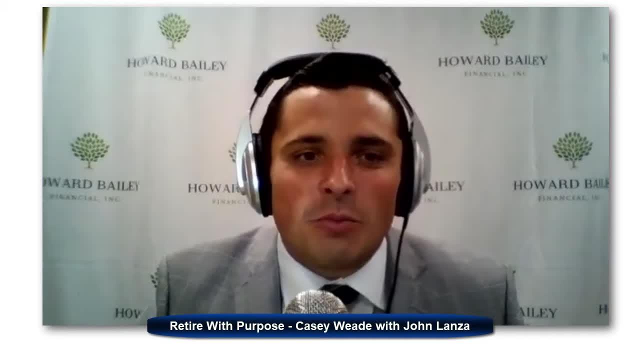 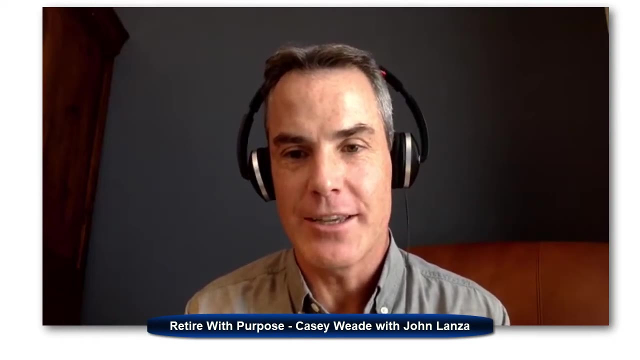 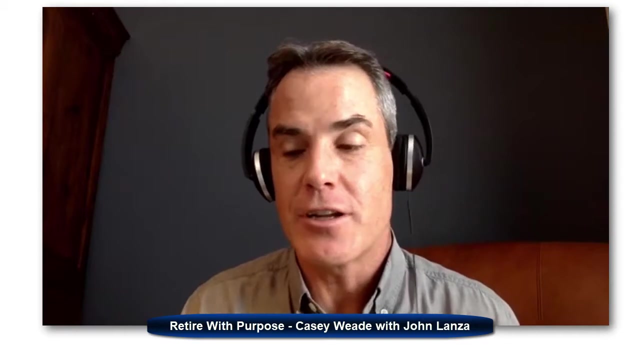 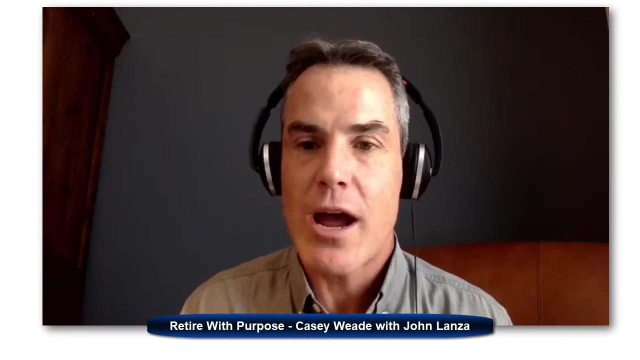 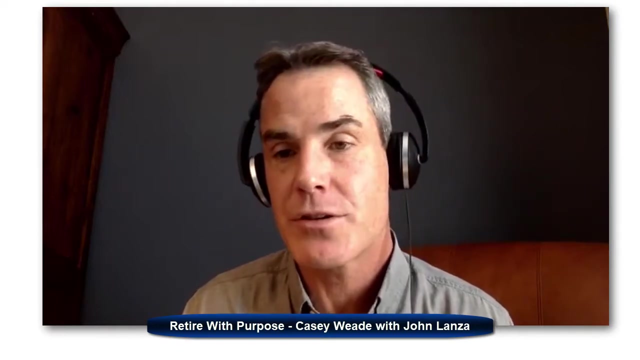 would you co sign or advise someone to co sign on debt, student loans or mortgage with your children And do you honestly think it will be paid back when you retire And may need it? You know I have not thought about that question, So I'm not going to answer that one directly. But the one thing I will say, though, on the student, on the student debt side, is: we've all, so our kids are 15 and 12. They know exactly how much they have in their 529. And we, we have consistent: whenever we've traveled, we'll take them to college campuses So they get a sense of how much these the different campuses costs, like state school versus private school, And we were just having this conversation, So we're going to get back to that. 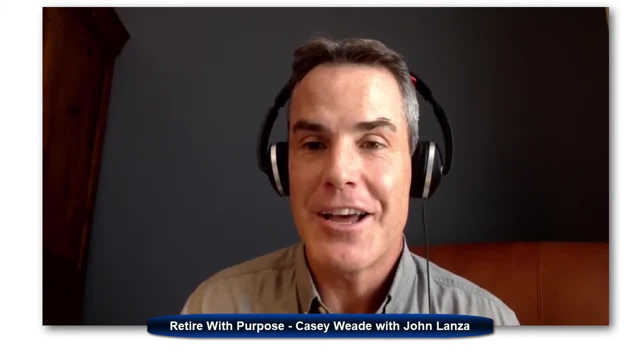 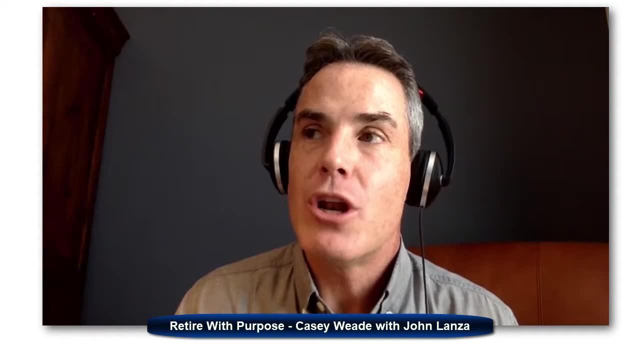 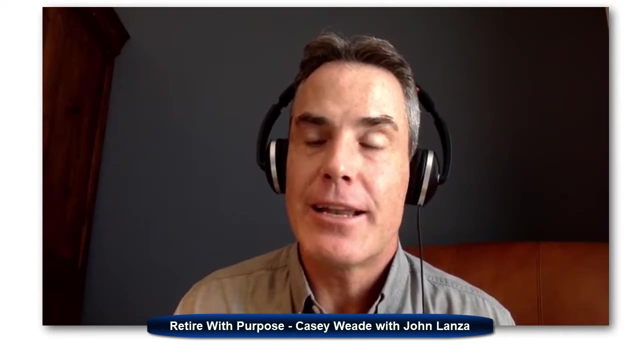 conversation last night, because you know our 15 year old is uh heading there, you know sooner than than we might imagine and we what we know. they know that, uh, they know that the that, that they're that, that it it can get out of control with the paying for the for uh for college, right, so that's. 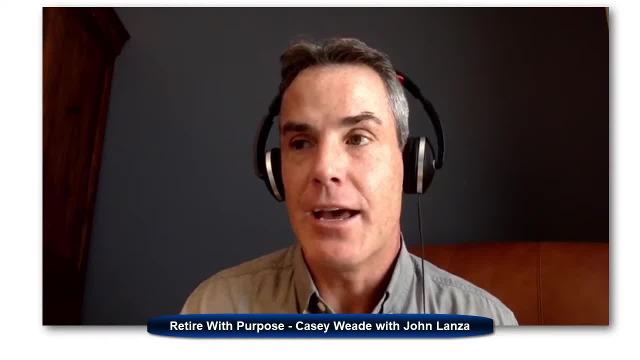 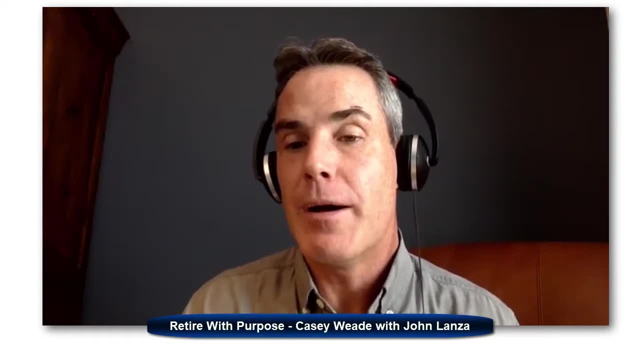 why we've opened up the conversation with them and that's why they know exactly how much money that they have, so they can start making that calculation. um, one of the best pieces of advice that i got- i think again this was bill dwight- was a loan is not a bad thing to do for your kid, so i 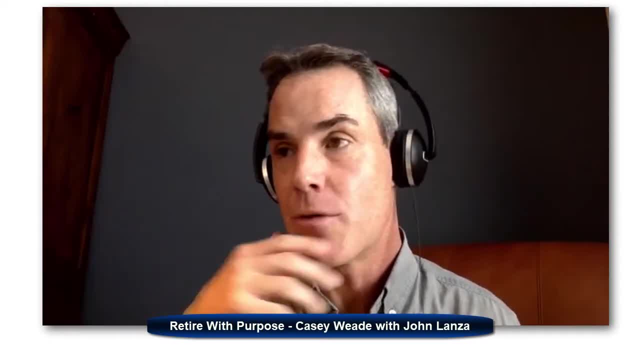 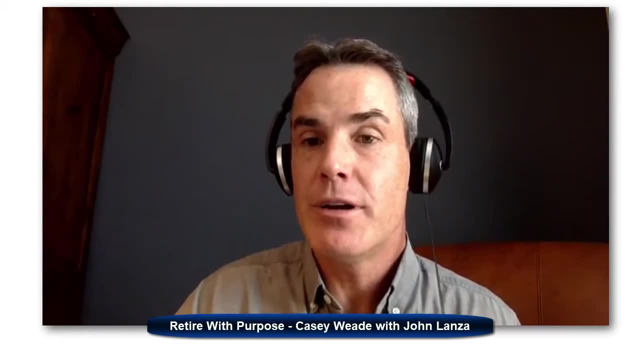 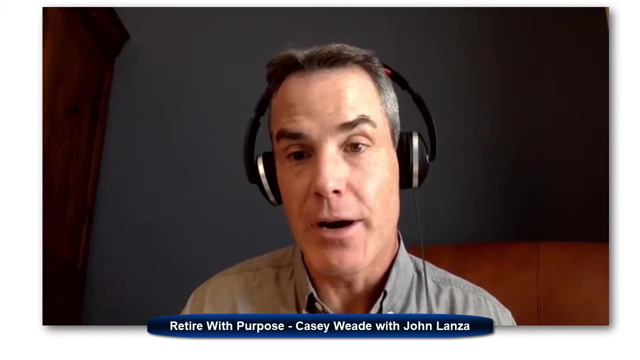 won't talk about necessarily like co-signing on debt, uh down the road, but uh, he has. the example that he used, which i thought was really good, is that his kid had bought a computer, trashed the computer and wanted him to buy another computer for him. he said no, but he didn't have the money. 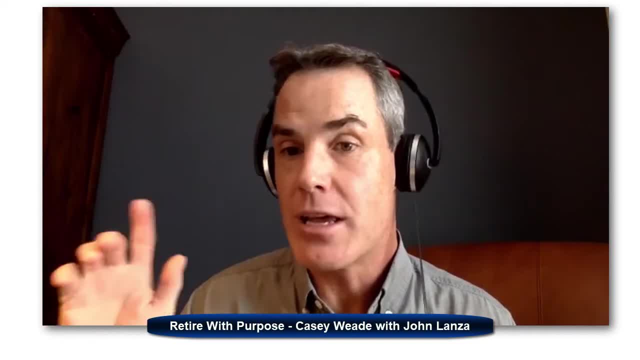 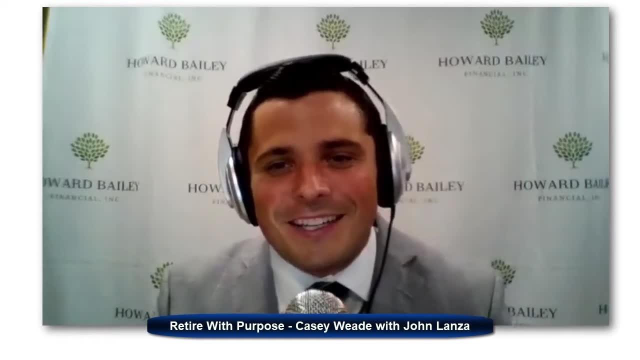 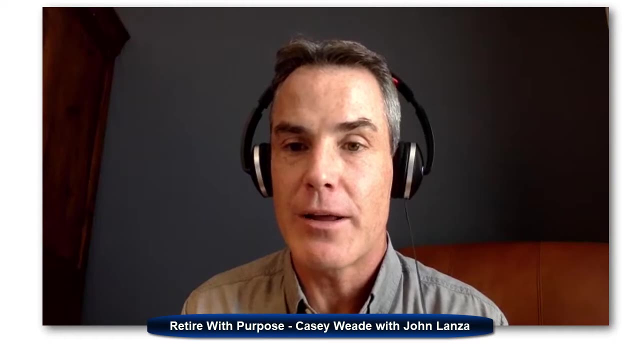 said i'll loan you the money, and it was. you know. he collected the interest and the kid took much. i loved that story. i listened to that podcast you had- if john also runs a podcast- art of allowance. that that is excellent. that was a really good point. it was. it really was powerful and i'm- i'm gonna do the same. 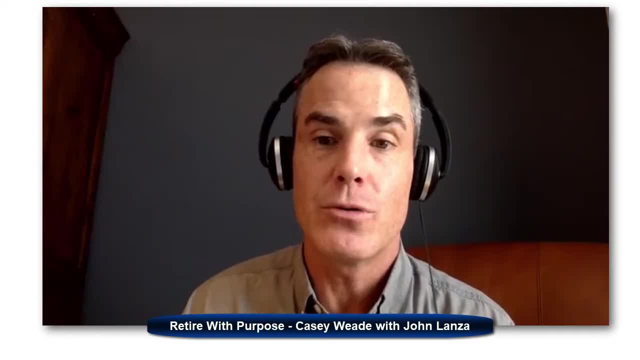 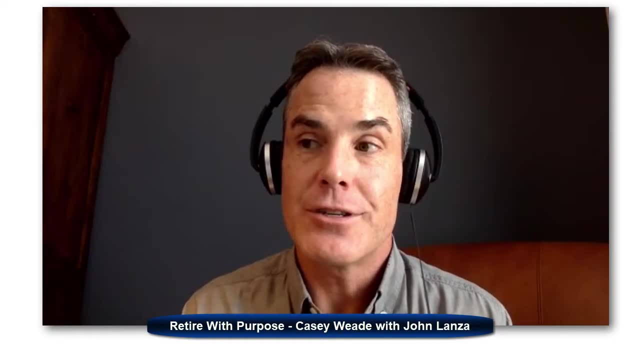 thing, because one of our kids wants to go on a trip to uh rome next year and it said: we're, you know you are gonna have to pay for at least half of that trip. and she's like, well, i can't. you know that's either going to be. she's going to have to take a job. it's probably going to be both taking a. 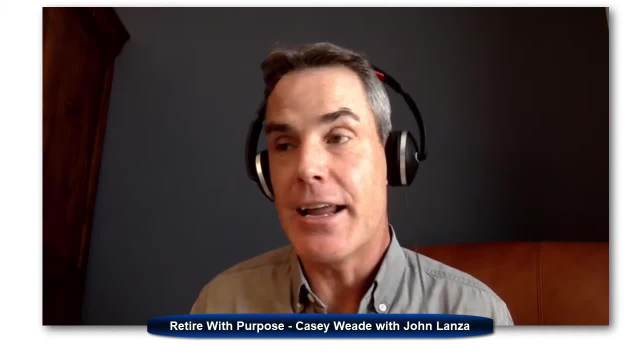 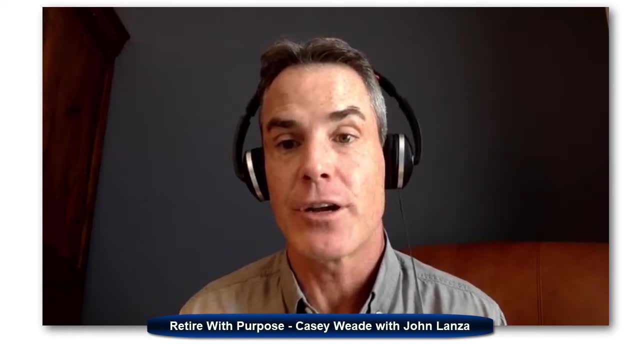 job and taking a loan from us and i- and having having had that conversation with bill, i feel much more comfortable about the idea that it's a good idea. it's a good idea for a kid- they end up getting their, their wages garnished. yes, you know in a sense right. so now they get a feeling for. 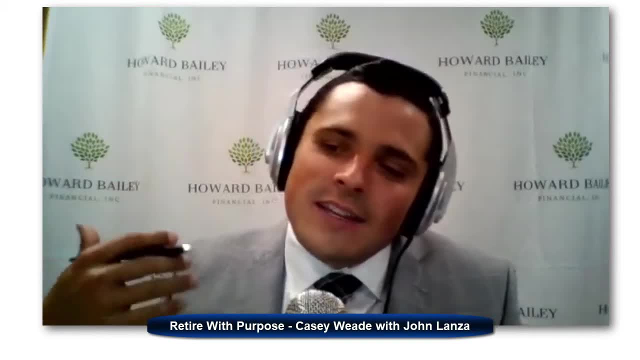 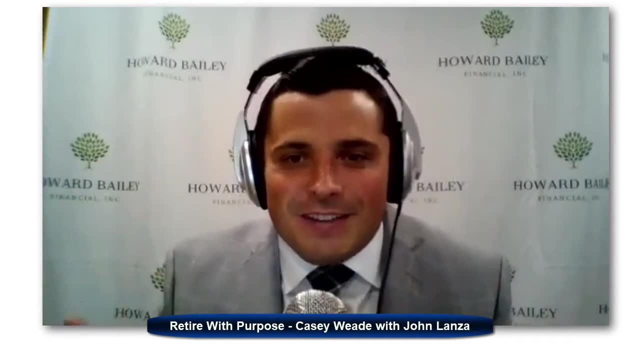 what it's like to have a mortgage payment or what it's like to have a loan, and- and you didn't put them at risk, you know to damage their financial future by making a mistake. you said you know. now, if you make a mistake, at least you know it's. you're tiptoeing into this, you don't have to worry. 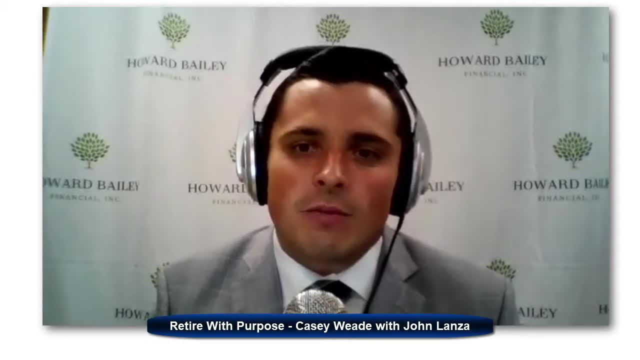 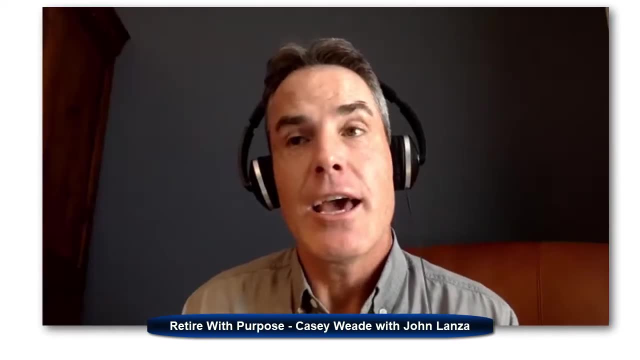 about you know them affecting their, their credit or or really running into an issue because you still are there to catch them, especially if they're, you know, 13, 14 years old. that's okay, right and and you're, and it's a low stakes environment. i know some parents will listen. 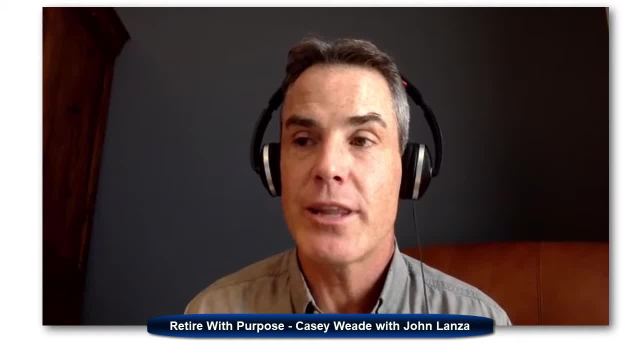 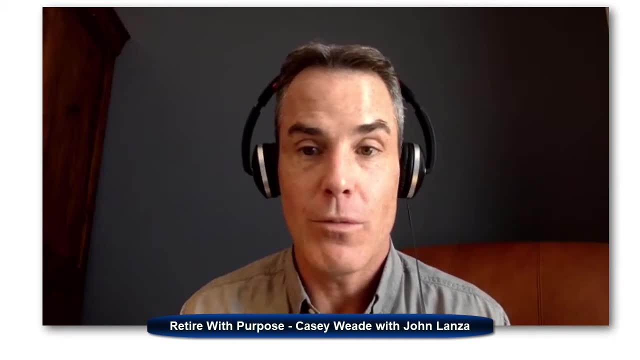 to this and say, wow, that sounds pretty harsh loan for your kid. why are you doing that? but and the reason that it makes sense is that they're going to eventually have to deal with a loan, almost almost definitely, inevitably, inevitably, it's going to happen. so why not give them the experience of having gone through the process. yeah, sure, they're paying you back and- and you're a parent, it's apparent it's your prerogative also to relieve them some debt. you could do that if they, if they've been, if they've, if you feel like they've learned the lesson and they've paid off. 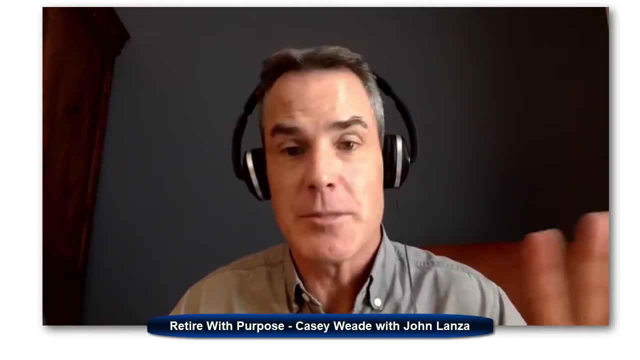 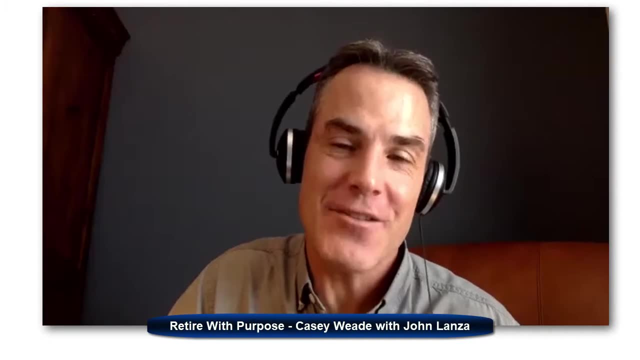 the loan and you feel like, okay, this is, this is becoming. the lesson's been learned. that's perfectly fine. chapter 11: yeah, but it's the lowest. it's the fact that it's low stakes, like you had said it's. this is a chance for them. they're not going to. you're not going. 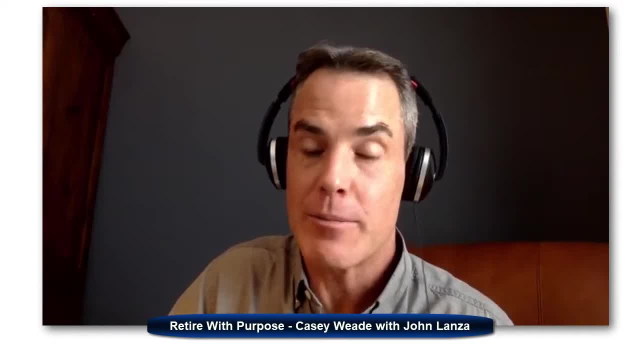 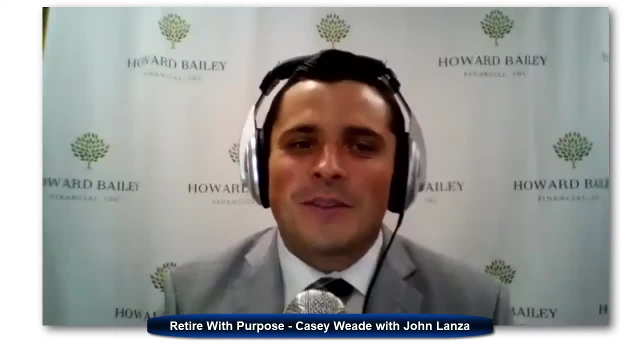 to impact their financial future at all, except most likely positively, because then they'll have some experience with something that's it's going to come up. this is going to come up, absolutely so. so, john right, we're wrapping up here. i wanted to ask you a couple of stock questions, if i could. 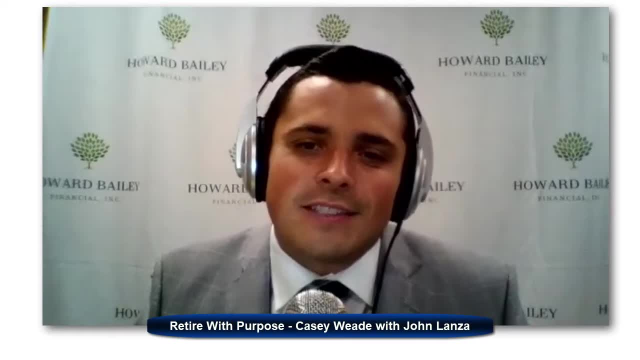 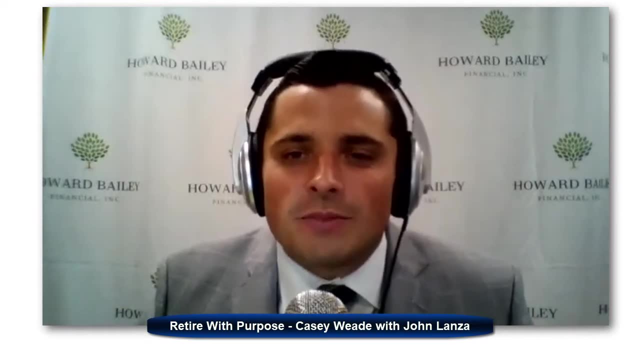 my first one. i think this will be interesting. uh, since your focus is on younger individuals, if you could revisit your 20 year old life, and if you could revisit your 20 year old life and self, what advice would you offer? i should have the stock answer to that one, because i've asked people. 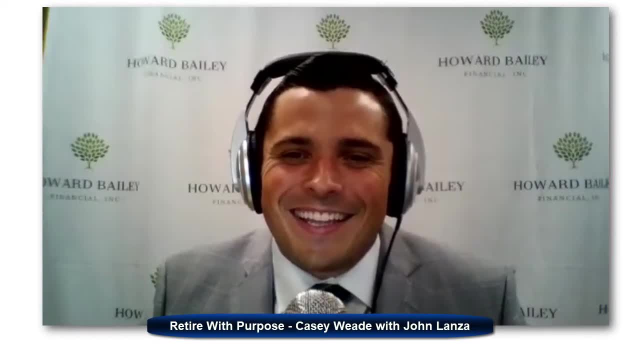 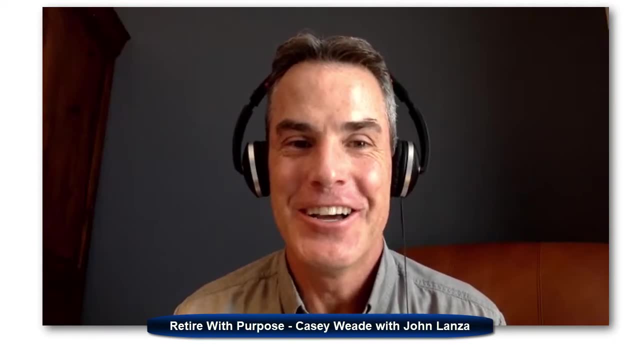 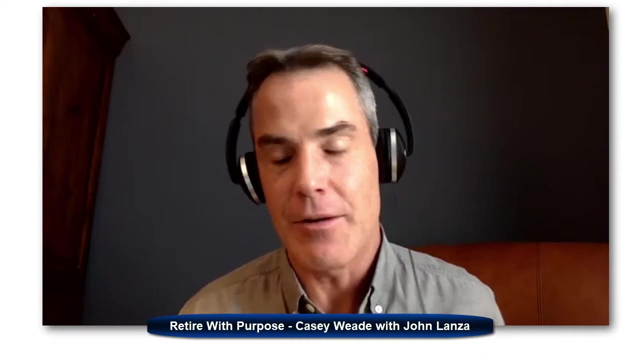 uh, the advice would have to be: um, buy, buy real estate today. you know it would be: either buy real estate today or sock money away and use that power of compound interest, and they're both basically the same thing, that is. that was one of the things my dad 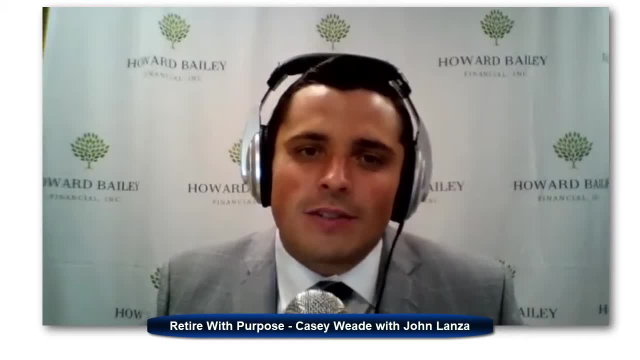 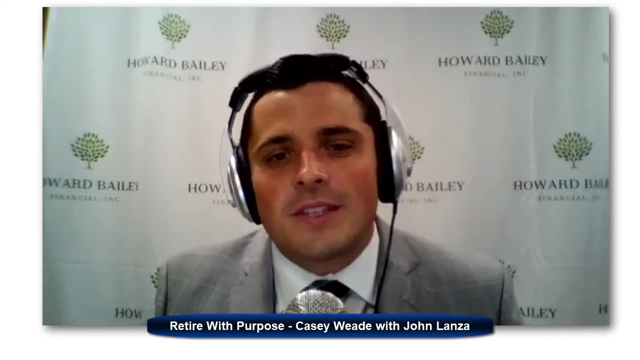 always said he made- uh, you know he was a financial advisor- uh, however, he made the majority of his wealth and real estate. and he always said, even- and this was something very unorthodox, very controversial- he would say, uh, but he would recommend, you know, young families. uh, if they're. 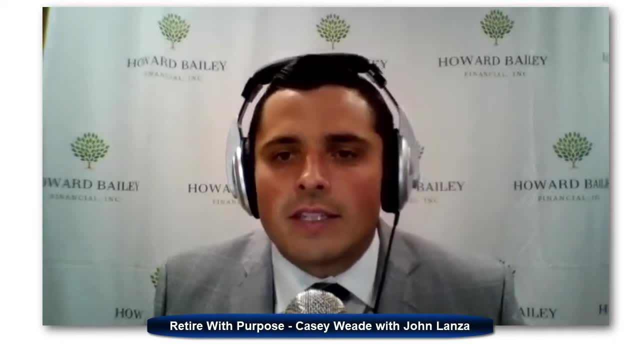 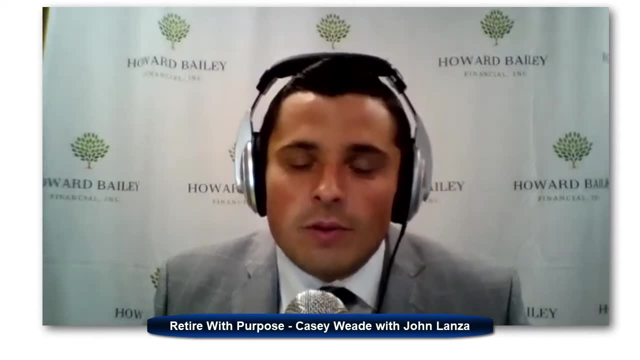 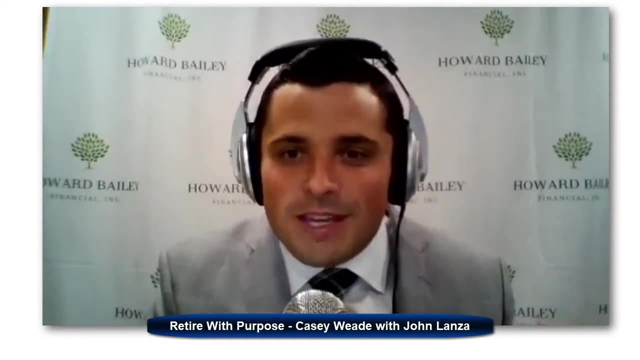 in a, you know, financially stable position and they had some excess income, go buy a lake cottage. and that puts you in a position where you are forced- it's forced- savings. maybe it doesn't, maybe it doesn't make 10, 15. percent a year, maybe it doesn't perform as well as the market, but now you're forced to make that. 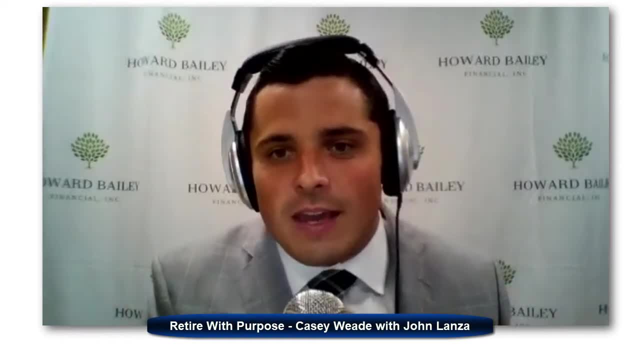 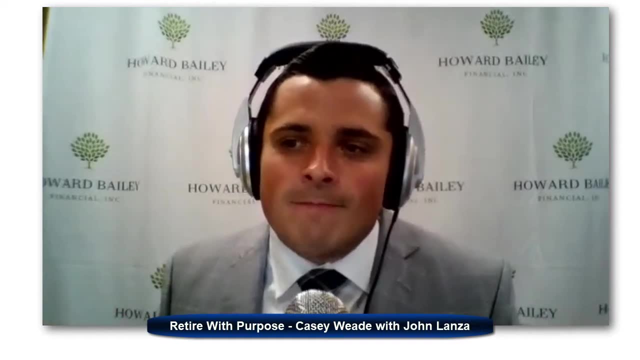 mortgage payment every single month to pay off that place that you have on the water and it's hopefully appreciating over time, whereas you put those dollars into your 401k. you might say: you know what i really want to buy that sports car. this year i'm going to cut back my 401k contributions. 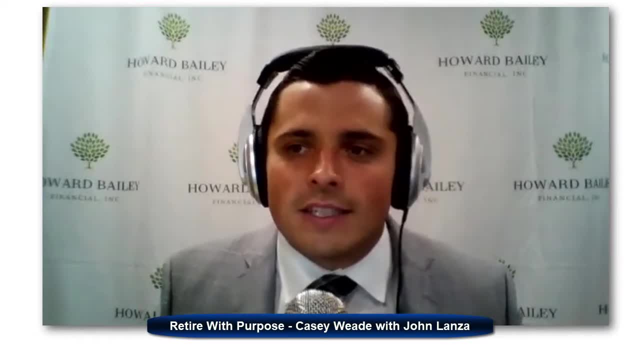 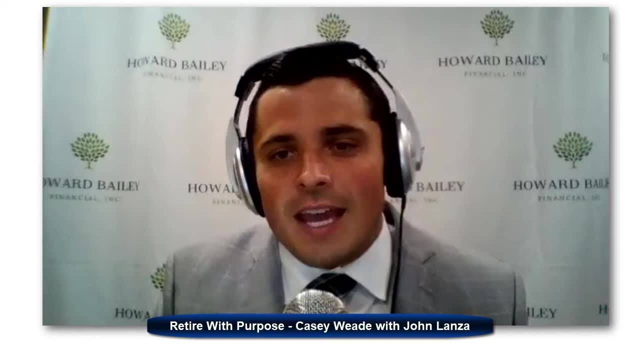 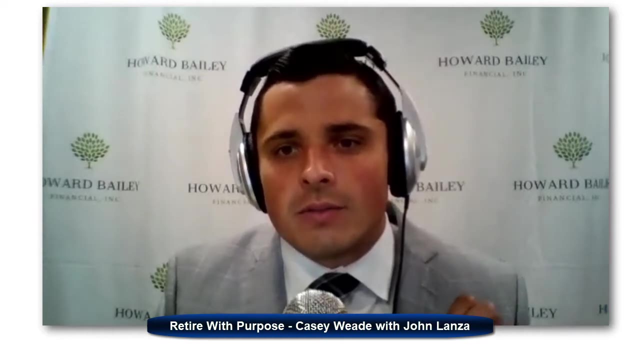 a little bit. uh, real estate's definitely one of the ways that i see and they say: and the majority of millionaires have been created due to real estate investments, and so there's absolutely something to be said about real estate. maybe it's not the performance of real estate, maybe it's just the obligation that it creates in your life. yeah, that's one of. 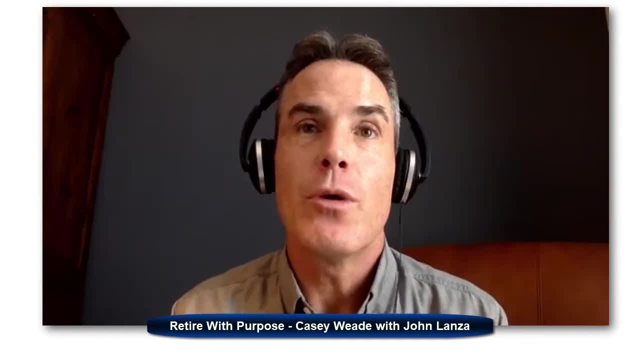 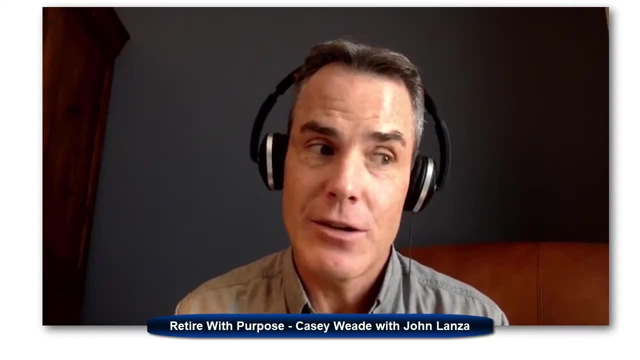 the things we told our kids we hope we hope they'll do, which is to when they go to college and we'll see if they end up doing it. but you know it's like live in the dorms for two years and then you know we'll. we would love to help you, you know, buy a place that you live in and 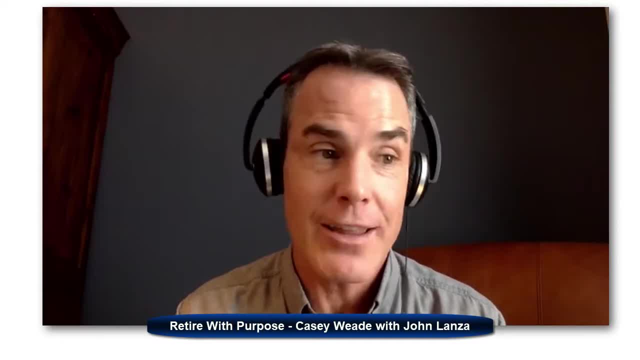 rent it out, because then you can you know you you can find the kids you know they'll be friends of yours that would be living there, and then you're kind of starting them on the on that right path. so i've seen families do that and have a lot. 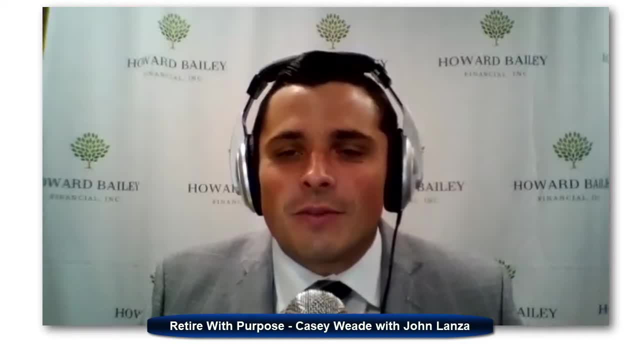 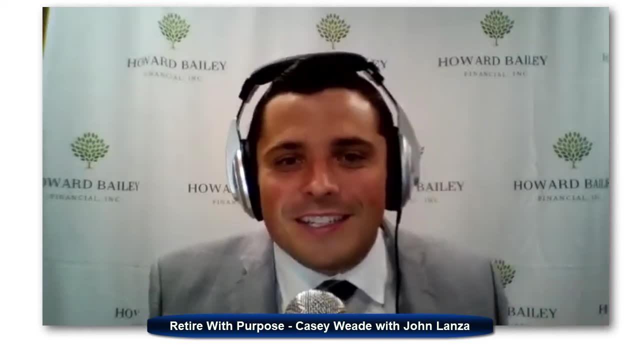 of luck with, uh, their, their kids kind of get the feeling for what it's like to be a landlord and they can decide if they want to do that or not the rest of their lives. but at least they're starting collect those rent payments and it's it's pretty neat that that passive income. yeah, my next question. 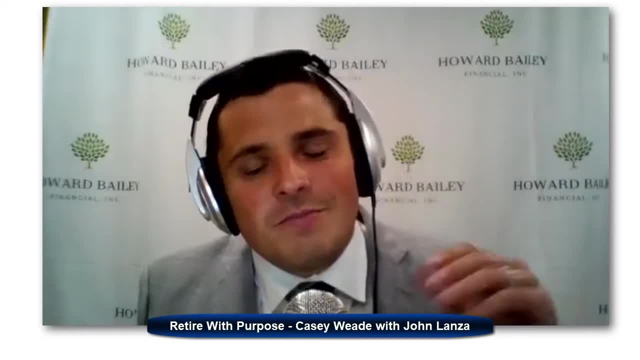 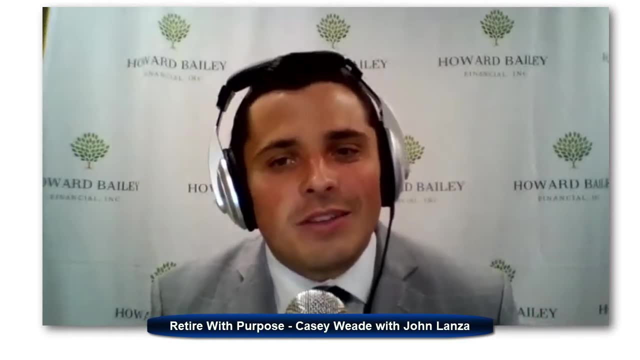 is if there was one question. i assume you've. i mean, i know, you know from new york times to, uh, you know, the wall street journal. you've been interviewed quite a few times and you've been asked a lot of different questions. if there was one question, 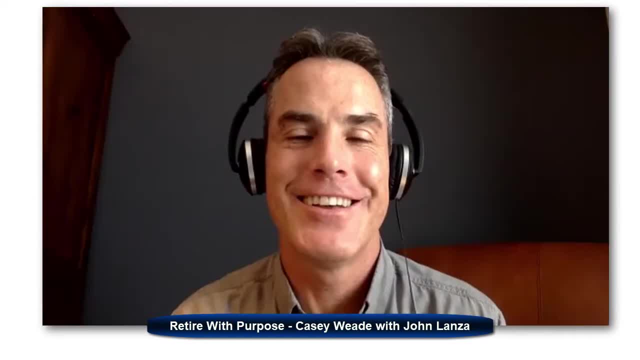 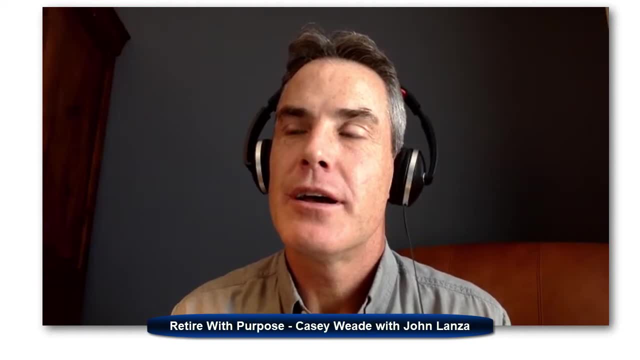 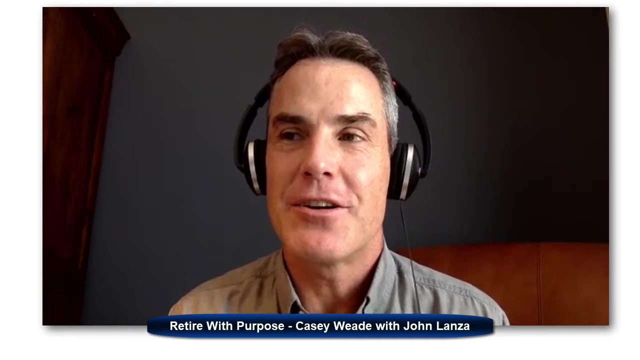 you could never be asked again. what would it be? wow, um, that is a good question. one question, i guess, one. i guess the question that i that and this. doesn't come up that much, but there are times where people will give you the snarky comments like, well, why would i? that doesn't sound very money. smart to. 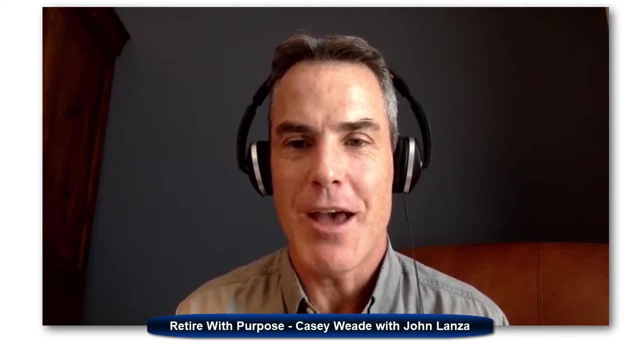 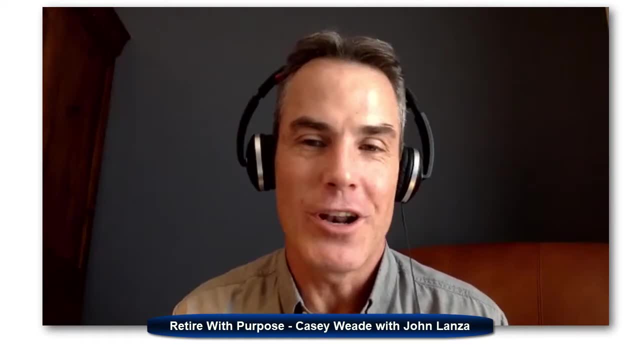 you know, get one of these things that you're talking about, whether it's the money mammals, the art of allowance, i'm gonna be money smart and i'm not gonna spend my money on that, said you don't, so so i guess that would be the one question i could think of: be money smart and 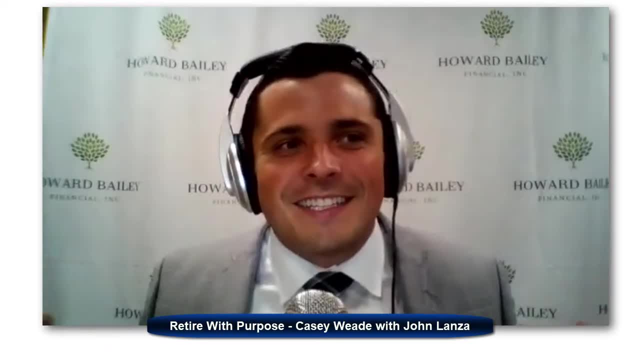 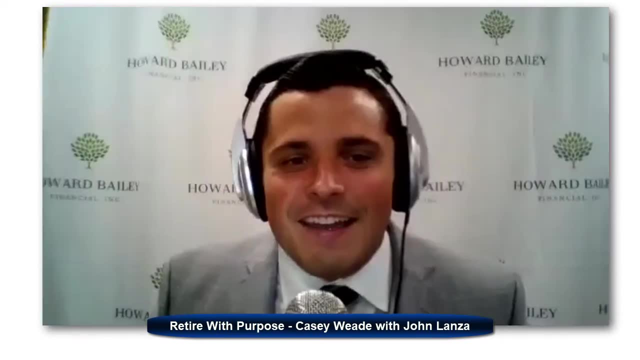 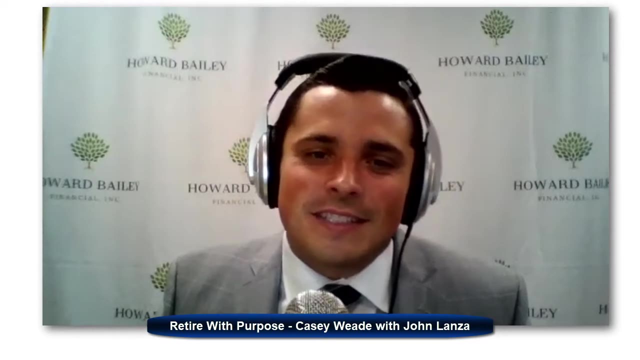 not spend my money on the money mammals. i gotta say the, the cartoons. my kid loves them. we've been watching those on repeat at our house and and i mean, and they, both of them there are two-year-old and our one-year-old the tv, and i, well, you know, this is, this is uh, this is a lot better. 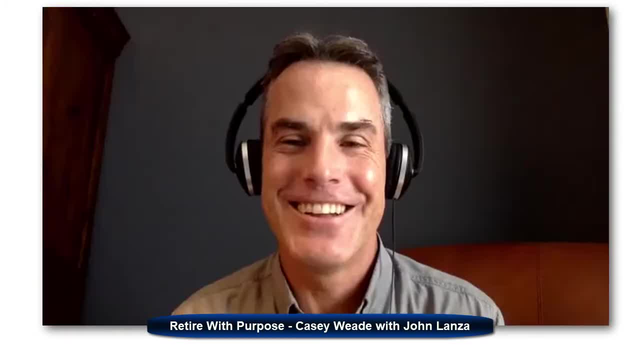 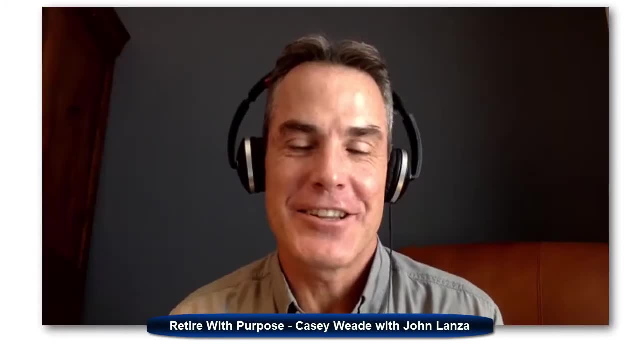 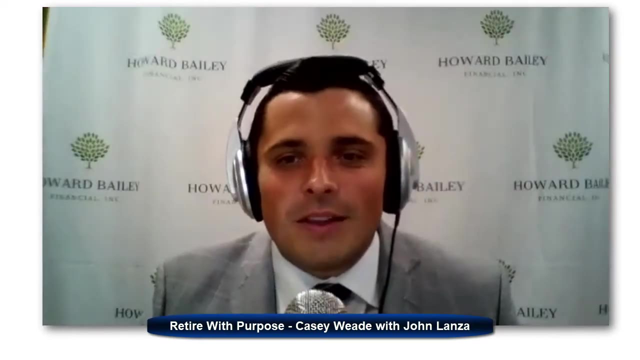 than you know, uh, transformers or something. at least it's educational and the kids enjoy it at the same time. so right and it's, you know they're. they're not like, they're not expensive and they're there to just teach kids about money. i know, i don't even remember how i bought the the family. 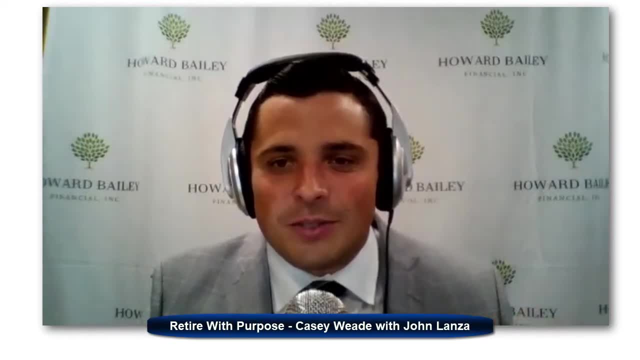 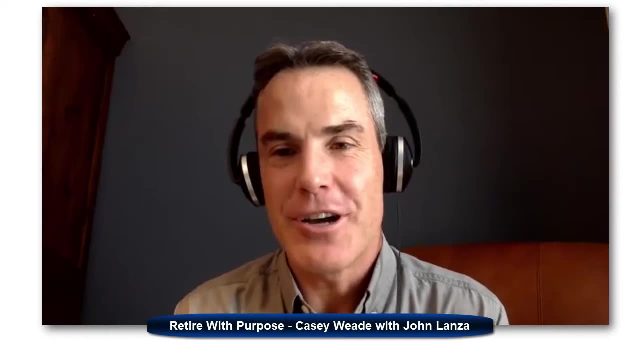 kit that had, right, the dvd, the book and the children's books in it. i don't know, i don't know even remember how much that was to you. uh, it's, it's. uh, oh, i should not, i think camera, is that the third? i was gonna say it was something like 14 or 15 dollars, i don't know that it was, you know. 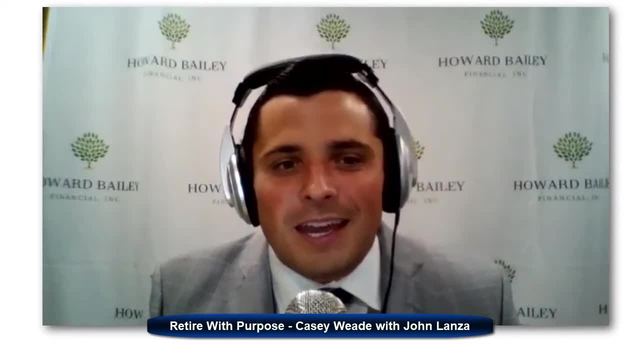 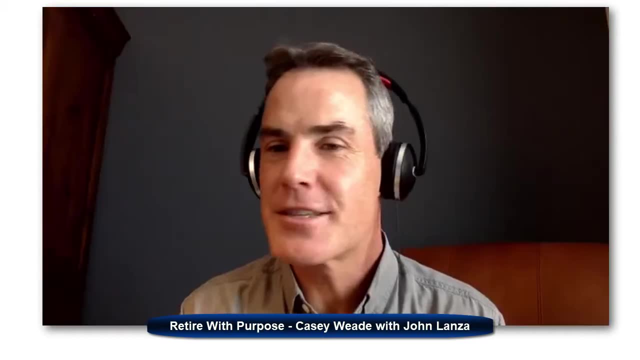 it wasn't breaking the bank and i'm sure it's going to pay back. you know, probably a thousand fold, you know. if not, it's not substantially more than that over the lifetime. yeah, it's less than 40 and you know you're getting your, if nothing else. like we started talking about the beginning, 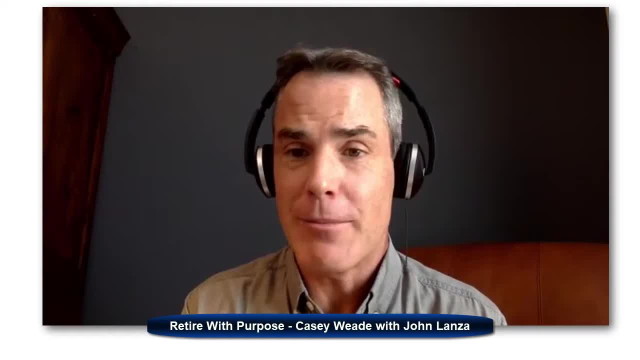 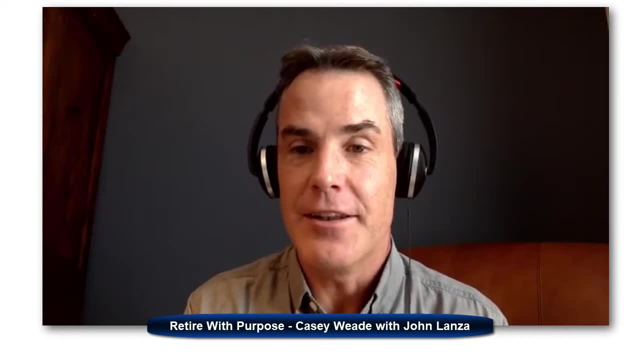 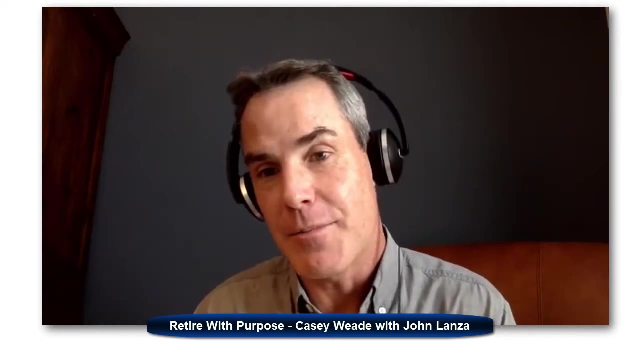 and, and you don't need, uh, you know the money, mammals, the art of allowance, to do this. it's the starting of a conversation, is really that's such the key. and, um, you know that's and, and and that's, that's just providing a framework. is what those things do? getting the kids excited and then providing a framework for 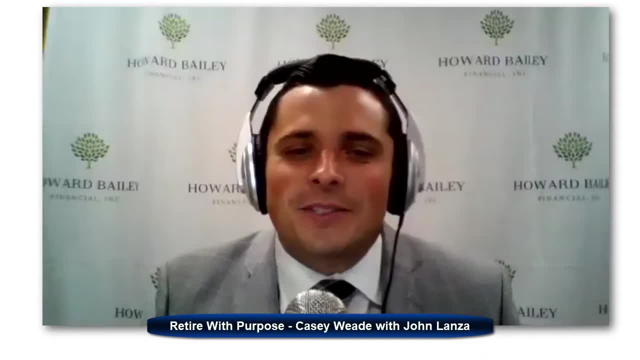 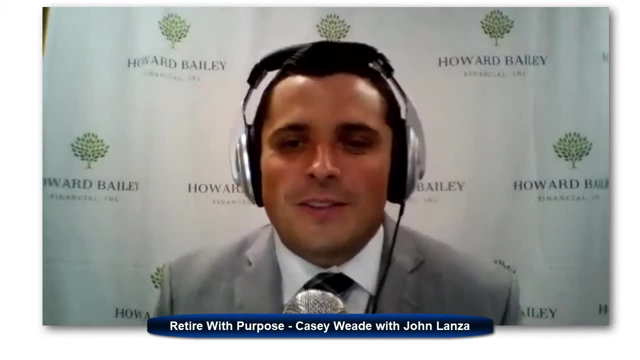 the parents is the whole purpose behind it. so my last question, john, and this question. i've asked thousands of people, uh, whether it's on radio, tv podcasts or in person or in a live audience, and i am surprised that you're doing this, and i'm surprised that you're doing this and i'm surprised. 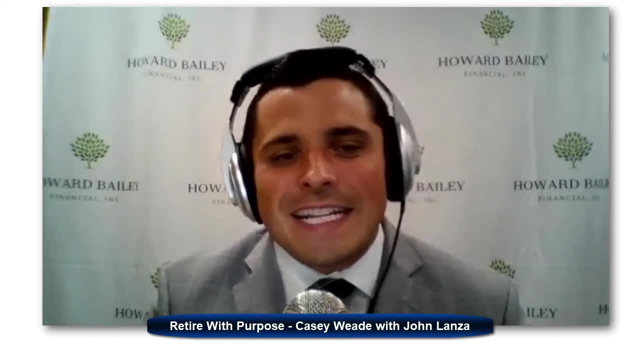 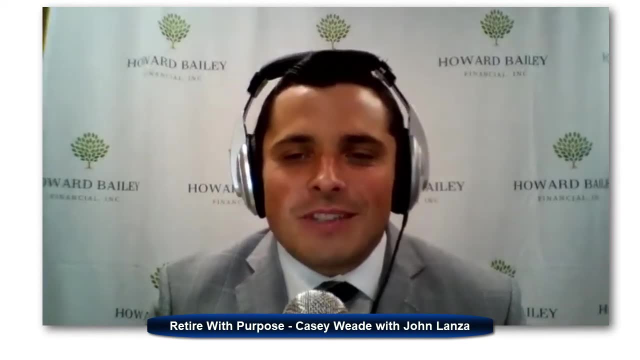 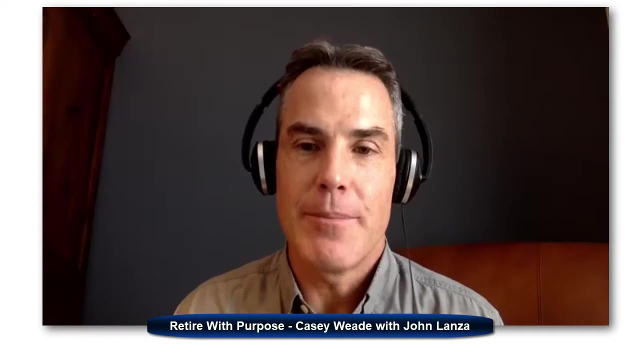 the wide uh breadth of uh answers that i get here, uh, yeah, and now, and i don't know how far you are from retirement, however, uh, my question would be: what does retirement mean to you in one word? if you could use one word, what would that word be? uh, financial independence, that's. that's what. 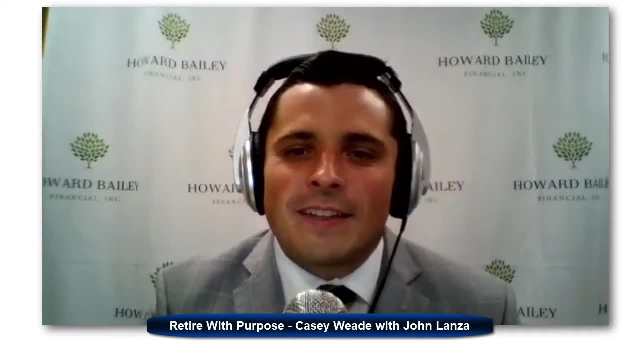 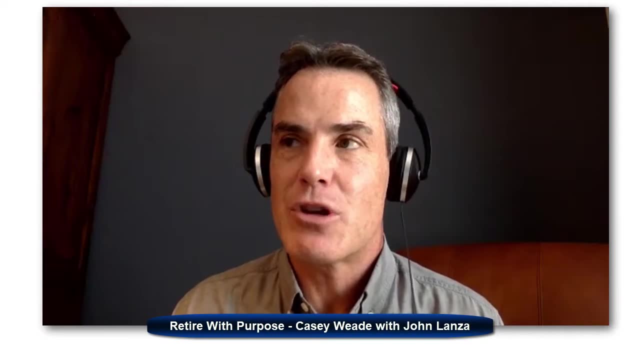 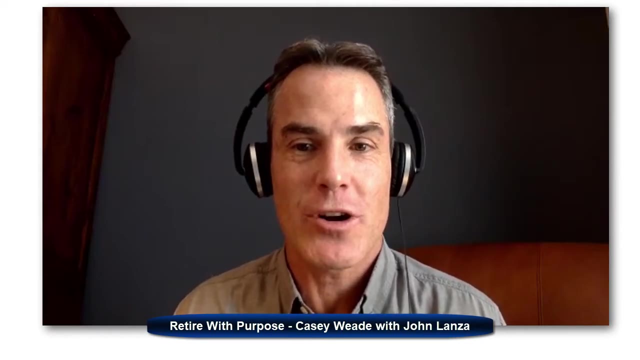 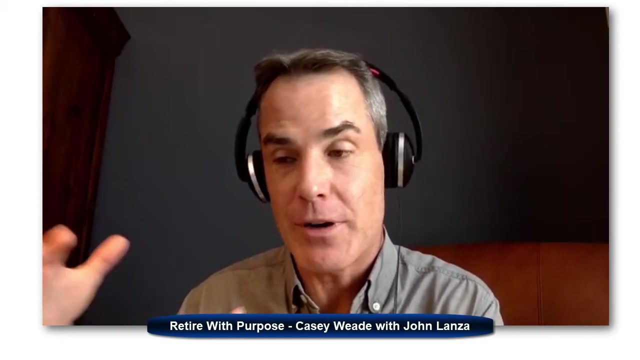 retirement means independence. yeah, independence, yeah, because- and i think financial independence is the key, because i don't have any desire to retire- my dad retired and he's working more now than he did. i think what he was working? because he he was a banker and now he wrote a book. uh, that was about his uncle's ex. what his 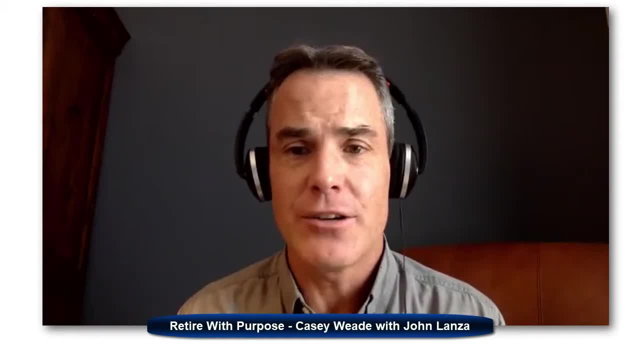 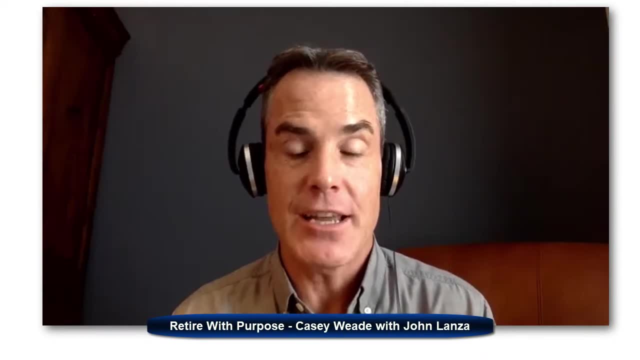 uncle went through in world war ii and he does talks and all that and he's really found meaning in doing that. so that's what i mean. that's that's really kind of where the meaning comes in- is that you just want that financial, financial independence to do what is kind of your life's purpose. 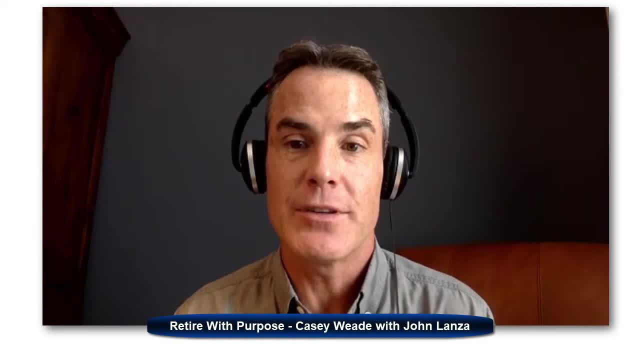 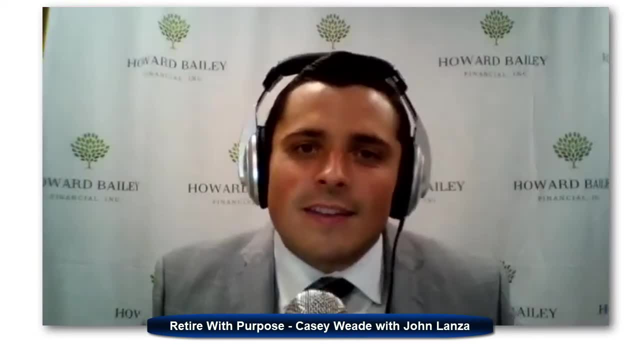 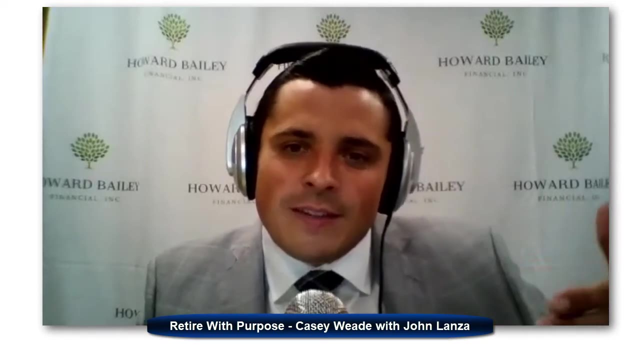 and i feel like i'm doing what is my life's purpose, and so that the retirement is less important than the financial independence. do you feel- and you know we can cut this out later if you want, but do you feel like you've- are you at that point in life where you have reached financial? 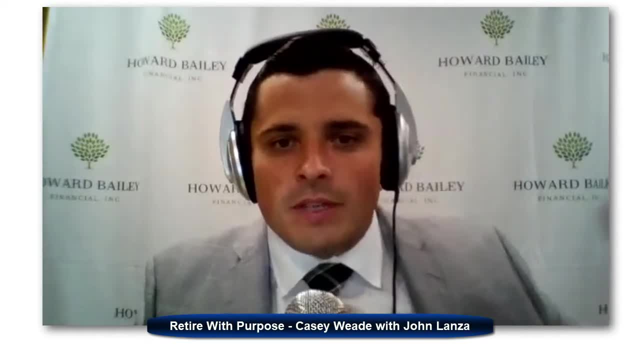 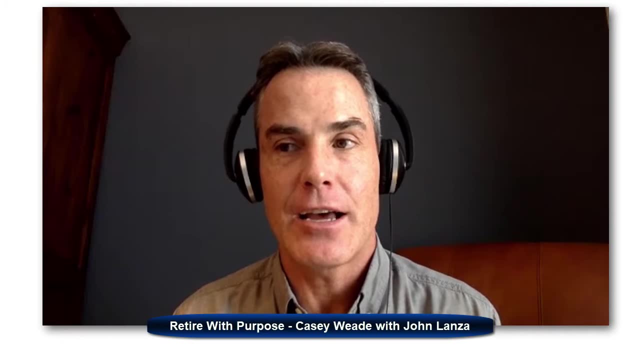 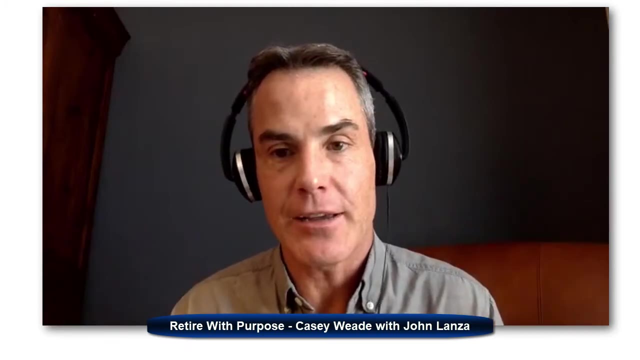 independence and you're living- uh, you're living- your purpose-based retirement. no, we're working towards financial independence, um, but the nice part is that i- i feel like i get to the like i said. i'm working on something that i feel like is the purpose, like if i, if i, if i had all the 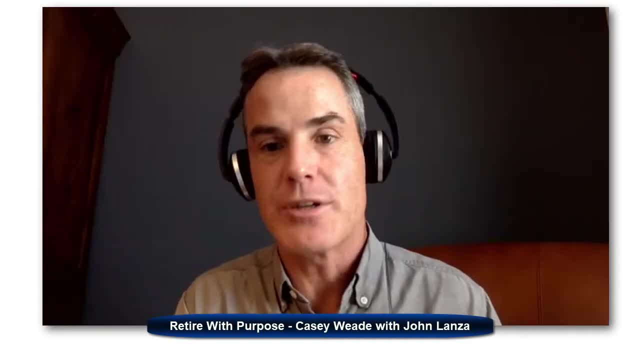 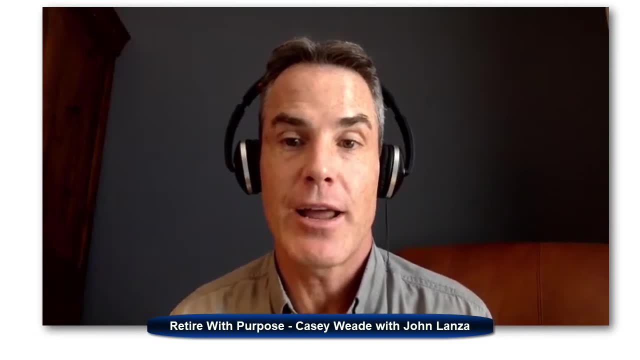 money in the world tomorrow, and, and, and, and could retire tomorrow. i don't think i would do. i really don't think i would do it much, uh, anything much different than what i'm doing right now. well, so so when you get there, what's going to change? when you get to the point where i have enough? 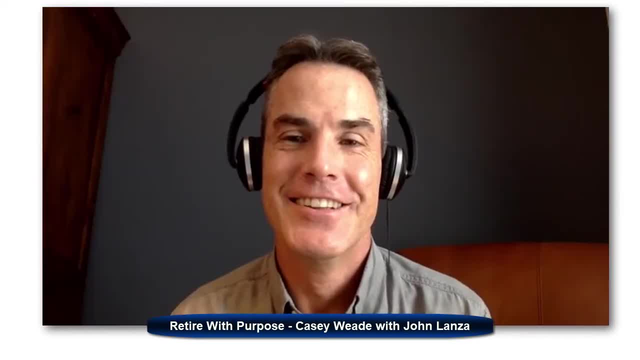 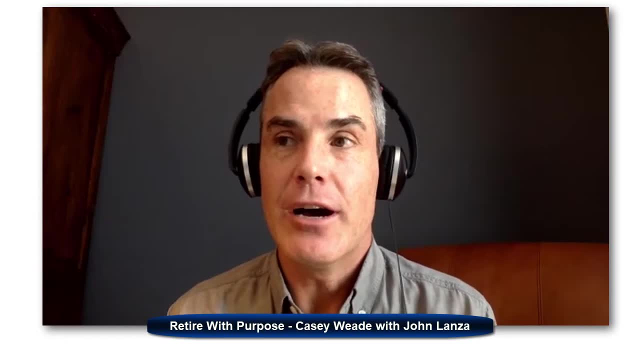 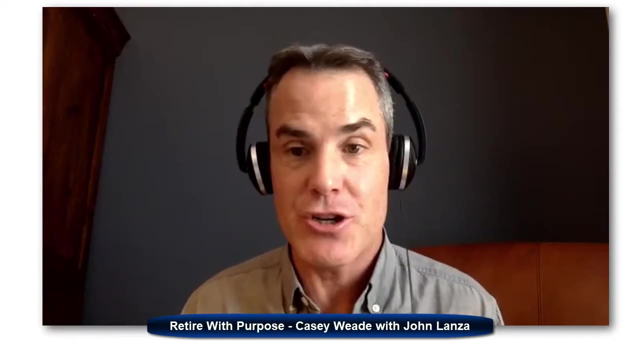 i could quit working tomorrow. how will you treat your life differently? um, it's not going to be markedly different, um, because you know, i've, i, i- one of the things i've done- and i talk about it in the book too- is just in the i. i've gotten as much out of teaching. 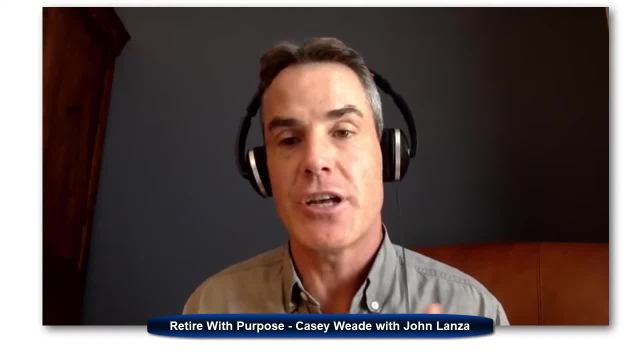 my kids and i think they've gotten, because there's just so much self-reflection. that happens when you start really engaging with this concept and this discussion of money, when you start talking about your kids, you naturally have to kind of reflect on your own attitudes toward money, and one of the 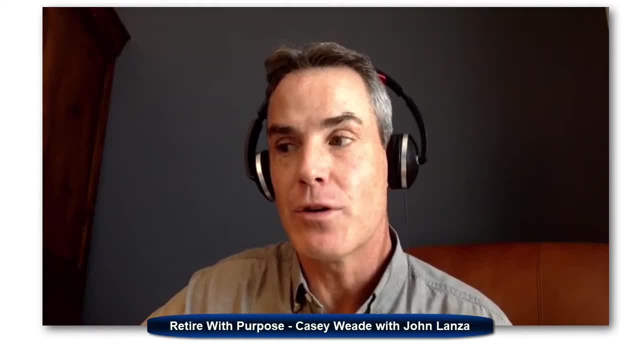 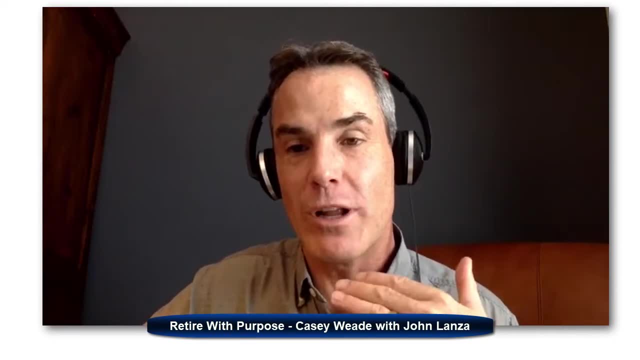 things that i've done is i've done a lot of self-reflection and i've done a lot of self-reflection. i've done a lot of is i've, i've, i've really cut back on. you know, i have kind of a minimalist wardrobe, i, i live a relatively minimalist life and uh, and i like that i, i could and i, you know. 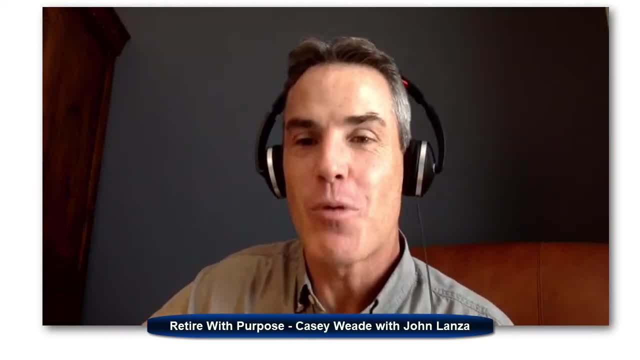 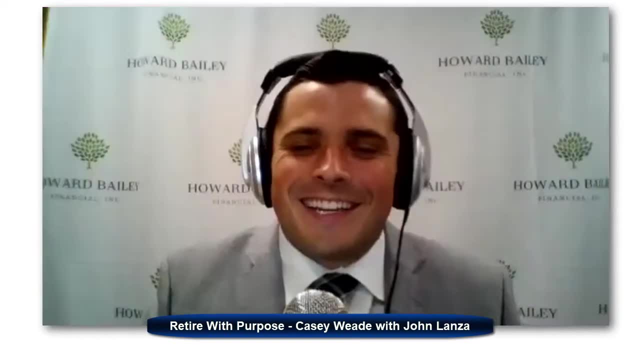 it's, it's, it's, um, it's. it's an interesting point of conversation with my wife and i because you know i went through that period. i was looking at at tiny houses. she said we're not moving into, i'm not, i don't really want to live in a tiny house, but there is. 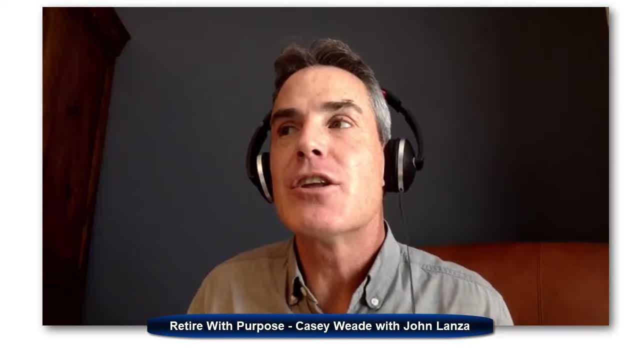 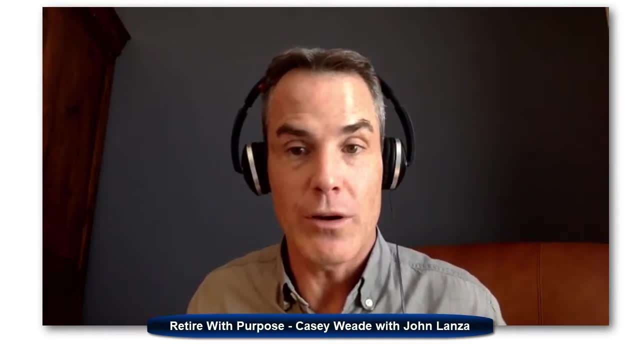 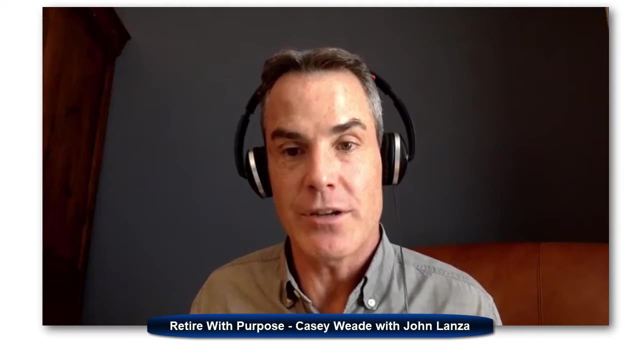 my interest was piqued in the sense that it's the the idea behind it is is very much the idea behind what- the art of allowance as well, and what we're doing and what we've been talking about here, which is that things are not what define us. meaning is really ultimately what defines us, and it goes back. 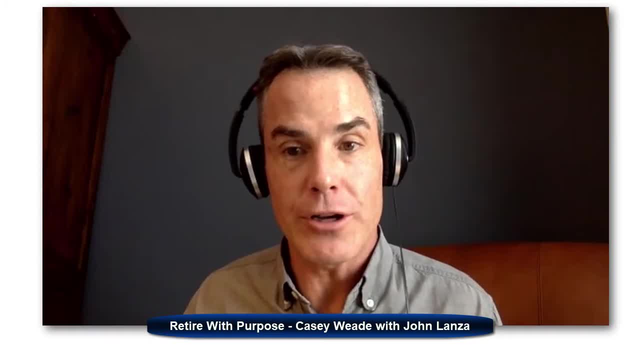 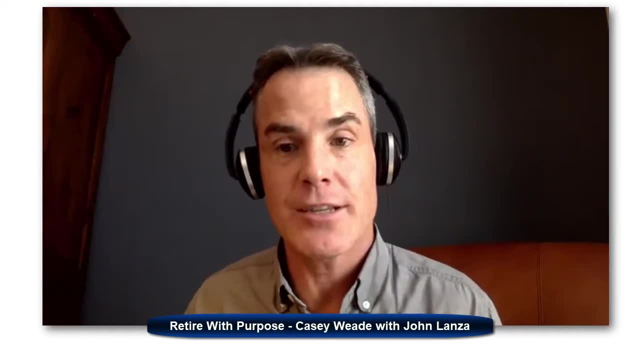 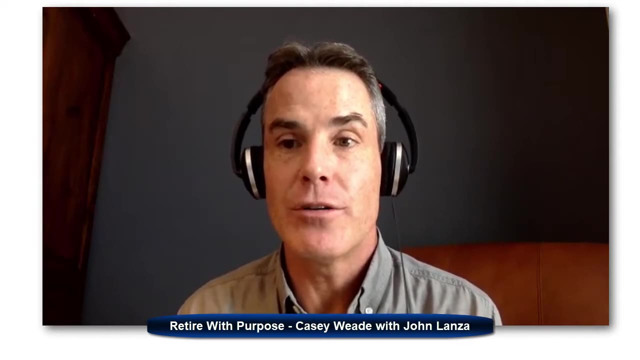 to this kind of philosophical question that you posed earlier, which is kind of: you know why, you know what, what you know. how have we lost, how have so many of us lost touch with that, and what can we do to get ourselves back in touch with that? and that's in part what i wanted to try. 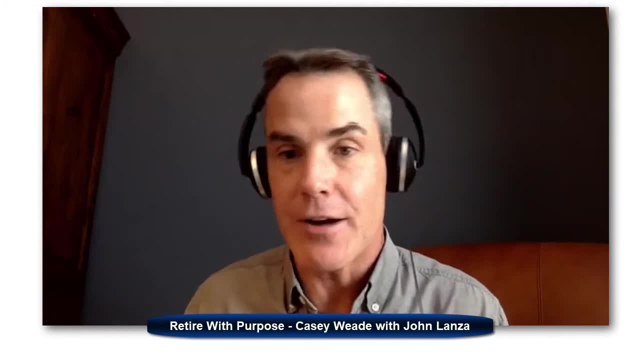 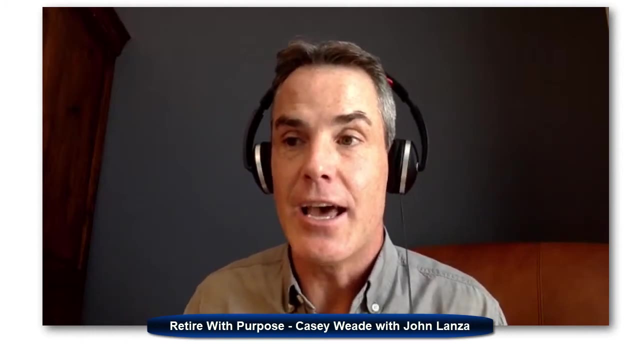 to accomplish. in the book is. you know, there we talk about the kind of framework but we also talk about in those little asides kind of what money is what, how money it, how money affects us, kind of affects our attitudes, what our attitude toward money is and our attitude towards stuff and 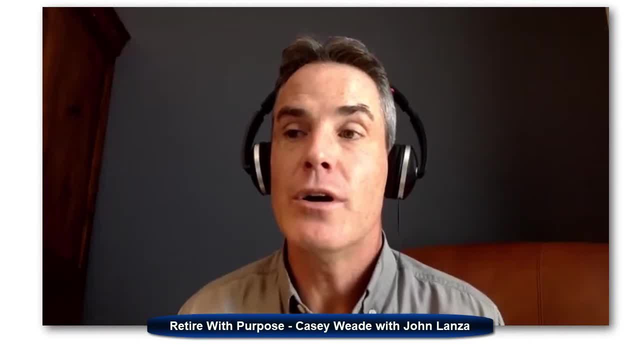 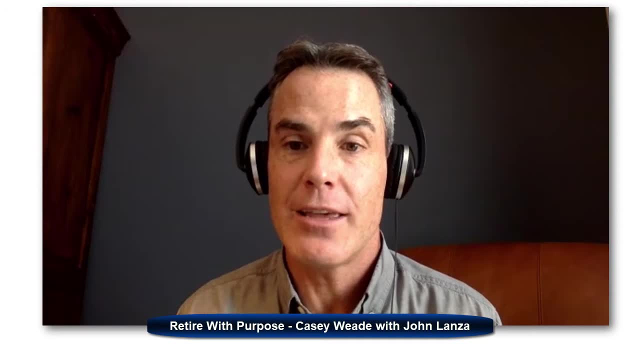 things and products and all of that, and how we're going to be able to do that and i think that's a really good point and how we really need it's. it's a good idea to just take stock of where what we're doing with our money and how we can kind of use it most effectively to increase our own kind of 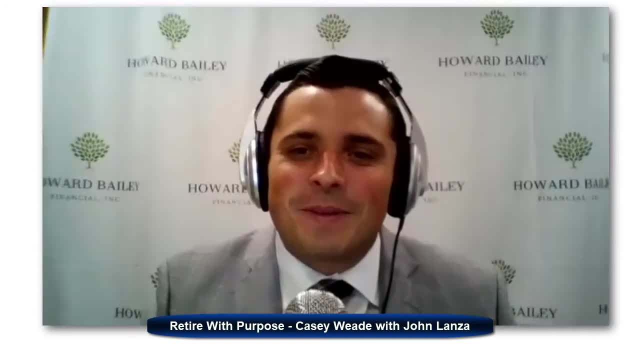 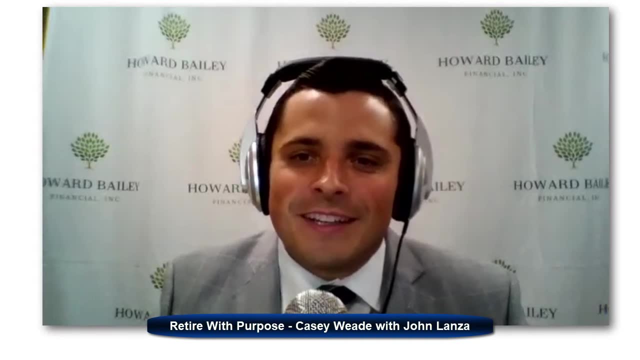 fulfillment and happiness. well, john, it's been great to be able to have the opportunity to interview you and and talk a little bit about these topics that, for me, raising children are just. you know, we're just at the cusp of figuring this stuff out and it couldn't have been better. 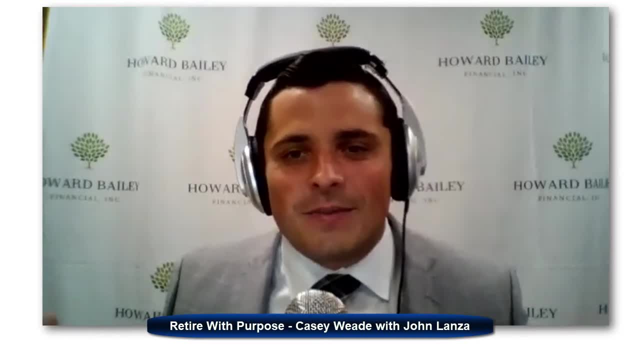 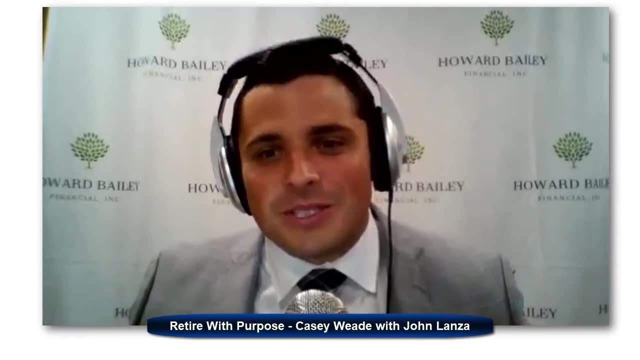 timed. all of our friends are beginning to have children, and so now you know, people always want to ask that question. it seems like on every podcast: what is the book that you'd be giving out? what's your most gift booked? and, and i've got to say i 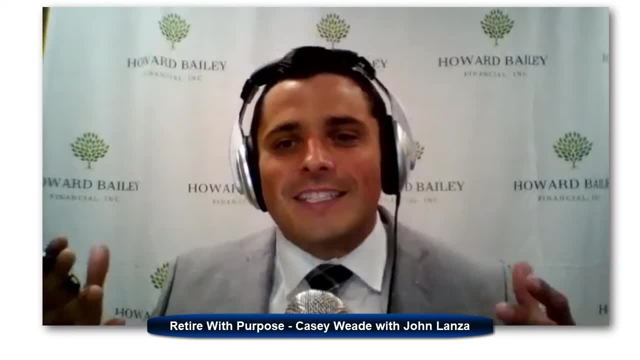 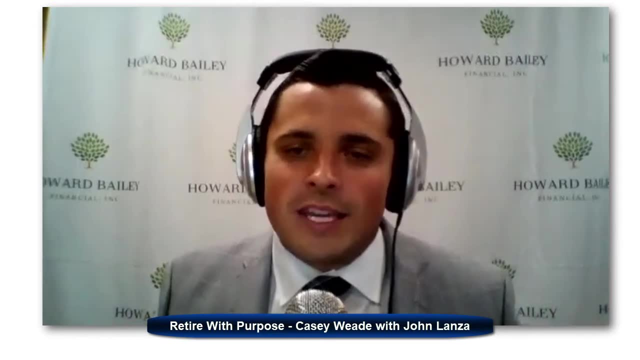 think there's a good chance this will become my most gift book, at least in at this point in my life. i've just got so many friends that could benefit from this information. you know i i live it every day being in finance, being a certified financial planner, running an independent financial. 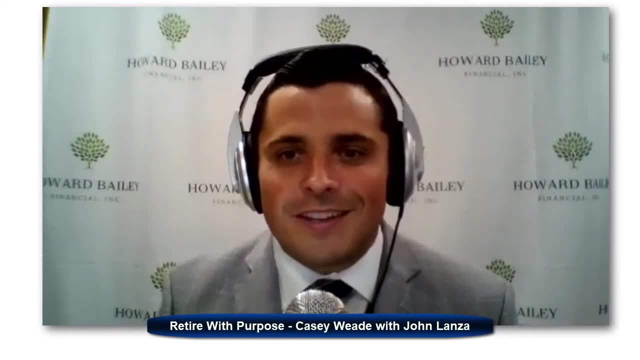 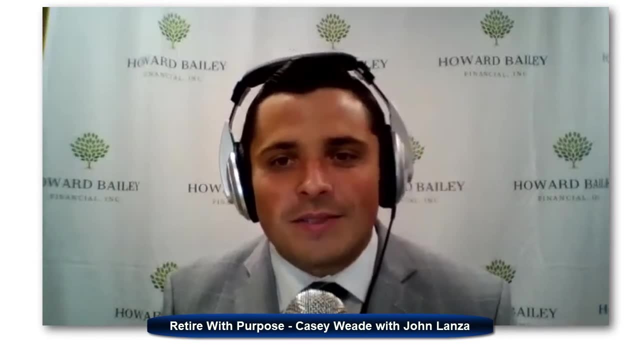 planning practice. you know it. just, it's common sense to me. that's what i, that's what i think about. however, you know, my friends are we're living and working completely different lives and it's not at the top of their mind. even our, our- uh, you know our- godparents. you know we're going to have to. 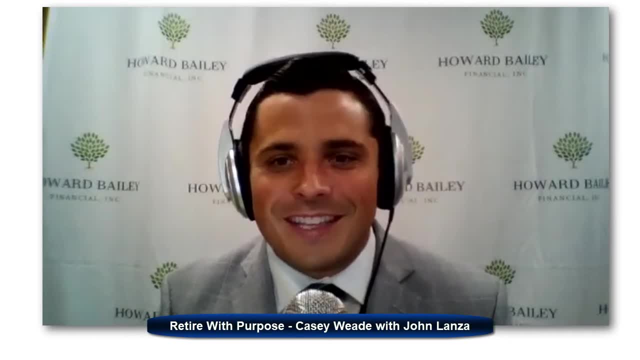 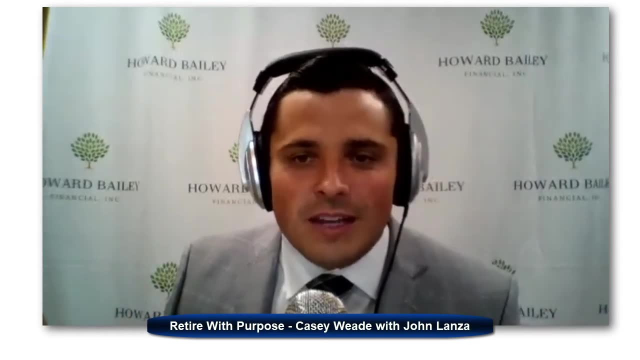 get them on the train so they know what they're in for if anything ever happens to us. so thank you again for for really just giving putting this in my life and all of our friends lives. uh, you know, we're going to have the opportunity. we're going to give out a few books to, uh, everyone that visits.